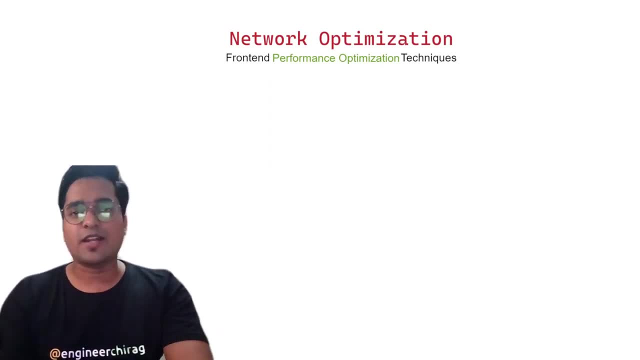 techniques. So what we are going to cover in this particular episode, let's, let's quickly talk about that. The first one which we are going to talk about in the network optimization. Okay, let me reset. Okay, In network optimization, the things we are going to talk is: first: one is the lazy. 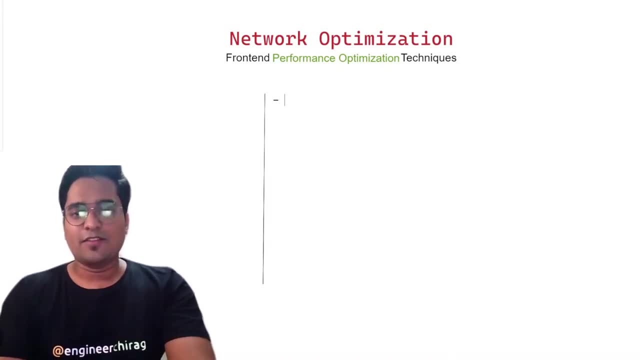 loading. Okay, so first one. first, we will be covering lazy loading. What else? We will be also talking about JS in async fashion, loading JavaScript, JavaScript in async fashion. What else? We will be talking about content visibility, which is very important and cool technique we will be covering. 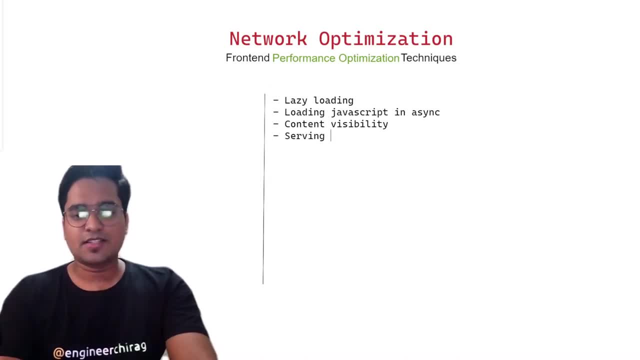 What else? We will be talking about serving critical CSS and the techniques to do that. We will be going to cover those things. What is that? So hold on with me. we are going to cover that. we are going to cover the caching layers as well. So caching using service worker. If you haven't heard about. 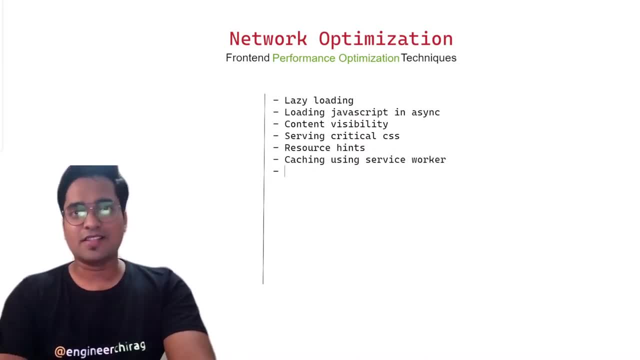 these techniques. don't worry, we are going to cover in depth What else we will be covering: caching using CDN And what are the headers. basically, that is going to help you to make it more beneficial. We are going to cover the client side rendering. we are going to cover server side. 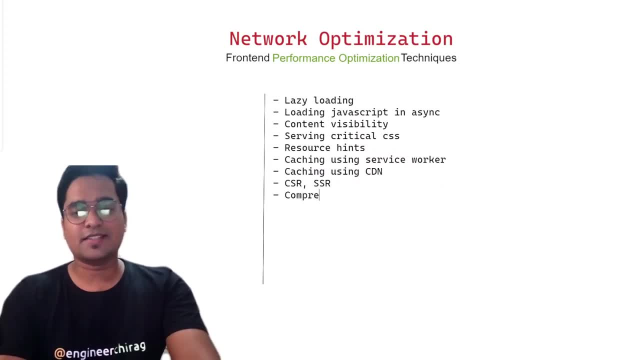 rendering. we are going to cover the compression techniques, So we are going to cover this as well. Okay, now what is? we are going to cover things which will help you to basically avoid the, you can say, layout shift and repaint, which is going to 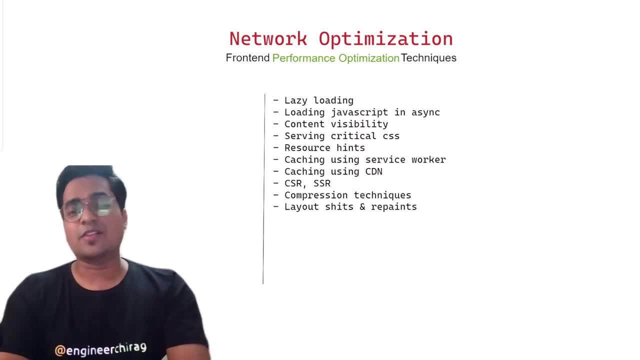 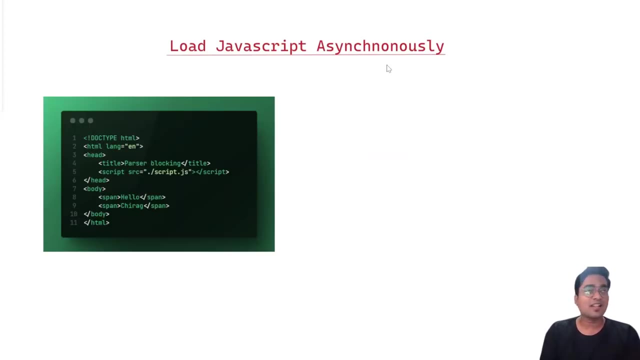 give you a browser or your application a better performance. not limited to that. we have so many extra thing that we are going to cover, So keep watching till the end, and so many exciting things are waiting for you. First thing first. our JavaScript are synchronously so that we can actually leverage the network layer right. So we 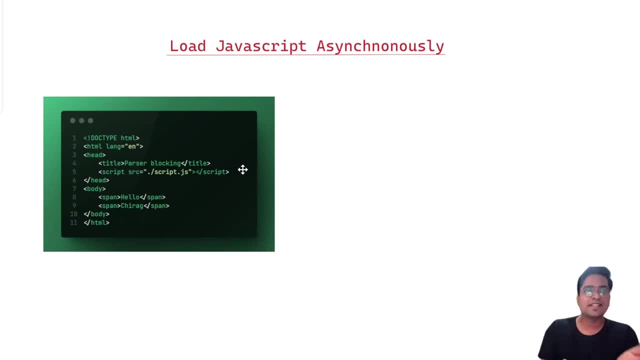 have a lot of limitation. we'll be talking about those limitation in terms of downloading the asset, how to download, when to download, but taking this example, basic HTML, where we have in the head we have a script and in body we have simple text to be rendered. So how generally browser? 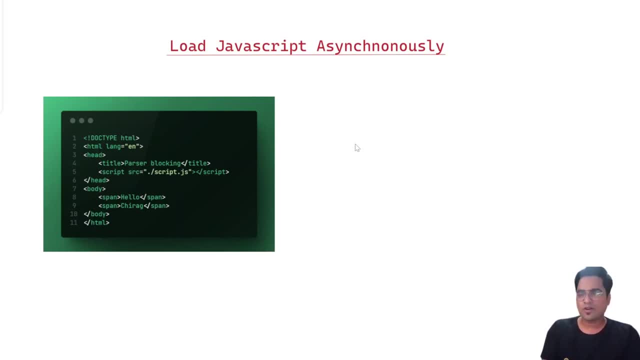 basically renders this and how basically downloads the asset. we will be talking in detail, But let's see some glimpses of that, Okay, So in this particular case, when it encountered the script, what it is going to do, it was parsing, parsing, parsing, parsing. it see, Oh, there is a script tag. 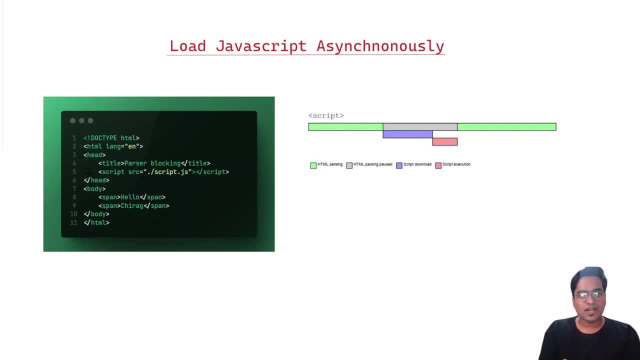 okay, let me do something. What is that something? it encountered a script tag over here. it started downloading it. So once it is downloaded, until it is downloaded, your parsing is stopped. So browser basically won't go into the parsing of the text which is B. you can be that. So once that particular 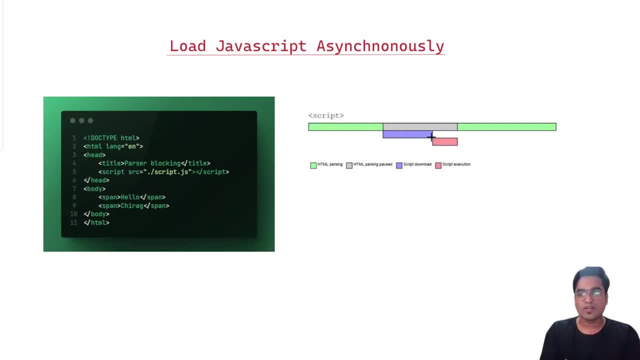 downloading is done. what is going to do next? Is it going to pass again? No, it is going to execute the script first And then, once the script is executed, it is going to pass again. So consider, you have multiple script over here. In that particular case, your browser is going to download the script, execute 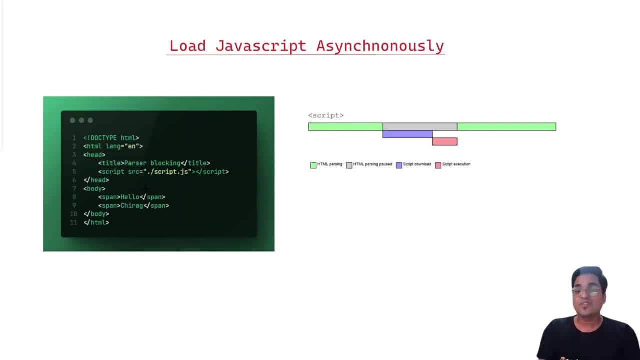 download, execute, download, execute and you won't be able to see anything in the your web page or your browser. basically, until this, your scripts are downloaded and executed. Dude, this is definitely going to hamper because you have a lot of scripts sometimes in your application you have. 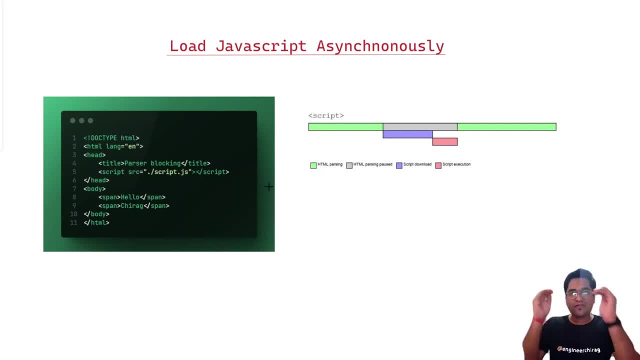 that application, or you have written so many script, right? So you can't wait all the script to be downloaded. Sometimes it's like more than 300 KB or 400 KB, right? If you don't optimize it, it can be in MBs. You can't wait for a couple of minutes or a couple of seconds, basically in order to 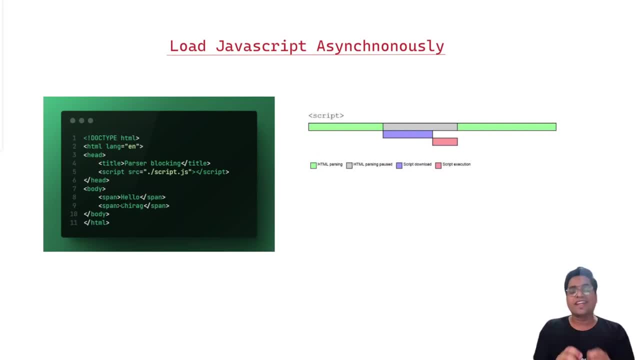 showcase something to the user. This is not going to work. Okay, before we actually dive into and see what are the benefits and what are the different ways, let's try to understand this thing in a very simple way. So consider: you are dress up, you are, you wanted to go and chill out. 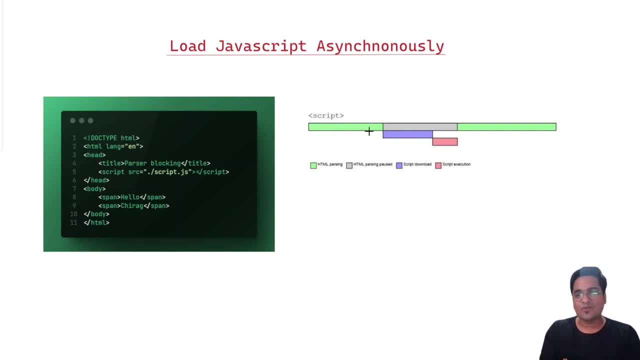 you are going out with your friend, you took a bike and you are basically about to leave your room. You're you're about to leave your house. Suddenly your dad encounter and you found that you are going to leave the house And dad just says, dude, first clean your bike, get the petrol filled. 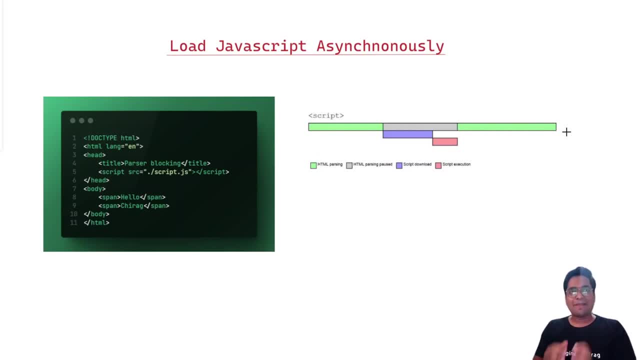 and then only you can go out. Oh shit, My plan is screwed up. I was just about to leave with my friend in order to do a party, But as I was going out, my dad gave a responsibility, which is to clean the bike, get the petrol filled and then basically go out for the party. I'm late. 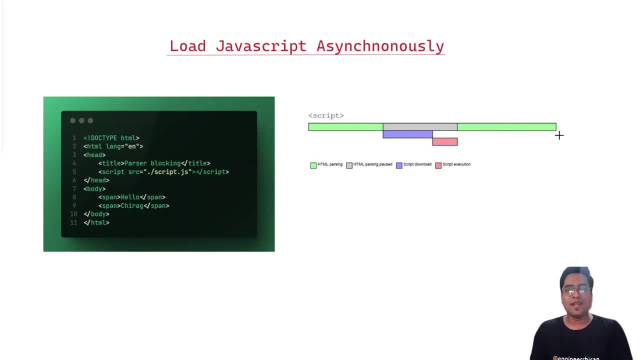 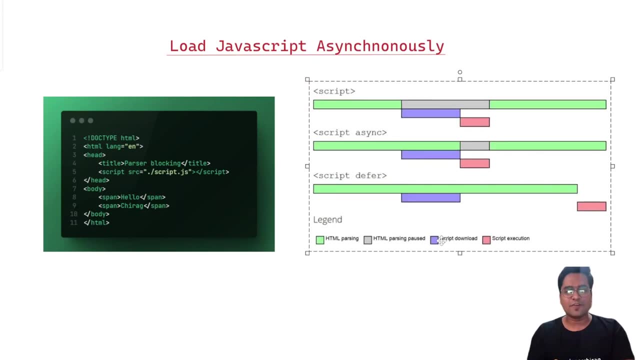 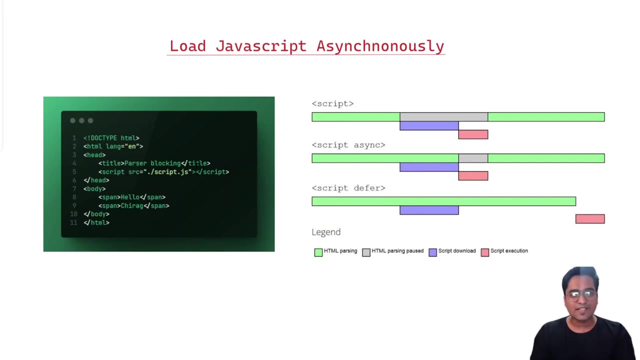 right. This is something which probably I can't be at. What else can we do? Let's talk about the other alternative. Most of the folks may be aware, but let's talk in a different fashion altogether. This is this time. Now, what if I say, with this script tag, if I add a small thing which is say: 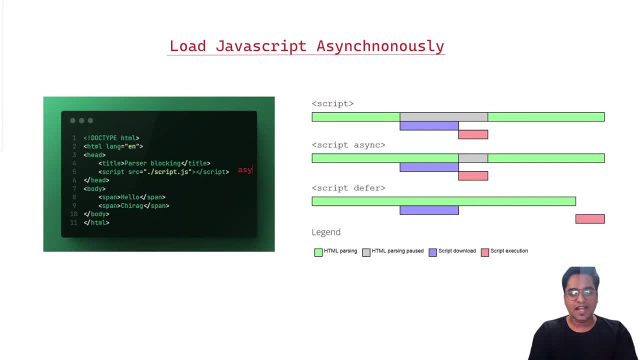 suppose a sink. I just go and say I wanted to make this a sink and we're basically a sink. I can make it as an attribute and I can attach it anywhere inside a script tag. right, I just add a sink. What it is going to do It is: let's try to understand with this, your script, or you can see. 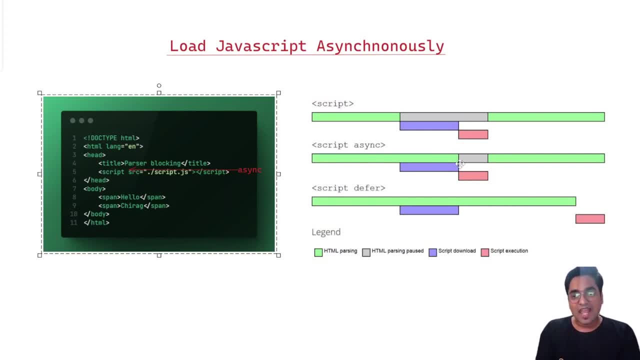 your HTML is basically getting passed and it, when it encountered a script. your script is going to be downloaded in parallel, But once your script is downloaded, the the execution of that script will hold the parsing. Your parsing can't be done in parallel, So what you're going to do is you're 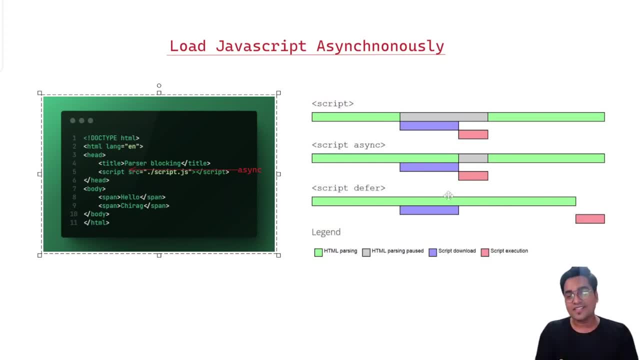 going to go ahead until this, that JavaScript is executed. Once the execution is done, then only the parsing is going to happen. Okay, Dude, this is again something very strange. So now, in this particular case, try to understand what is happening. So consider you again ready and you. 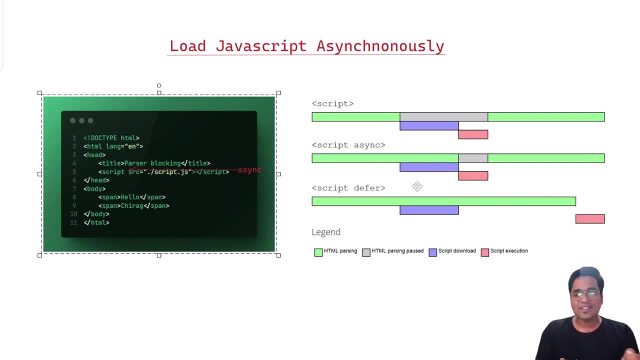 wanted to basically go for a party, What your dad says you can go. you can get the cleaning done on your way, maybe, but you have to get the Petrol filled before You leave for a party. Dude, this is again going to halt me for certain duration, but again it is. 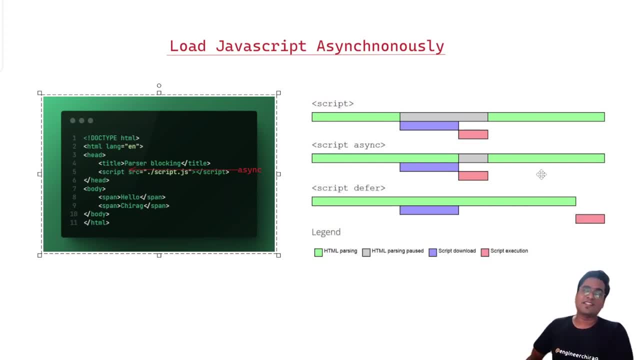 going to halt me in order to reach to the party with my friends as soon as possible? What is the other, better way? Now, say, suppose we can optimize the same thing by saying that I don't have I have to actually wait for the cleaning, or I don't have to wait for getting the fuel filled before 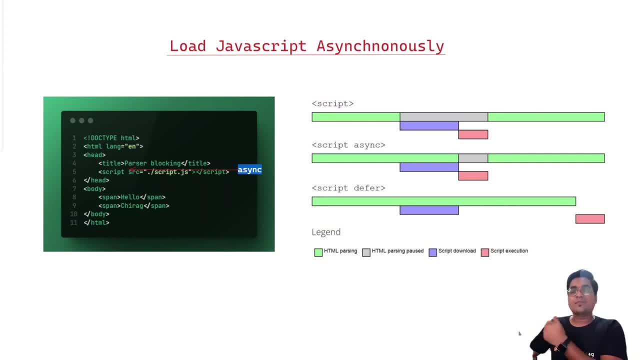 Actually I leave. I can do this thing on the way, or something I can delegate Once I am coming back from the party. how we can do that? We can use defer, So using this defer. we can use defer, So we can use defer. Try to understand what is happening, What you did, basically your HTML. 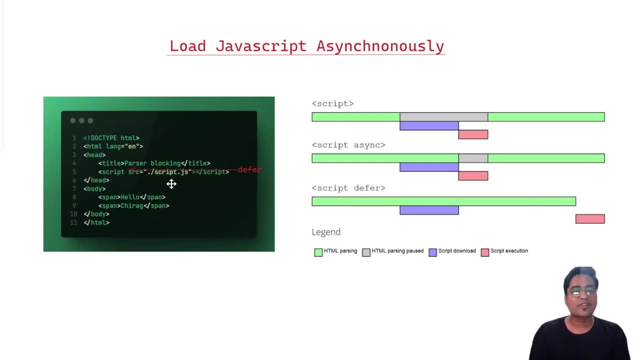 parsing will complete and there is no one who's going to hold your HTML part parsing What it meant by. you are going to see your content, which is listed over here, which is: hello, Chirag, as soon as possible. your passing is complete, but whenever it encountered your script, it will download that. 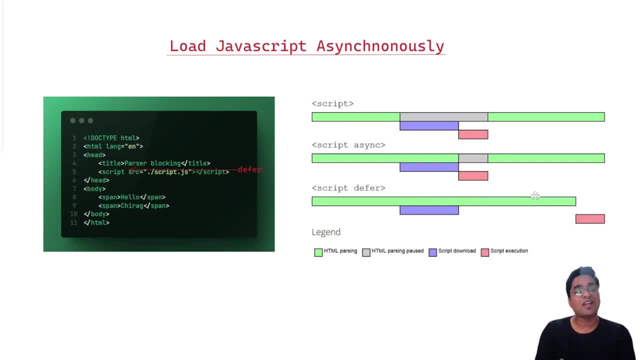 script in parallel, without halting your parsing, so that you can see your content as soon as possible. Once the parsing is complete, it is going to execute your script. It is as similar as you. you can get your vehicle clean on the way, but when you are returning back to the home, make sure you 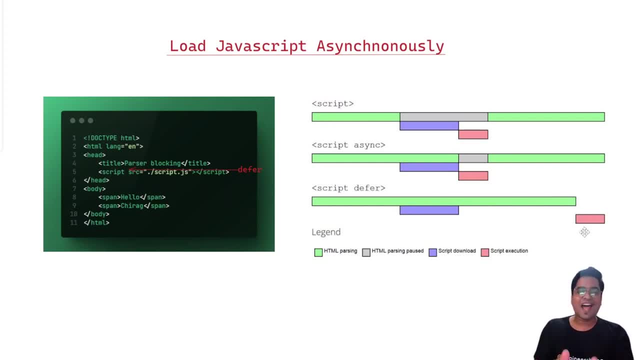 got your petrol filled, Yeah, So this is how, basically, your async behavior in JavaScript basically works. You you can see how you are leveraging your network layer, how you are leveraging your network layer with just adding few attributes in your script and you are making your. 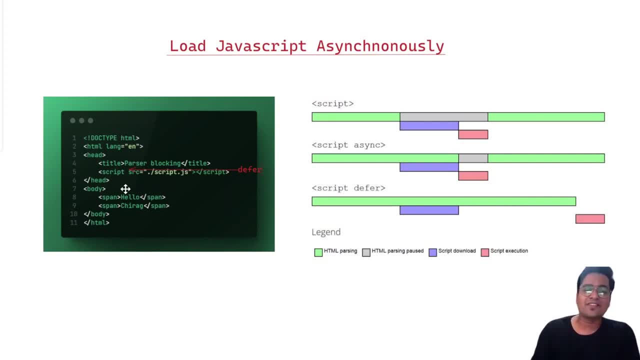 web application fast so that your, you, your users, your viewer can see your content as soon as possible. Okay, This was one interesting thing. There are a lot more things that you can try it out. You can try it putting the particular script at the bottom of the body and let me know what do. 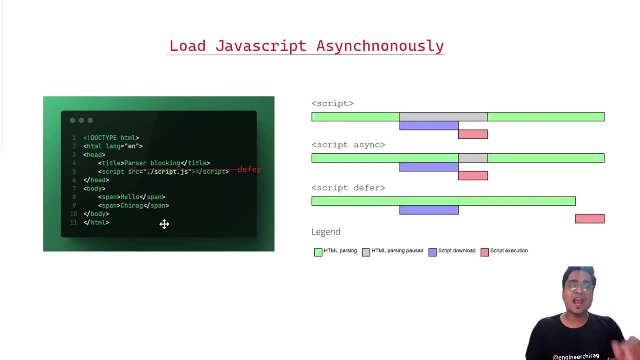 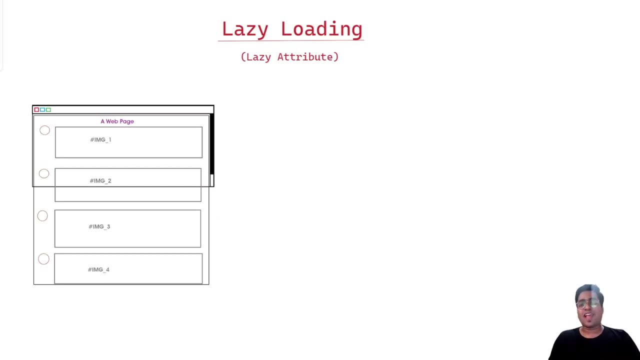 you see? Do you see a difference? by using async and putting your script at the bottom? So I will be waiting for your comment: Lazy loading. So this is another yet very powerful technique as the name of work in order to complete this. I will do this job in parallel of doing the other stuff, right? 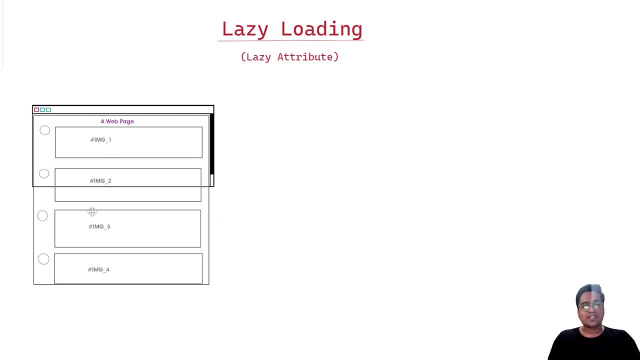 This is how, basically, the lazy loading does. So consider this example: we have a webpage, right, We might have used, like everyone uses, the Facebook or the Instagram, right? There are so many images in the Instagram, So many stuff that is behind the fold. What is fold, The thing which is visible in. 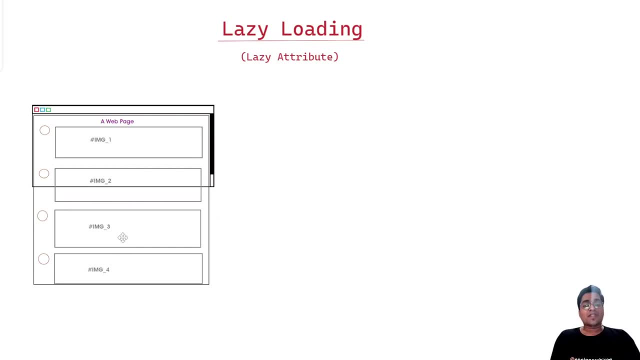 your viewport and the things which are not visible in the viewport. Now we wanted to load the stuff using the lazy load right. How we can do that? We can use a small techniques which will, out of the box, give this functionality in the feature. What to do? Let's see. We can use a small snippet which 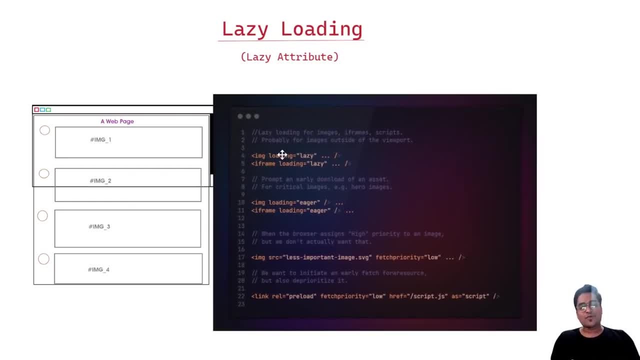 is going to help you with, which is there is new attribute which is called loading, and you can pass multiple values to that. There are two very powerful values that you can pass. One is lazy and second is the eager. What is this lazy and what this basically eager says? Let's 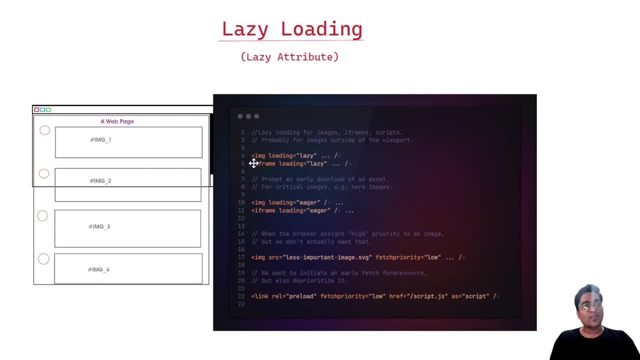 talk about that. So when you add anything lazy to any of your image or iframe, basically what it is going to do. it is not going to halt the parsing and the rendering of your webpage. It is basically going to load this particular image in a async fashion. Now, lazy doing a lazy load, right. 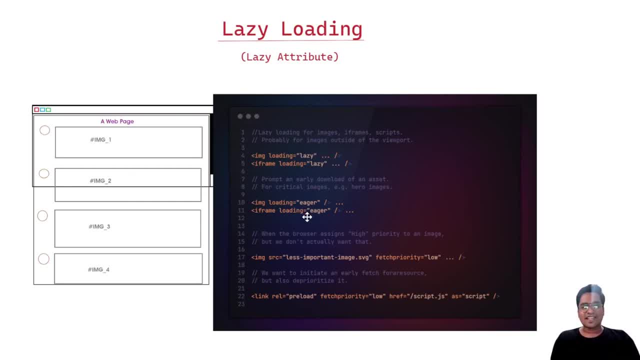 Now, what are these two values? One is the lazy and second is the eager. So consider example: you have added this value in in something like on your top of your screen which is logo Right Or something, some images or some icons which are visible, basically using the IMG tag on. 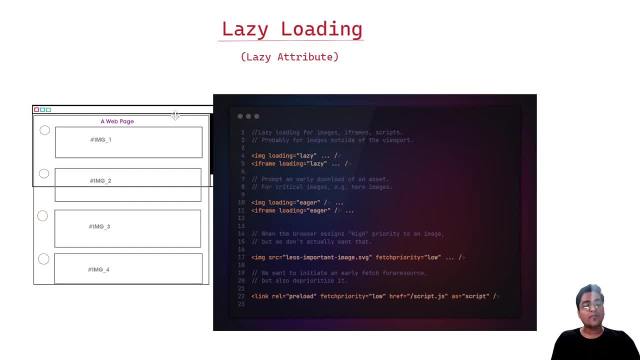 your header or something which is basically available on your viewport, on the first screen itself, Right. In that particular case, you want to load your hero images or hero asset in a eager basis, As the name says: eager- I am very eager. I'm hungry. Just give me as soon as possible. 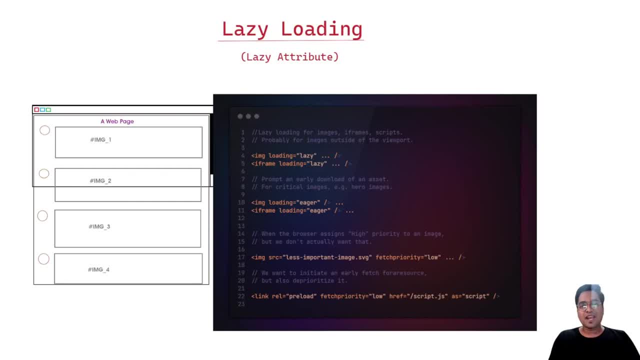 but don't halt my rendering of my webpage. In that particular case, you can definitely use something called loading eagerly, Now anything which is behind the fold, just use which is loading lazy. Now, what it is going to do? It is going to basically parse your webpage, render your webpage. 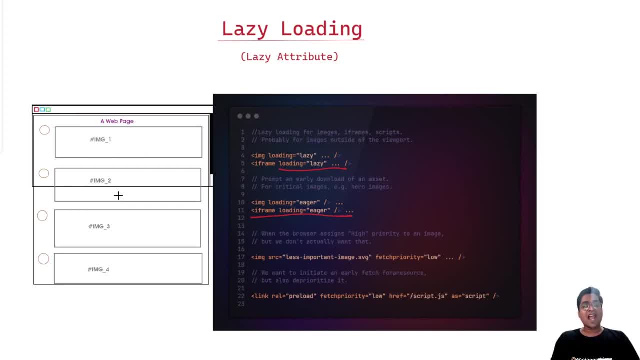 load your images on the first fold with the eager fashion and anything which is behind that viewport. Basically, you can load it using the lazy tag. This is going to give you a lot of benefit Now, even in your first fold. say, suppose you have a hero image in terms 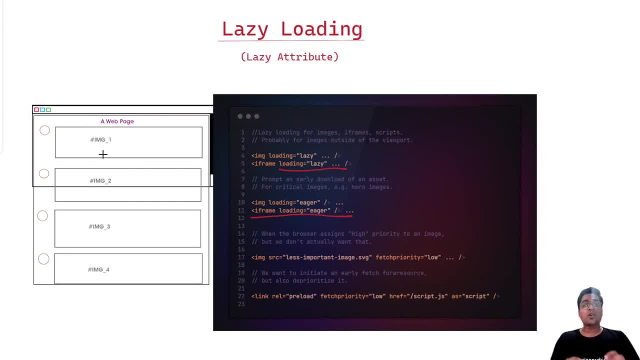 some banner, some logo, certain things which you wanted to load even at a faster rate. you don't want to load certain carousel images which is at the bottom of your viewport, you want to basically showcase the banner or your logo as soon as possible. even then you can decide some varieties among the p, among the pieces which are. 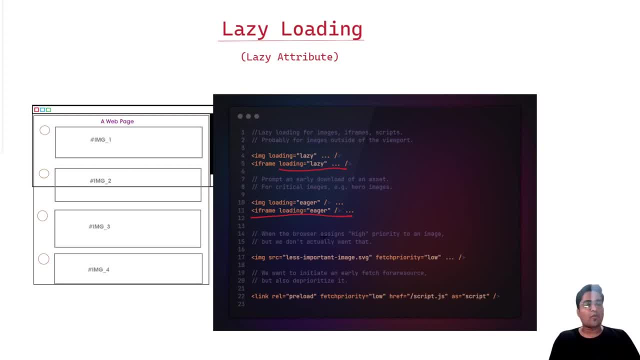 doing you loading using the eager fashion. so how you can do that, you can use something called priority. this is very, very important, very, very interesting concept. so what you can do, you can add an extra parameter, extra attribute which says that load with me with low priority, so anything. 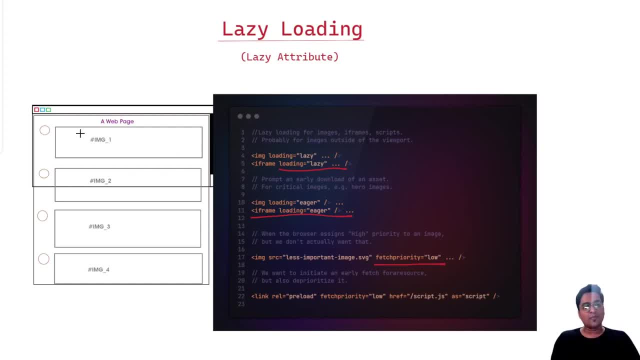 which is in the, which is of the low priority in your viewport. you can put this attribute and your browser will take care of that. definitely what it meant by. you wanted to load your logo in a eager fashion, but you wanted to load certain images in your eager fashion, but again you wanted 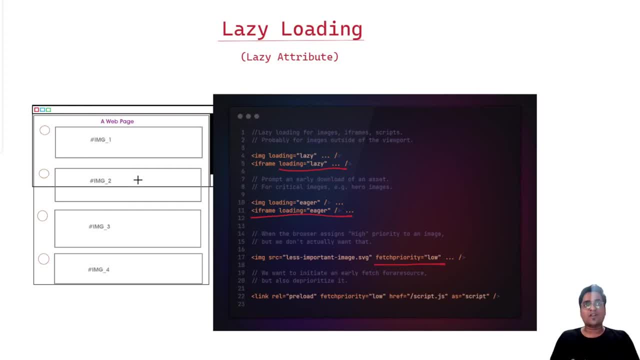 to set the priority of it in a lower fashion. right, you wanted to set as a low. this is very interesting thing. it is very small feature, a small thing that you have to add in your uh document or in your code, basically, and this is going to give you a lot of benefit. just go and try it out, although you 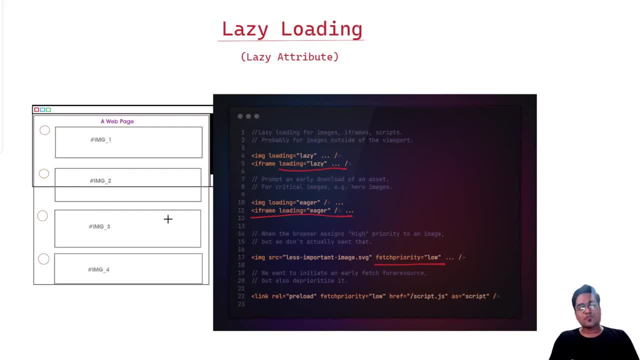 have to apply certain strategies, depending on when you are coming to the viewport, how to decide basically what to mark as a lazy and what to mark as an eager. we will be talking about those things in the coming episode as well, but this is what i wanted to highlight in terms of the lazy attribute. 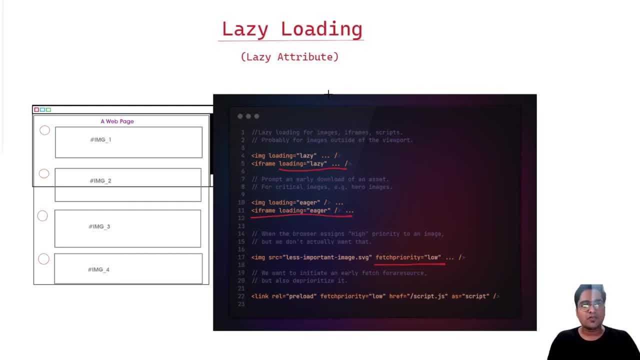 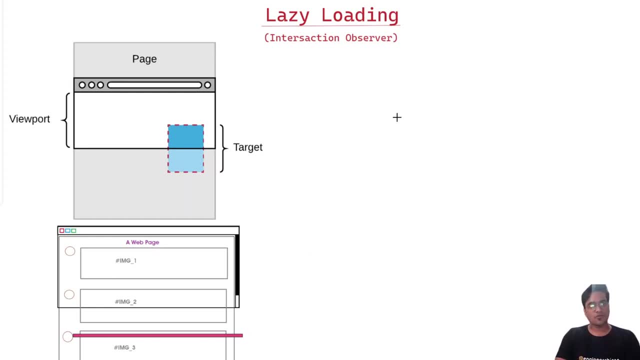 which is going to give you a lot of benefit. just go and try it out. we will be talking about another easy loading technique using intersection observer. this is a web api which is provided by browser so you can easily use it using window dot. uh, you can say intersection observer, so let's try. 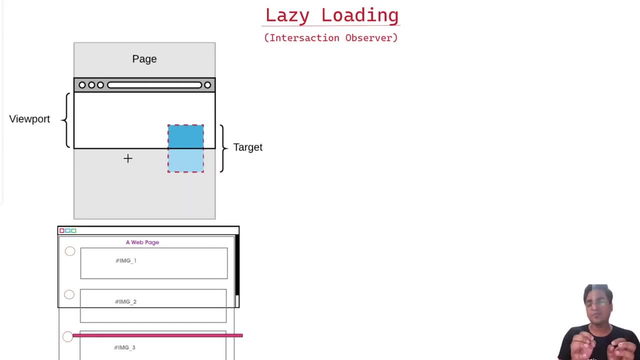 to understand this concept. what happens, although we? i have covered this in more detail in one of the mock interview which is related to autocomplete. you can find the link in the comment. you will get the detail, but let me brief you how this is basically happens. okay, in this particular 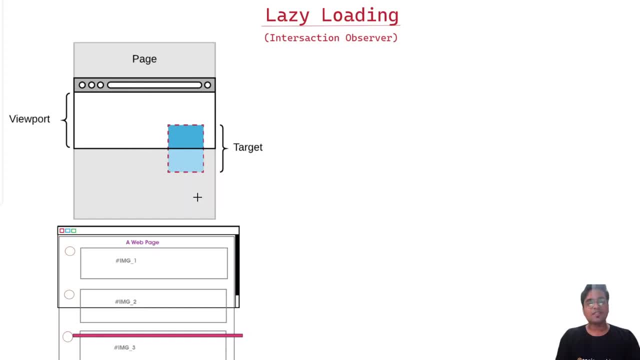 case. this is our viewport. so consider: we have so many images like flipkart page, where you have, or you can say, product page, or you have infinite scroll or something. say suppose you have google photos, where you have so many photos and so many content to be loaded, or so. 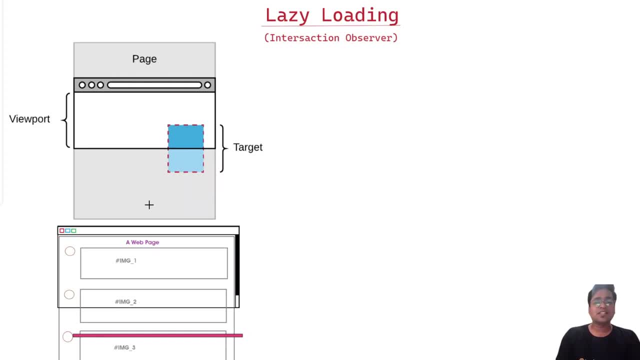 many visits that need to be loaded right. so in some, in such cases, basically what we we can do, we can actually add some element at the end of certain, you can say container or the div, which act as a sentinel element. we'll talk about that sentinel. what is that sentinel? so basically, if 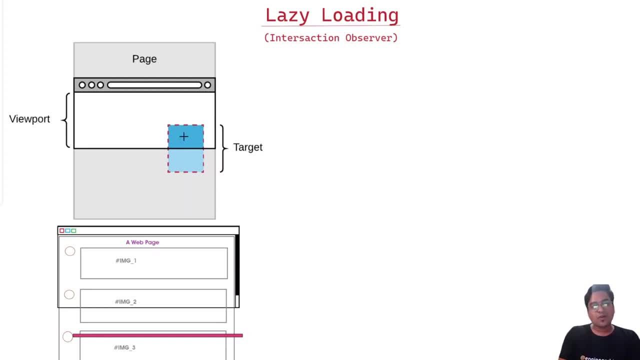 we are. when we are scrolling and we encounter that particular element, we can basically take a decision: dude, i want to load some other items as well. so for this we don't have to believe you can say you have to wait on the scroll or you have to trust on the scroll event, because those scroll events are very glitchy in. 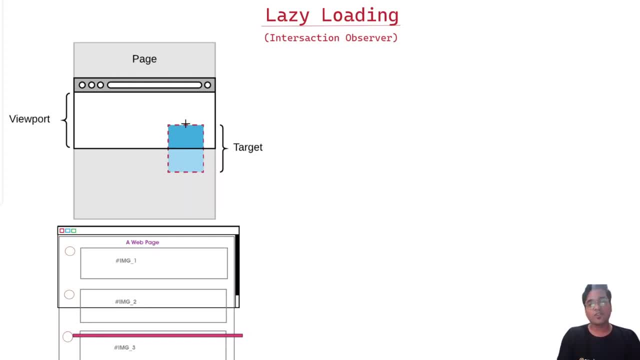 terms of the performance. so you can use this intersection observer where you define this element as in sentinel element and whenever your browser basically intersect that particular scroll intersect with that particular sentinel, you will get an callback and based on that callback, you will be able to make a decision. didn't understand? don't worry, we'll see the code. 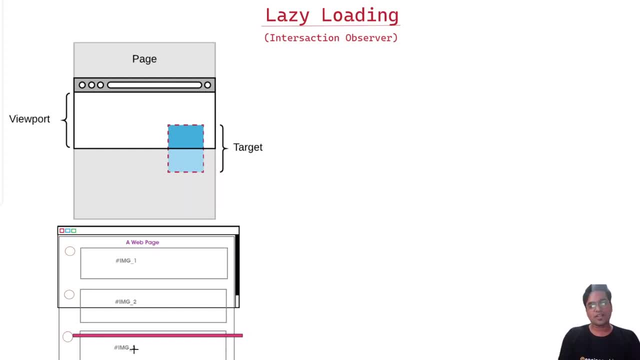 we will try to understand from that as well, but from this particular image you try to understand. you have image one, two and you have three and sort of thing. you don't want to load everything, all the images, right? you just wanted to load first two images or three images, and once you 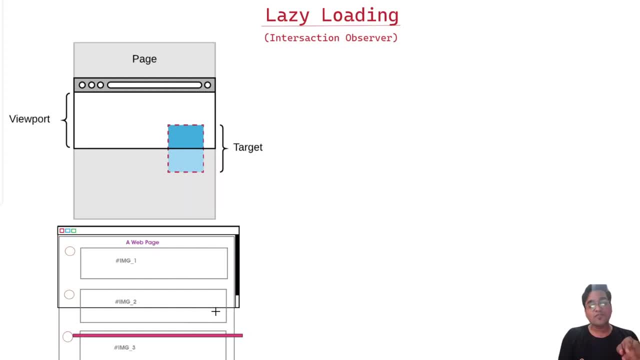 basically have these three images in your viewport, or you have seen these three images. you wanted to load more images, right, how to do that? so after these two images, you added a sentinel element in dom. once after scrolling your sentinel elements come into the viewport, you will get a callback. 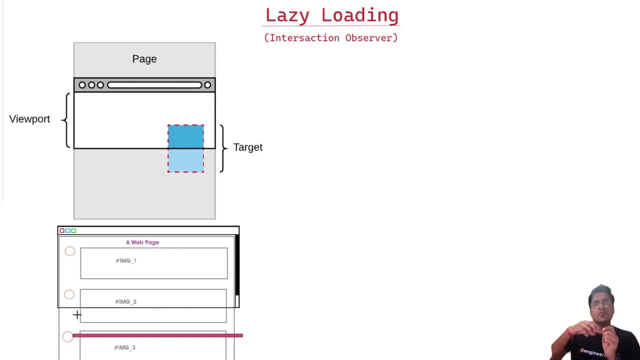 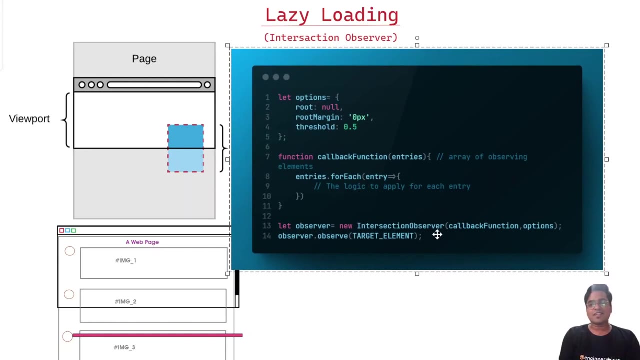 using that callback, you take a, you can take a decision to make another set of api call, get the images and add those images in your image list. that's it. let's see from the code how, how you can achieve this. okay, what you can do this is: this is the intersection observer api that we 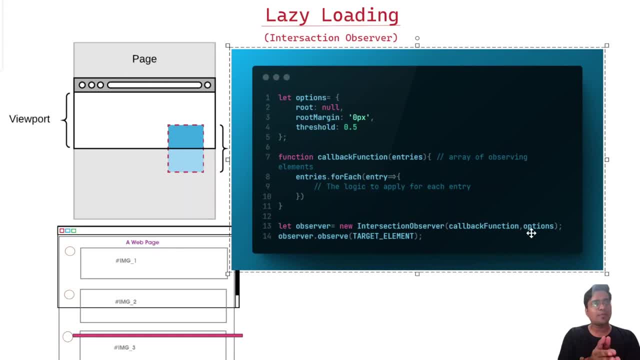 were talking about. you can create an instance of that. it gives basically two capability. one is the callback, which will be triggered whenever you encountered that particular sentinel element, and second is basically set of options. we'll be talking about both of them, but what we need to do 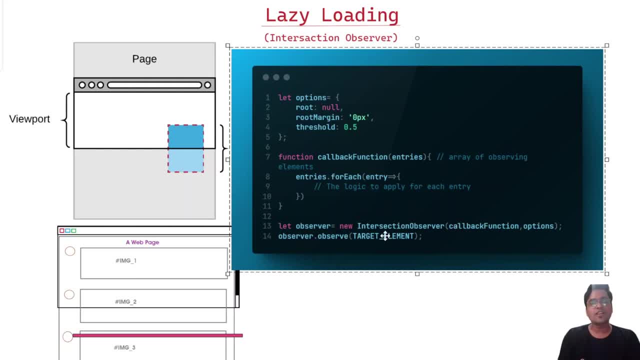 once we basically create an instance of this intersection. observer, you have to observe our element, which is, as we we can say, a target element or a central element. in this particular case, the sentinel element is this which we have created and added in a dom. if you wanted to try out, you want. 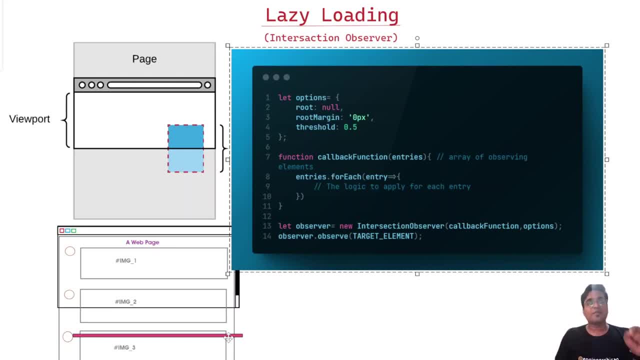 to see how basically it look like, go and check out the autocomplete mock interview. you will see a description and detail implementation over there. but over here, what we are basically doing, we are passing certain options. what are those options? these are very important and interesting thing. basically. one thing is: basically you have a route. say suppose you actually want a scroll in certain 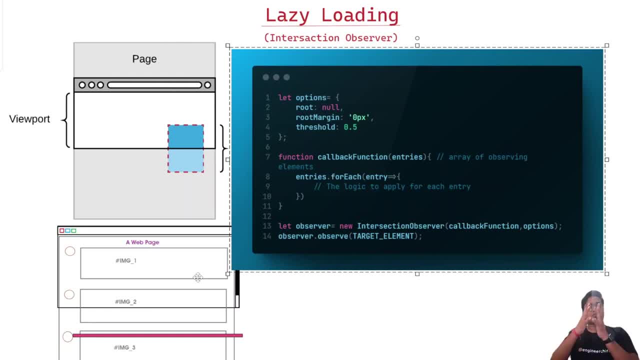 portion or certain container inside your viewport. you don't want to actually do a scroll and do these strategies on the entire viewport or a document. you want this scroll, you want this infinite loading- you can say lazy loading- basically inside section. maybe you have a search box or search pop-up which shows some suggestions you want. 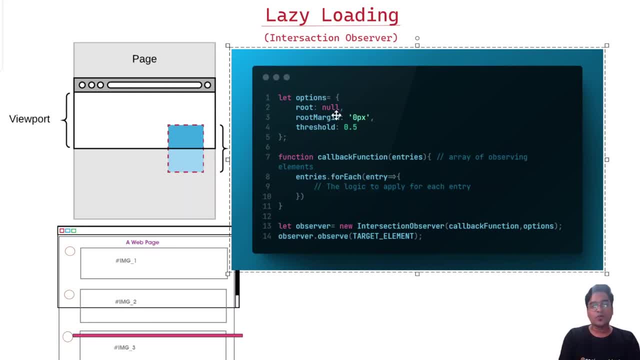 this capability over there. in that particular case you can define your route to that particular suggestion list and there are certain two, two parameter, which is root margin and the threshold. threshold is again very important and interesting part. say, suppose this particular sentinel is wide enough or have a good amount of height. in that particular case you wanted to make sure, even you. 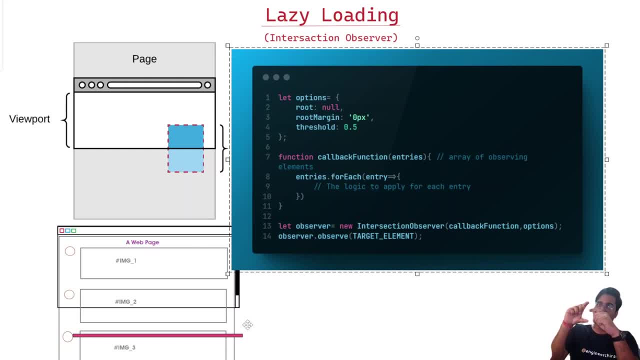 have actually crossed 50 percent of this div or the container. you wanted to get a callback. based on that callback you wanted to make ipa call. why this is important? this is interesting you can consider you have certain images. once you are actually crossed 20 or 30 percent of that image, you wanted to make sure. you want other set of. 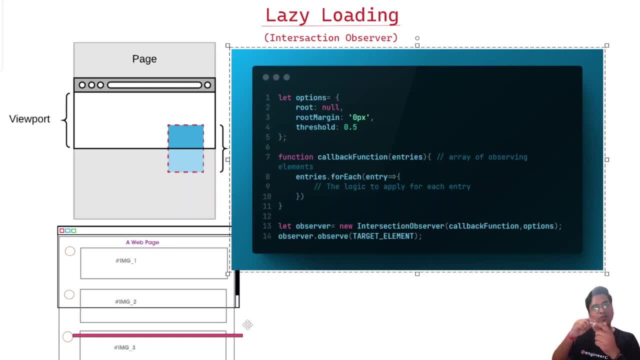 images right. in that particular case, you you don't want to give a loading experience to the user. that's how this is very important and interesting and this is a callback which you get and you can do a lot more thing with the entries that you get as in parameter over here. 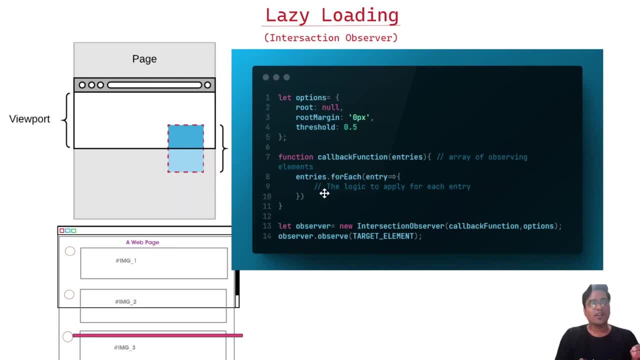 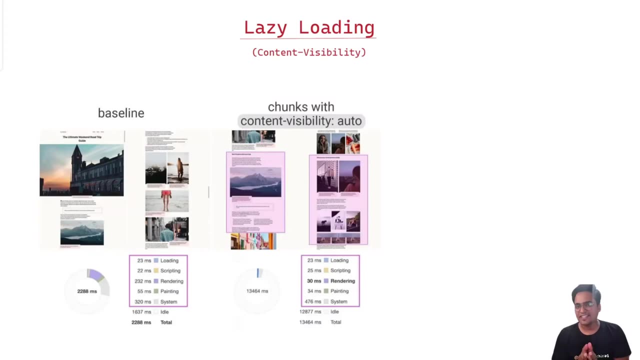 so if you haven't tried, just go and check out the mock interview related to the autocomplete and go and try out this particular intersection observer. this is going to a standout thing and you will come back to thanks me. content visibility: this is another very powerful way to lazy load, and that, too, with a very limited 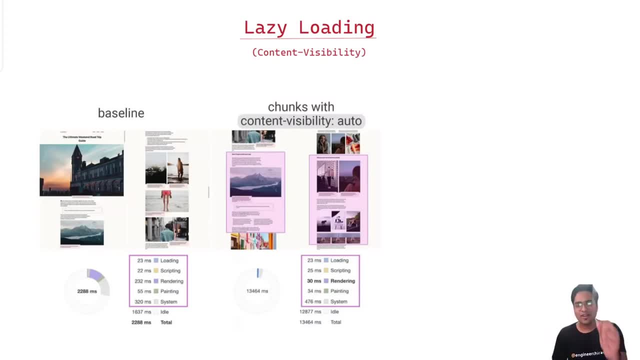 code changes that you have to do. you have to just add one property in your css and out of your load name. you really are going to get a lot of improvement. so let's talk about that. so in this particular case, consider: you have a web page. your web page is getting rendered. it has multiple folds. 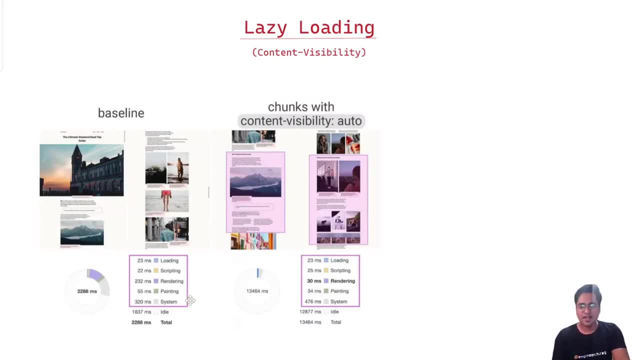 you see, you will be having a loading, you will be having some scripting time. there is a rendering, painting and system time. right, in this particular case, very important thing which you have to notice, the rendering time which is taken from example, which is 232ms by just adding a content visibility. 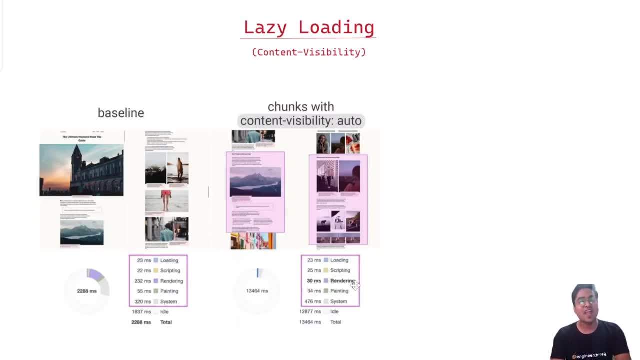 auto, it actually reduced to 30 ms and what it does basically try. let's try to understand: by setting content visibility, which has multiple things, which is like hidden, you can set visible or you can set auto auto, is something which is very great out of box. what it says, that anything which is not 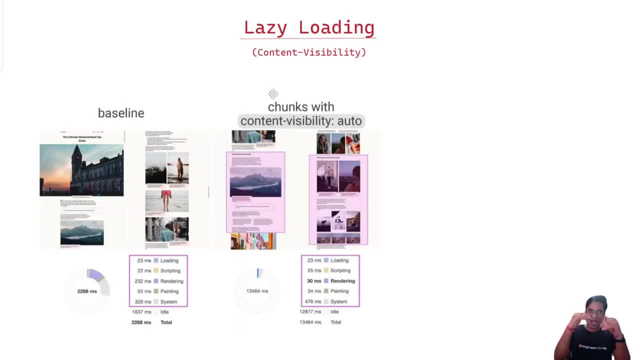 visible in my viewport, i will do a lazy rendering of that particular thing. i am not going to render it until this basically user is actually scrolling or reaching to that particular point. so it will just set the priority of the things which are on the first fold or in the visible area. it will try. 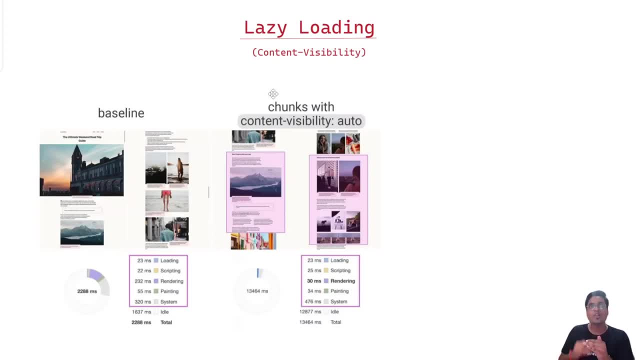 to load and render those thing and anything which is behind the phone. it is going to do that in a sync fashion or you can say in the lazy load fashion. this is damn cool. so it gives lot of other functionalities and capabilities, which says that even there are certain things, there are other. 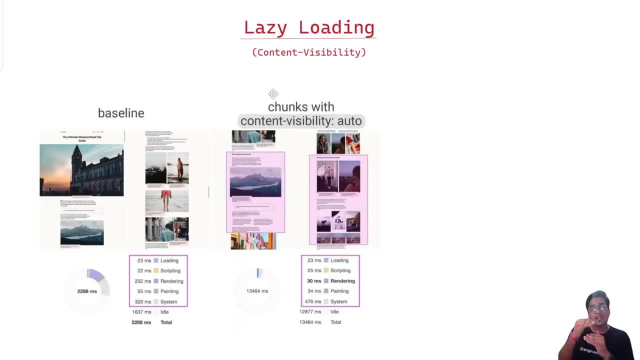 attributes which you can try it out, which is like hidden sort of thing, even it does like got rendered, but your screen reader is not going to attach those things or the screen reader won't be able to basically read those things until unless you actually scroll to those things. 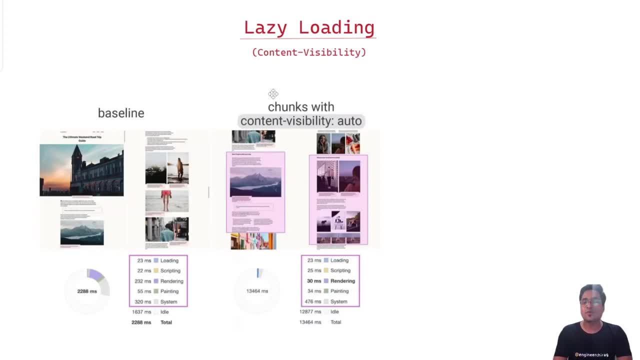 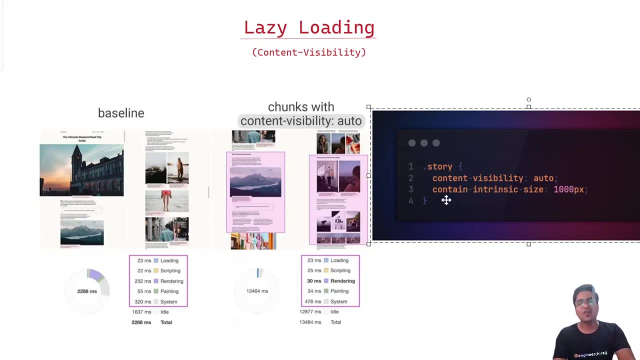 so there are so many things which is done behind the scene in order to improve that too, with just simple thing what it says, that it just says that content visibility is auto. and there is another property which you can set in order to just let browser know what is the size of the content. 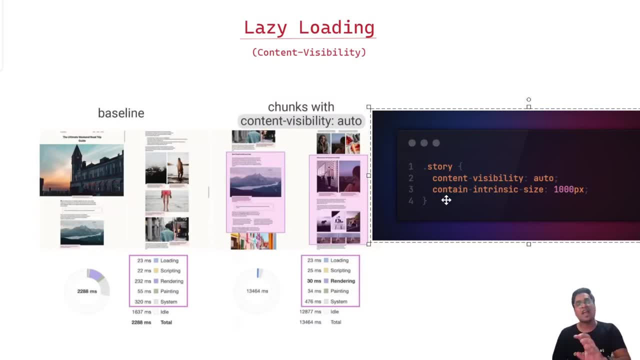 which is going to be loaded in order to make this decision and optimization better for you. if you can predict this is well and good. even if you can't, it is going to do a lot of thing for you in terms of the setting, the content visibility. so if you haven't tried, just go and try it out. 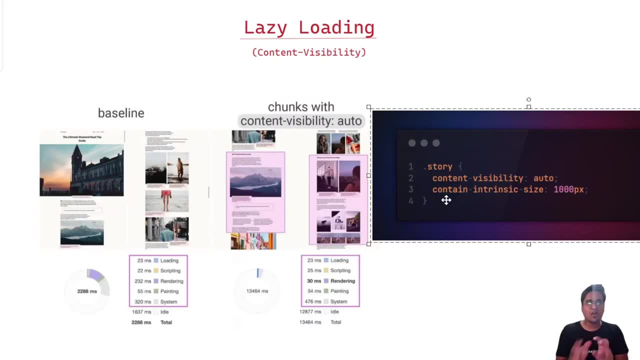 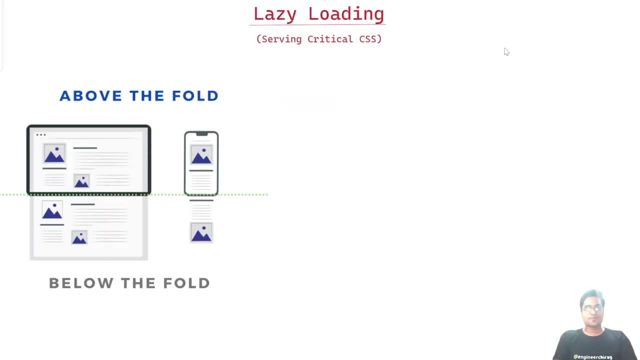 it most. it is supported in most of the browser but, yes, always check for these special properties, the backward compatibility or the browser compatibility, in order to try it out. let's go through another technique of lazy loading which is serving critical css, as the name suggests. we have to make sure only the css which is critical. we should load and rest. 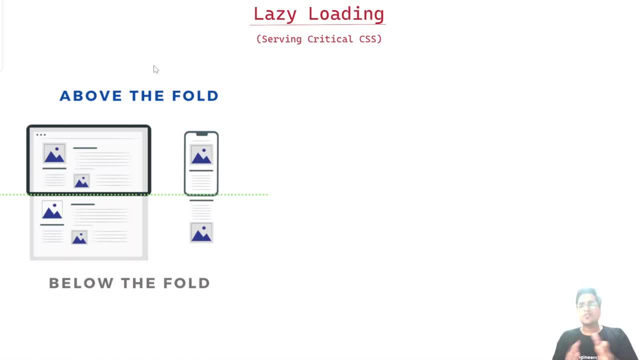 we can load afterwards. how can we do that and how it is going to basically benefit in the network layer? we have to think your css can be multiple kb. sometimes it can be in mbs in some of the time if you have not optimized and it takes some time in order to load from the network right and 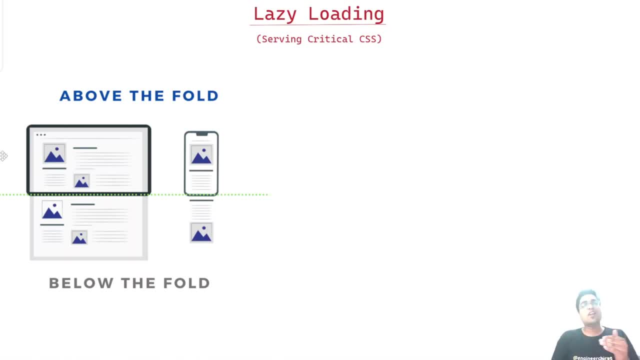 if you don't optimize, if you don't think about that, it can basically halt your rendering on your browser. right in back to the mainchannel, we had a big 항상 section where we are trying to make sure only the css, which is critical, we should load and rest. we can load afterwards. how can we do that? 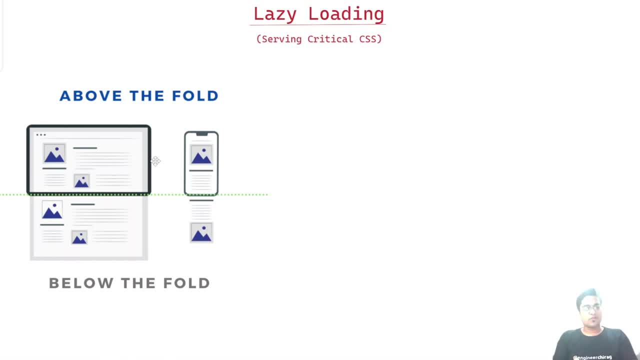 in that particular case, what you can do. we have above the fold, below the fold, if you can segregate your above the fold critical css in a different file and rest other css which is not critical in the other file, and you there is. there is a technique which says that make the first thing. 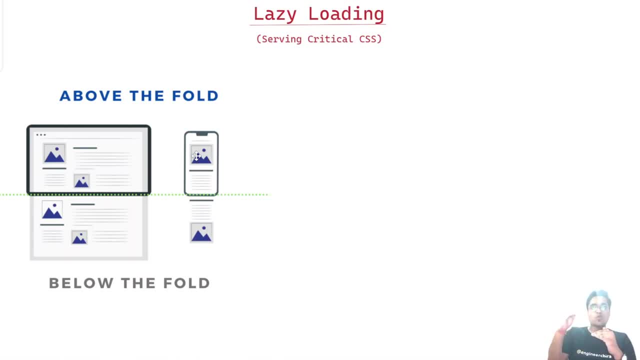 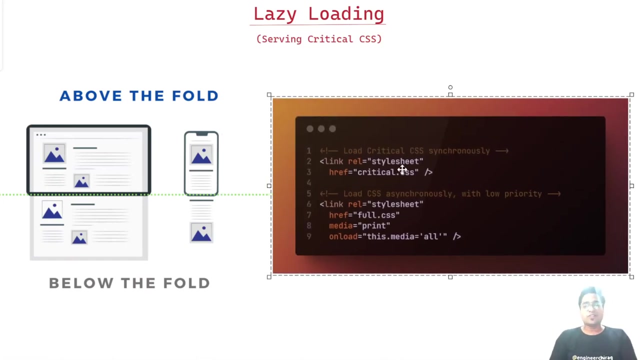 which is blocking, and make sure once it is downloaded, passed, and then only your web page basically renders. the rest is something it can be downloaded async and in parallel, basically using the lazy loading technique. how you can achieve. let's quickly see that. okay, so there are two css. 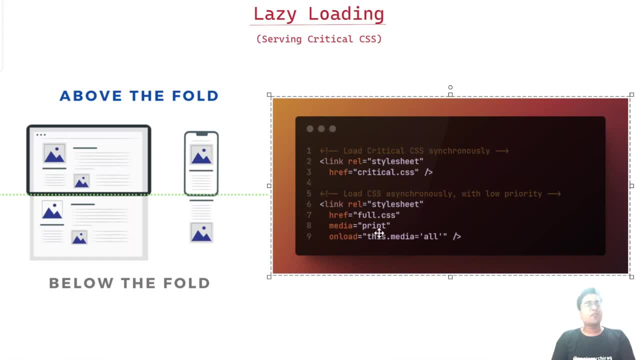 basically, we have broken down: one is the critical dot css and other is the full css. in that particular case, what we are doing- the first one is something which will block your rendering until, unless it is downloaded, it is your web page is not going to render. but in the second one, we are 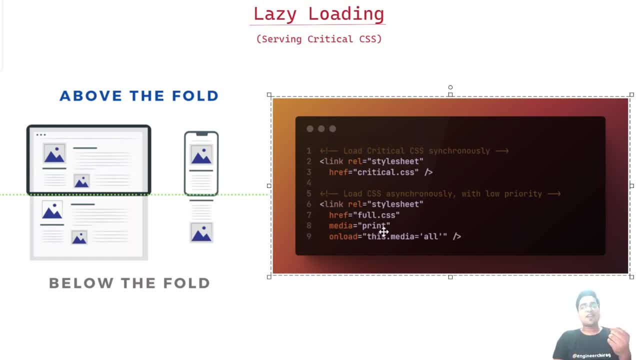 using a trick which says that this css is having a media type of print. so, dude, this is not something which is very critical. it will only be used for the printing purpose. but on the same time, we are saying: just load this. once your web page is loaded, your javascript is. 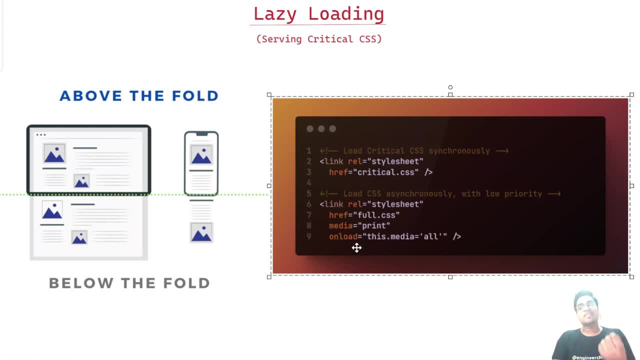 ready to execute just on load in that particular case. load this on your document. load. make this media file as an all which is eligible, or you can say available for everyone or for all the use cases in the css. what it is going to do, it is going to download and make it available for your next. 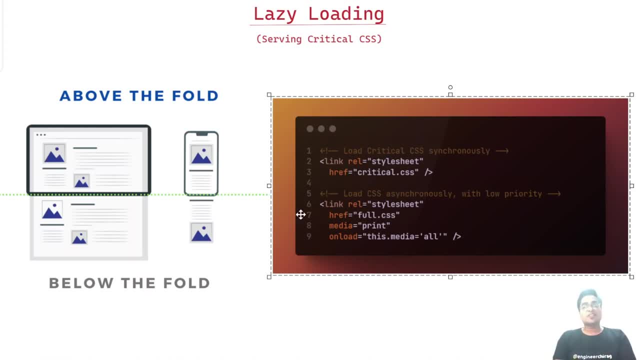 trending and next set of things which are available below the fold. so this is what we are going to do. this is very cool technique and this makes your css non-blocking in terms of your rendering. just go and try it out and you will definitely see a major performance boost. right, just make sure you. 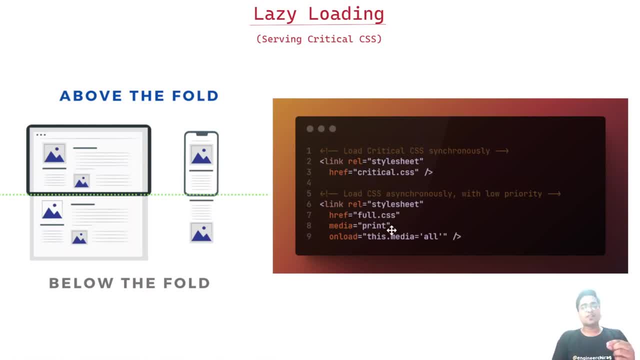 you should not put anything which is very critical for the first fold inside your full dot css because in that particular case you will see some of your pieces of your application or your web page are breaking right. so anything which is related to the number sidebar, you want it to be loaded on the 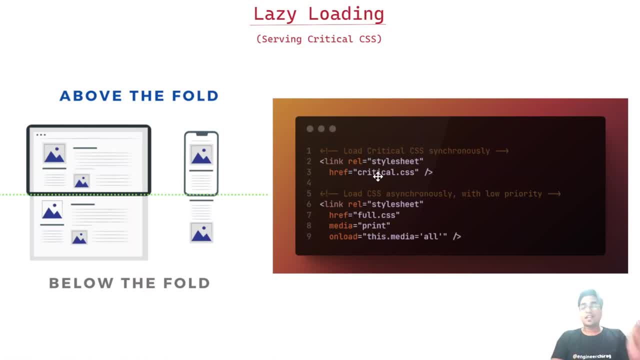 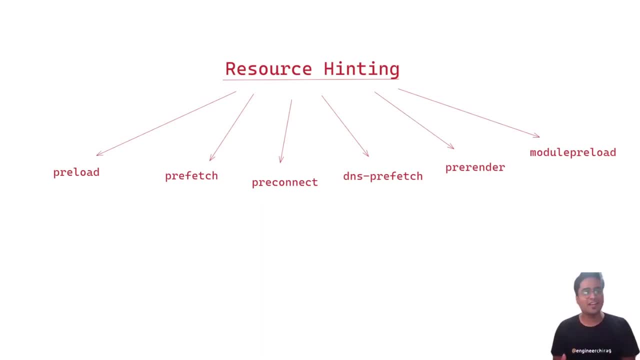 full dot css. make it available in the criticalcss. give a try. resource hinting: this is one of my favorite topic. like i, i really love talking about it. okay, so is there any way, as the name suggests? is there any way can we give a hint to the browser that these are the resources that are going to be? 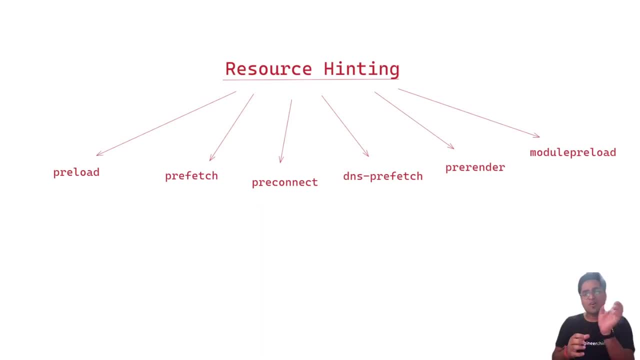 used or you can take some decision based on these resources. given some hint, i will provide you some of the things that we can give to the browser so that browser can be more optimized or it can make some network call or process certain things on a major priority basis, right? so what are those? 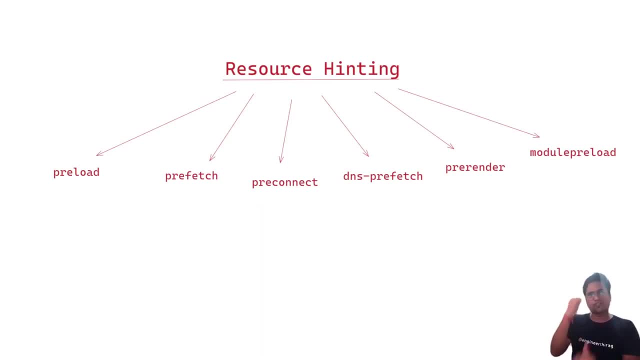 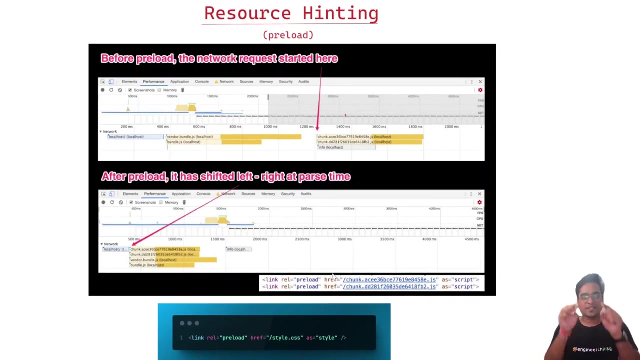 things. what are the different hints? basically we can give to the browser for the different different resources or the asset that we have. first come fast so we can give preload, pre-fetch, pre-connect, dns, pre-fetch pre-render and module previewed- what are these? and one by one preload. okay, so we have a web page. in this particular web page we have certain 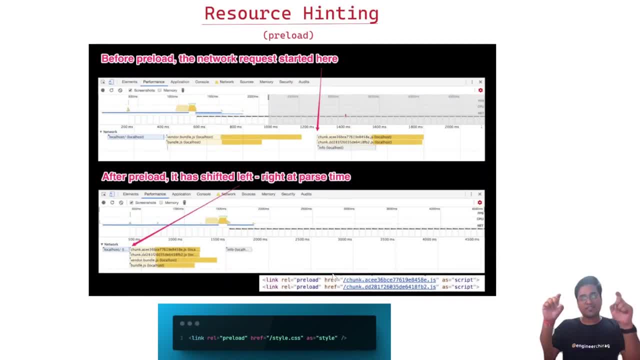 javascript or there are certain css right. those javascript and css are going to be used just after you basically render your web page right in your rendering. it is required. that is critical. so in that particular case can we give some hint to the browser go and just download so that when 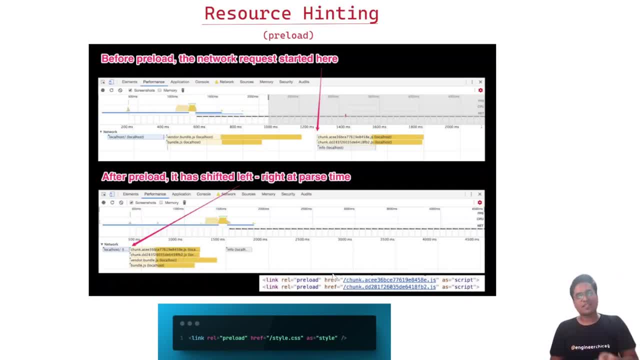 it is actually rendering. you don't have to wait while passing it. it knows already there is a request and it can leverage that. how can we do that? there is a small thing that you can basically do, which is which is you can actually add something called relation. rel is equal to preload in any of 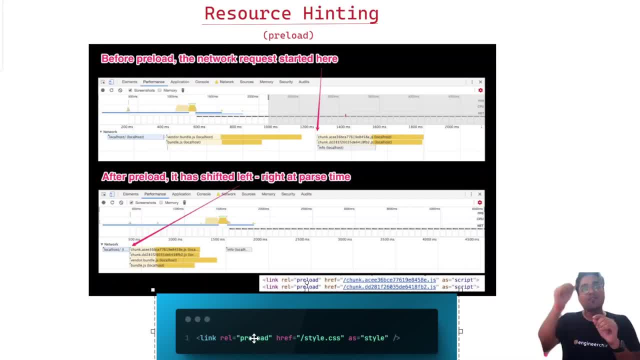 your javascript and css where your browser will understand when i am basically loading a web page. these are certain, certain things which is very critical and these are going to be used just in couple of. you can say millisecond or the second right. in that particular case, it will load and 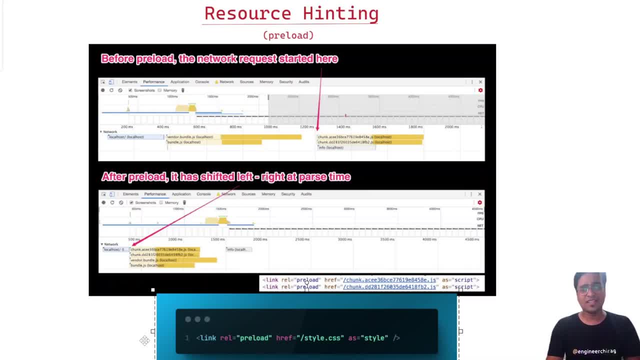 basically it will execute it now. in this particular example, you see there are certain chunks that will be basically used after. you can say, suppose few visits are loaded and these are basically used in couple of the visit and as these are lazy, loaded but we don't want to show the loader experience to the user. what? 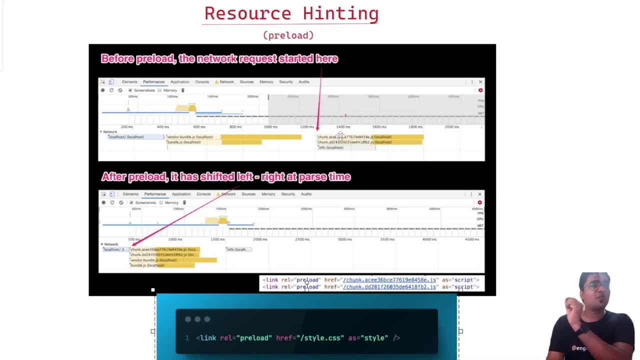 we can do. we can add a relation as is equal to preload. basically, we wanted to preload these asset or the chunk so that we don't have to show the loader what it does. it actually shifts the loading of these chunks at the start of your rendering of your javascript and css. you can. 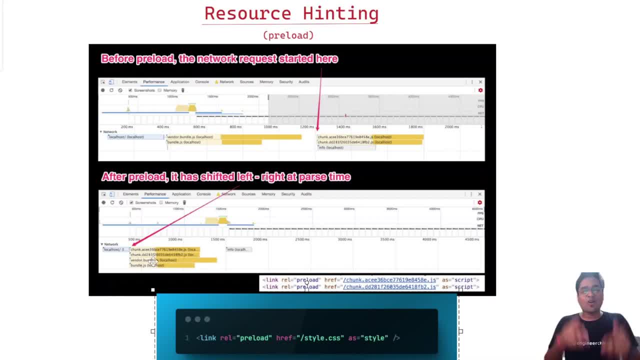 add these chunks to the web page itself so that it knows these are already downloaded things. whenever it is required, it can be used, okay, but every time we may wanted to load something in the background but we may not wanted to execute that because that execution can be unnecessary if 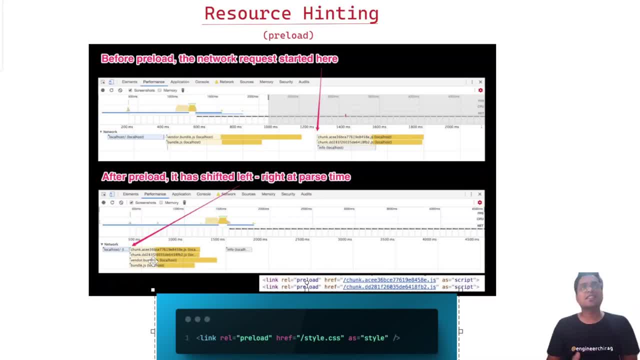 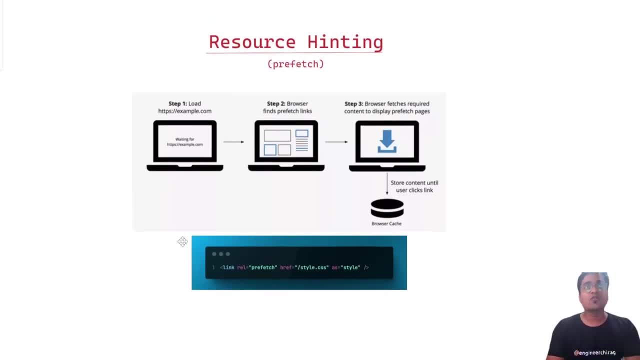 that is not available in your first fold altogether. right, in such cases, what you can do? okay, there is another hint that you can give to the browser, which is: i want to load, but i don't want to basically execute it. in that particular case, we can use, which is something called the preload. 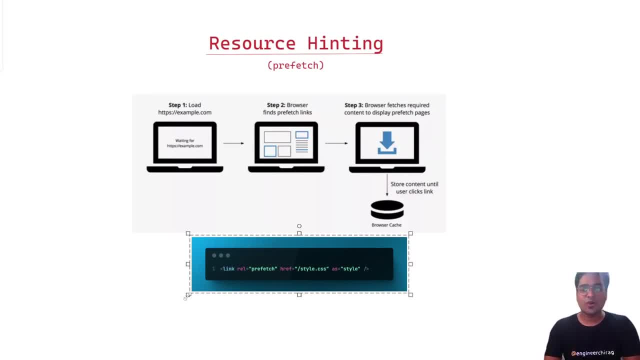 which is something called prefetch, which works like quite similar to what we have seen in a preload situation, but in this particular case it is not going to load, not going to execute. let's see we are loading. examplecom the browser finds prefetch link. what it will do? browser fetch. 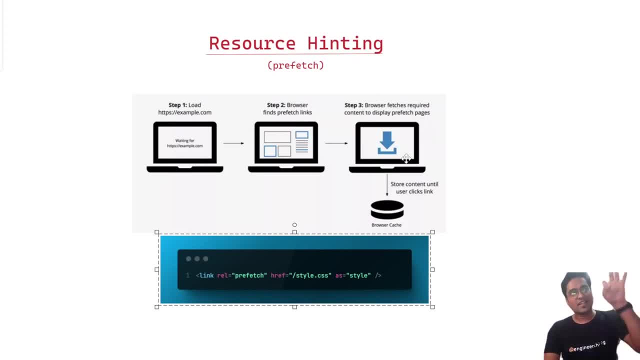 required content to display the prefetch pages and basically it downloads and put in the cache. so whenever you're at the time of your execution, at the time of your passing of your content, rendering it, if there is an asset which is needed, it will basically look from that particular cache, it will execute and basically it's available, that script, that. 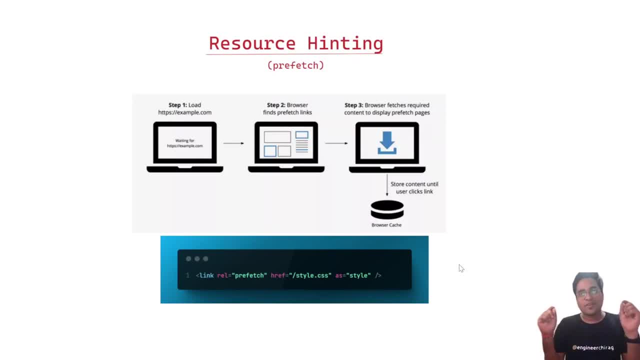 style is basically available to you. so where to use the prefetch? any place where you don't want to get it executed, because that is not going to be used right away, it is going to be used afterwards, right. in those cases, try to use prefetch. but again, there may be certain use cases where you don't want. 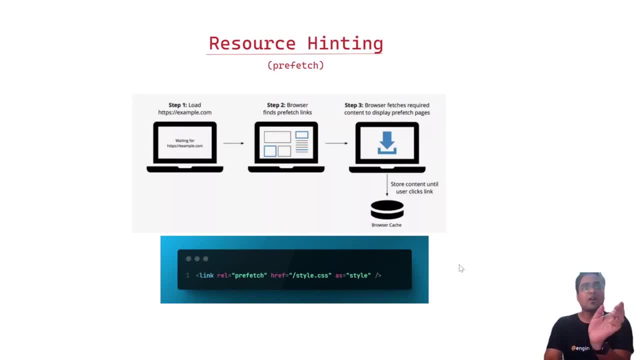 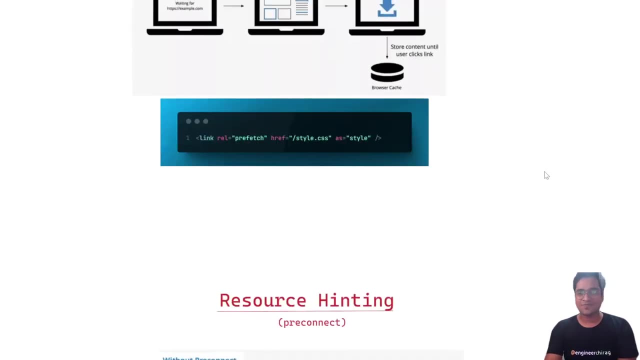 to even download those asset, because you may not aware of the complete url which is going to be used for your code or your your web page, right, in certain case you can use some other, you can say hints, which is going to be helpful. what are those? let's? let's see. the next thing is your pre-connect. 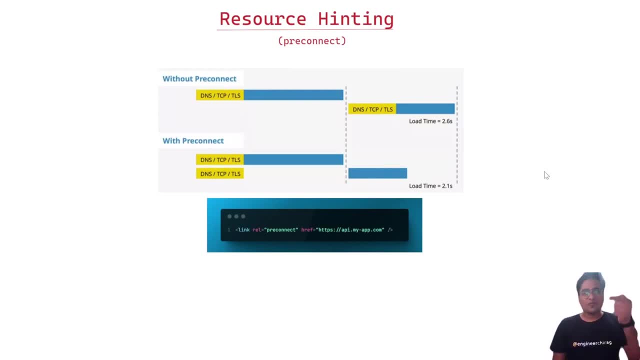 what it says. this is: this is very, very interesting and important. when you basically make any request to the server, it basically does: uh, you can say dns, tcp, tls, basically handshake, and after that basically it try to load a lot more thing. you make a request for the another asset. 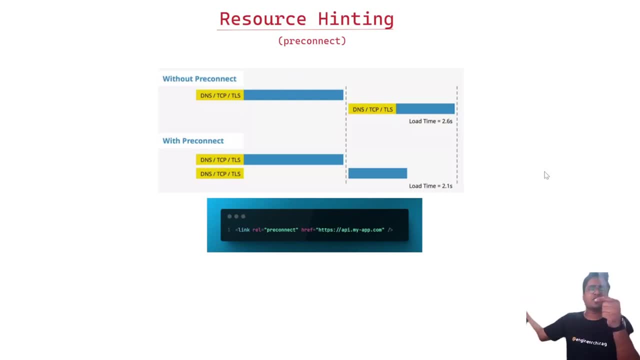 in. in that particular case also, it will do a handshake and then it actually try to load the thing, but, as you know, i have to load, say suppose, google font. i have to load certain things which are there in my web page. in that particular case i can utilize. i can basically prevent that handshake. 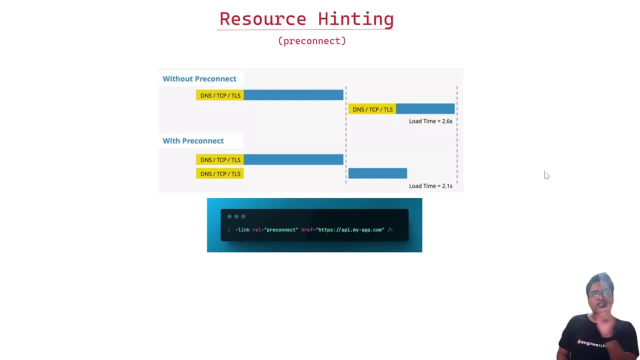 to happen at the moment when i wanted it to be downloaded, i can do this handshake pre-hand, so that it actually saved my time in doing a hi hello. so when you enter something, you enter a conference, do a hi so that when you have to actually ask a question in that particular case, you have already. 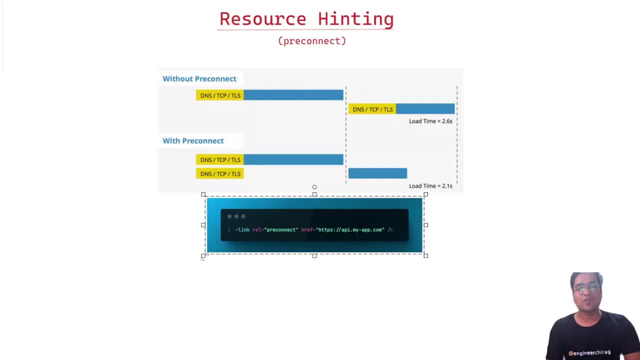 done an introduction. it's quite similar to that. in that particular case, what you have to do is nothing special. you use a similar kind of attribute which is rel is equal to pre-connect. so in that particular case, it will basically do a handshake with this particular domain, which or a sub domain that you 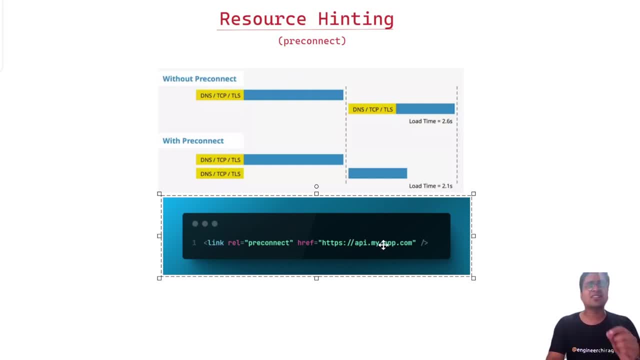 have provided so that the next time, whenever is required, it is just going to directly go and download it. pre-connect may not be available in all the browser because it recently started available, so, uh, you can try it out. another thing, which is which works in the similar fashion, which is: 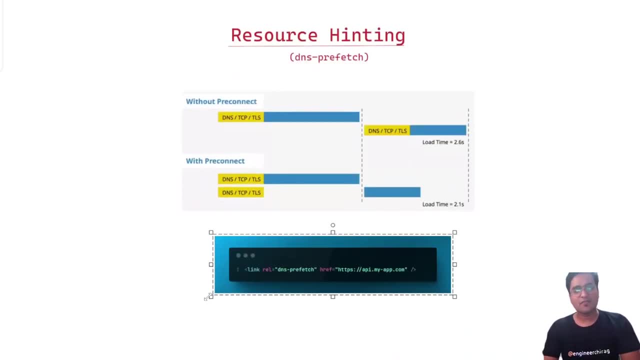 uh, you can use the dns prefetch. it is the same thing. what. what it basically does? it actually, uh, make a handshake and it is basically supported on the old browser, so nothing special. it's more about the fallback situation which you can see now. this is again very, very interesting. uh, hint that. 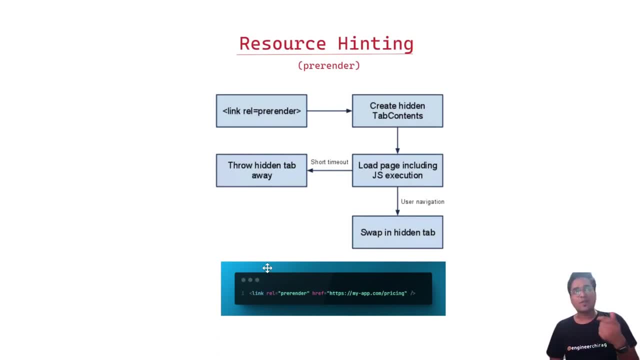 you can give, which is, say, suppose you wanted to basically render certain things or certain pages, or you users may be like going to request for this in the next cycle altogether, or users are going to basically click on a certain page and you know that these are the pages which are highly visited. 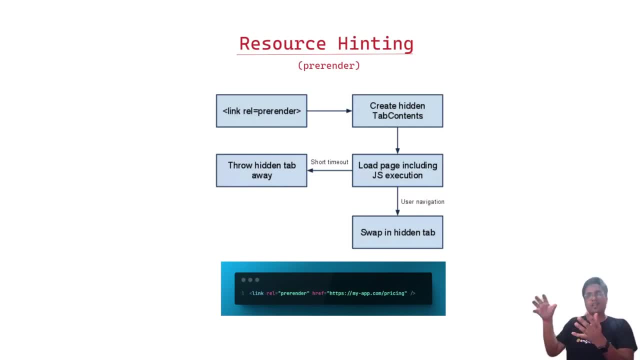 in that particular case, you don't want user to click navigate, then start requesting, then downloading. this is a very powerful what you can say. you can basically define any relation which is a pre-render or what it will do. it will create a hidden tab content with that hidden. 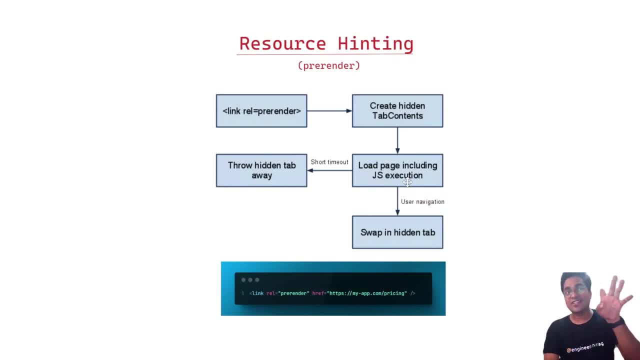 content. it will load your page including your js execution. it will execute. it will throw the hidden tab away once. basically after a certain time it will throw away. if the user navigate, you can leverage it. what it meant by you are on your main page and you know mostly when a user comes. 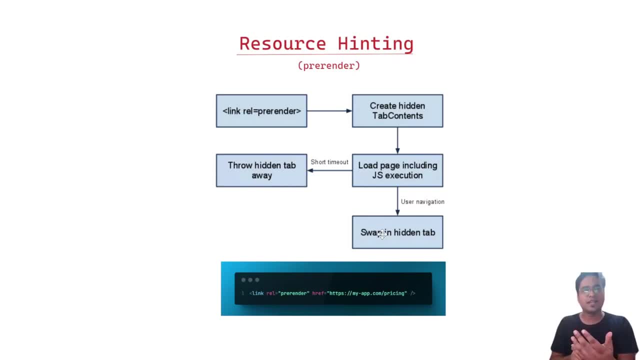 the user basically click on the login or they click on the sign up, and they are the two possibilities. most of the user are going to be doing a login and after login, you have to show the dashboard now, main dashboard. you have to show the dashboard. you have to show the main dashboard. 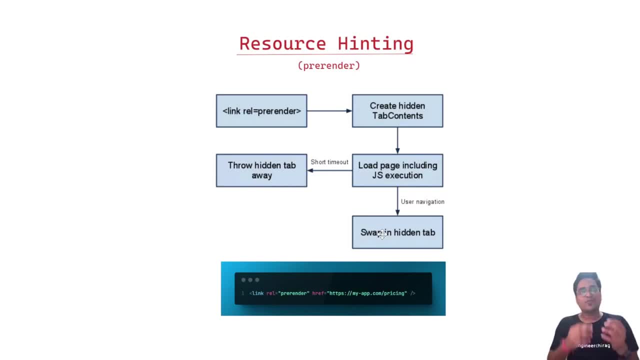 that is common for most of us right what you can do. once a user is doing the login, you can actually pre-render the dashboard out of the box and it will basically load in the hidden tab or the tab content and it will also execute so that once a user click on the login, they they redirect to a 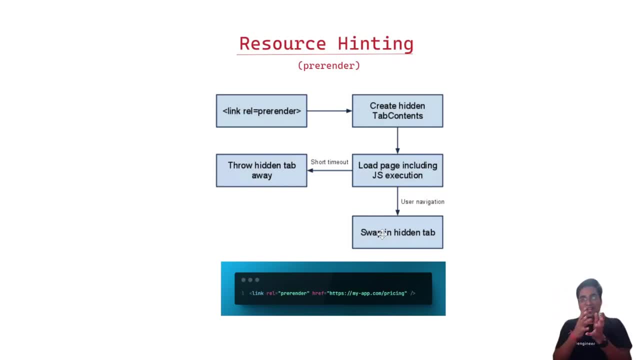 new page the user navigate to a new page where your hidden tab- the execution thing which happened behind the scene- actually shows up. so in no time you will see your next pages available then in there itself. but again it comes in addition as well. you will basically not need to heHa bude that. 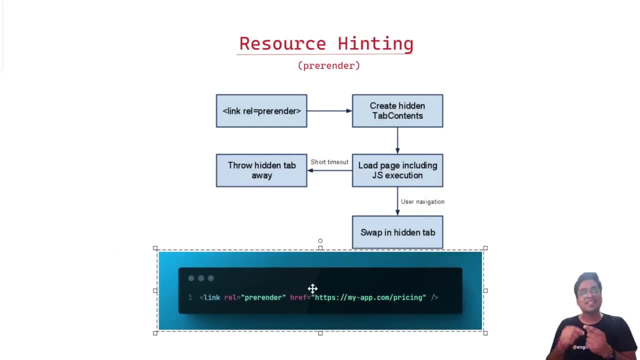 check anything. be in your view. all right guys. today i told you that you will see the levels to be pretty with the cost. you have to be very sure these are the next user, or next pages, basically, which a user is going to navigate. else you will end up unnecessarily loading lot of resources which 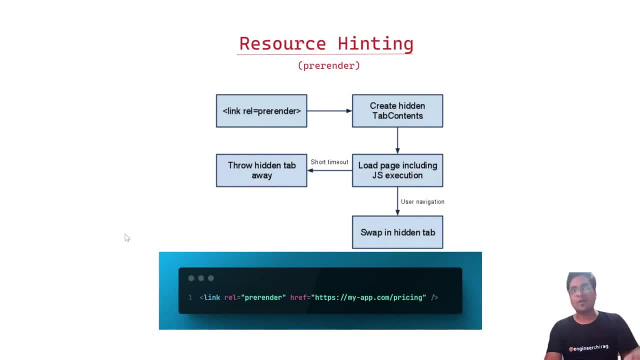 is not required and people who are in the low bandwidth or using the mobile data. they can actually end up wasting their data altogether right, or it can actually end up slowing down certain things. so use it with very precaution, but this is way powerful, trust me, this is way powerful. 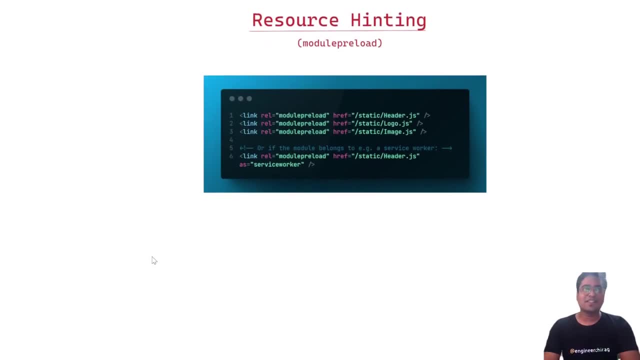 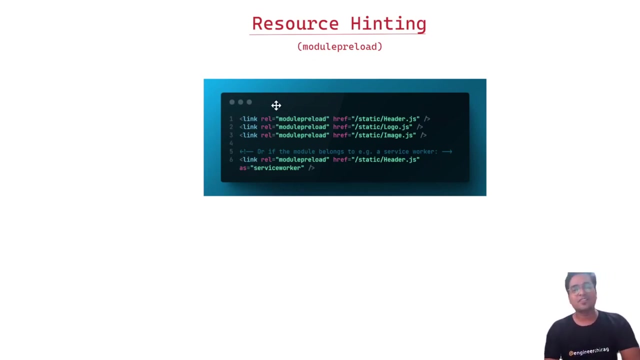 now there is another very interesting thing, which is resource hinding for the module preload, as as now, in the browser, you can actually load the- you can say- modules all together, you can import those modules, you can leverage those module. what we can do, we can provide this relation, uh, this. 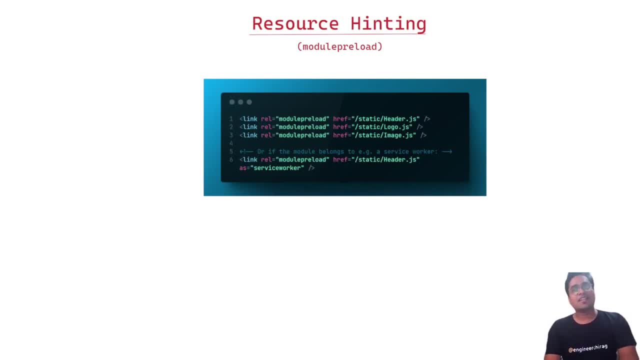 hint. basically, we say that this is a module preload and, in this particular case, what it is going to do, it is going to basically load your es module and it is going to download cache and it is going to compile your js module code as soon as possible. this, this is way good example which you can leverage along with. 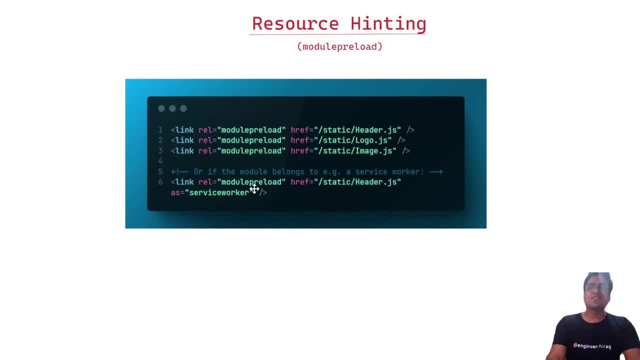 that you can leverage this one more for one more thing, which is if any resource, any module which is required within, from your service worker as well. basically, you can leverage this so you can give a hint which says that i, i, this is something which is going to be leveraged as a service worker. 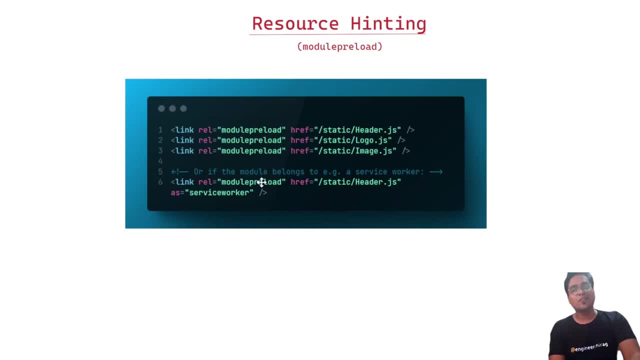 just give a hint as a service worker and you can load this module as well. what it will do again, just note it down, what it is going to do: it is going to download, it is going to cache it and it is going to compile it so that it is available for consumption then in there itself. so this is 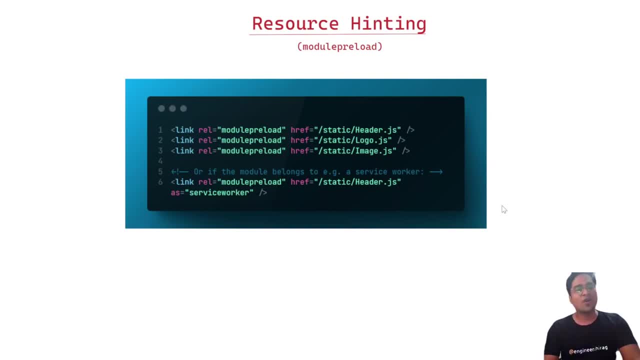 again very powerful. if you are using the es modules, just go and try it out. these are couple of the resource hint. if you haven't tried in past, i will request you just go and try it out and you will see the performance impact in your production application. and if you are in an interview, if you 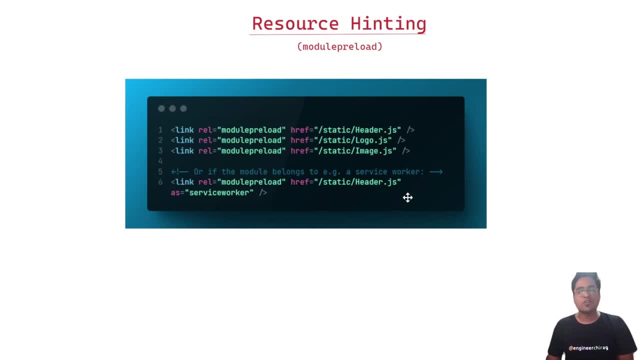 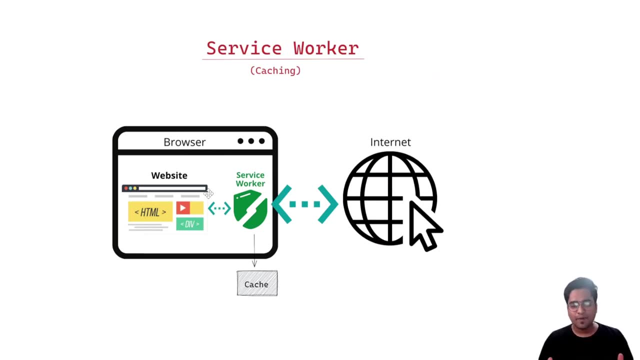 are talking about this and you can detail it out. trust me, it is going to impact you a lot of things and it is going to make a very positive impact. service worker- service workers are way powerful in order to basically provide you a caching strategy or making offline applications. 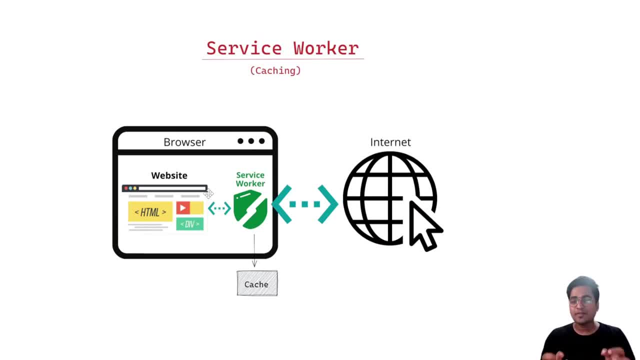 right. so in that particular case, there are so many cool things which are provided by service worker, but before we jump into what are the things which pro which are provided, let's let's try to understand what are these. service worker are. service workers are something like proxy server. 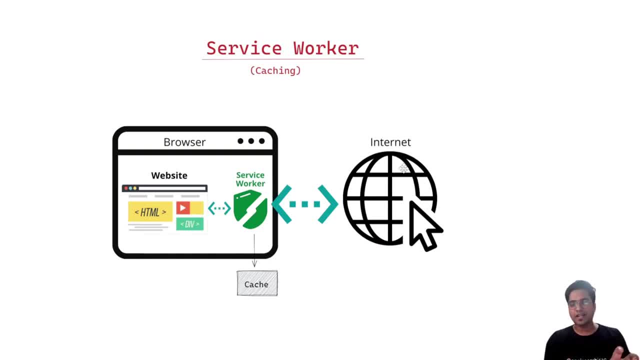 which sits between your browser and your server and it is going to make a very positive impact on your service worker and it is going to make a very positive impact on your service worker. so, in that particular case, any request which goes to the internet via the network, those are 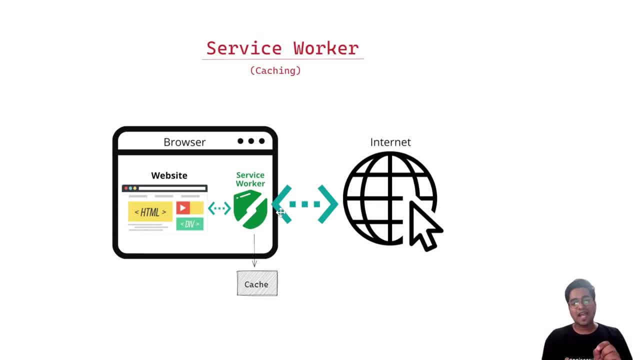 basically intercepted by service worker. now it has a lot of interesting thing: using service worker, you can interact with your cache, you can interact with your index db and lot more. there are certain limitations in terms of what you can't do, in terms of the dom manipulation and sort of thing, which. 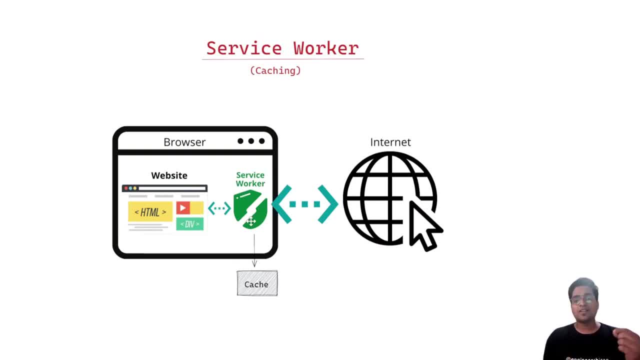 can't be done via service worker. but again, apart from that it it actually holds a very good interceptor for any request that goes out basically on the internet world. now try to understand how the server worker are related our day to day life. i personally feel service worker 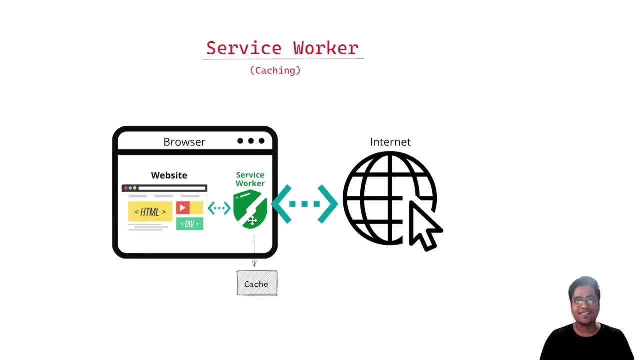 is quite similar to our mothers. so how? it's very interesting, like how a service worker can be related to our mother. so most of the time, what happens? we can offload our work to mom. just remind her mom, i, i have to basically wake up at this particular time. can you take care of the things? 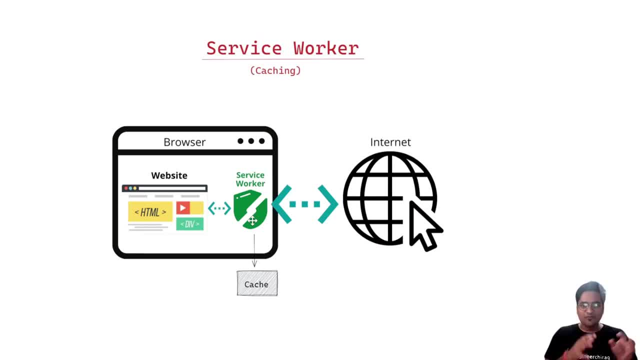 can you remind me at that particular time? now your mom will work in the background. she will make a level, everything in order to make you aware or make you awake of certain things. so she is there to basically do a lot of background job for you. now there are a lot of things she can actually do. 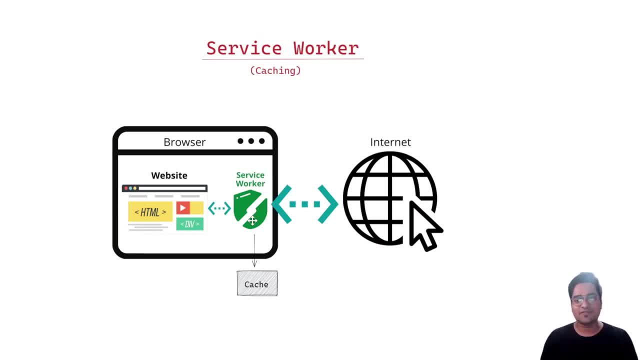 she can actually provide you functionalities like push notification, which is like someone was seeking for you, right, and your friend was seeking for you anything that you wanted to be aware of happening nearby. your mother can give you a push notification. actually, she can let you aware of the things which are happening around, right? so those are the 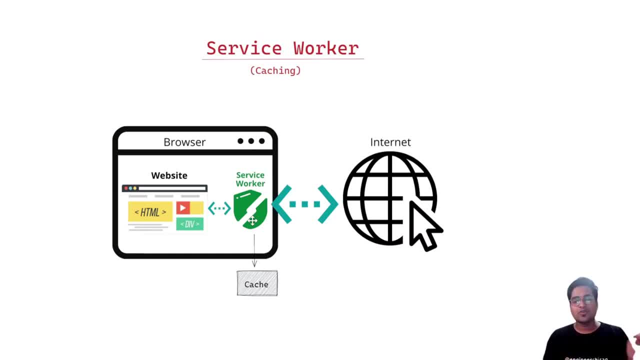 cool thing. and again, in terms of the caching, just let your mother know you like certain foods. she will make sure she will have a lot of plethora of those things in inside the house so that next time you are looking for a similar kind of uh food or similar kind of taste, you don't have to look out. 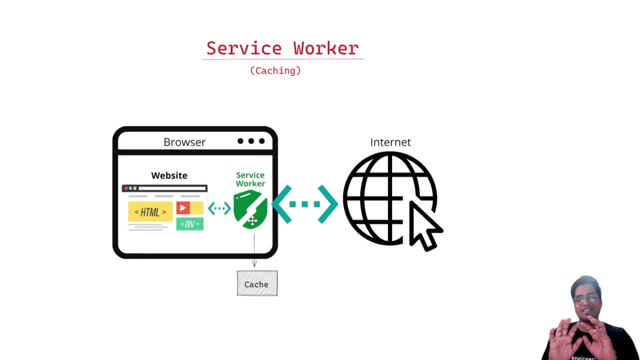 for that. she will make you make it, cook it, and she will basically add a cache and store it in the house itself, right? so then, next time when you're looking for it, she will quickly provide you the flavor, the food, the taste and and the best experience, right? so it's? that's why i relate the 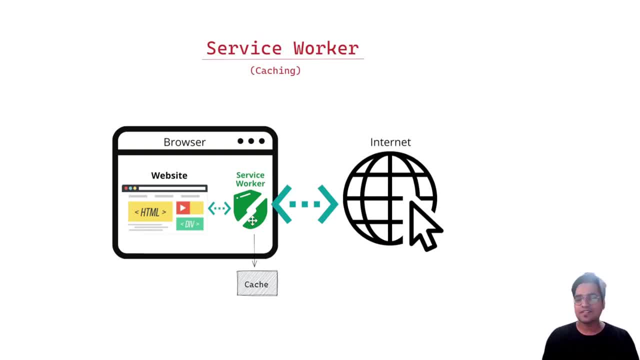 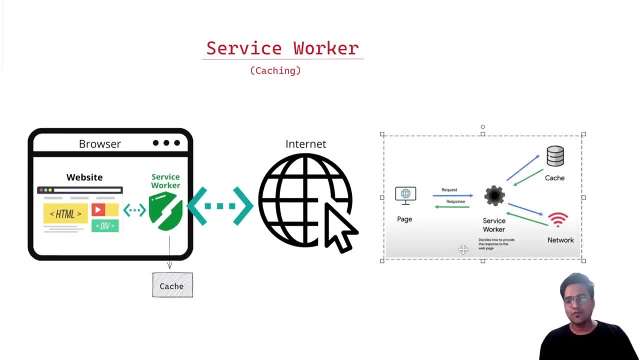 service worker, quite with the mom, which helps with lot of interesting thing. now try to understand in a bigger, in a different picture altogether, if that is helpful. so basically we can also try to visualize this in this form. you have a page, you have a caching layer, you have a network and on. 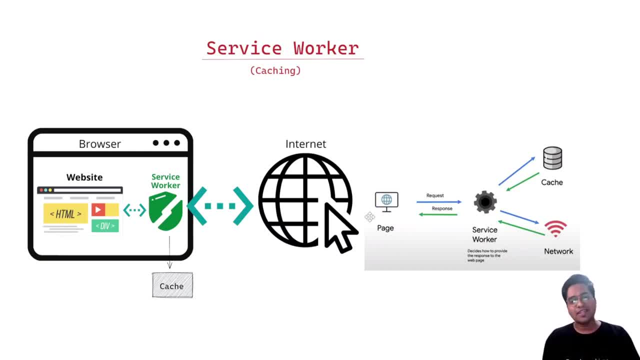 on the mid of that, your service worker is sitting. what it meant by any request: where your page wanted. first it will go to the service worker. now, service worker, you can write your strategies. either it should look from the cache or, basically, it should go to the network layer in order to fetch. 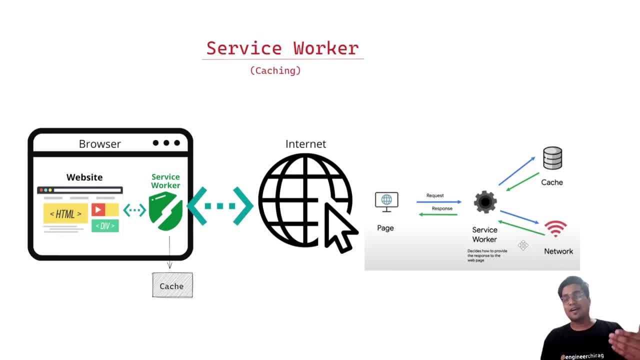 it now you can also make it more optimized and more advanced. in a sense you can say you can write a logic. if you don't have internet connectivity. you try playing with the cache, you try to play and keep your data in the index db maybe, or any storage on the browser, and once the internet is, 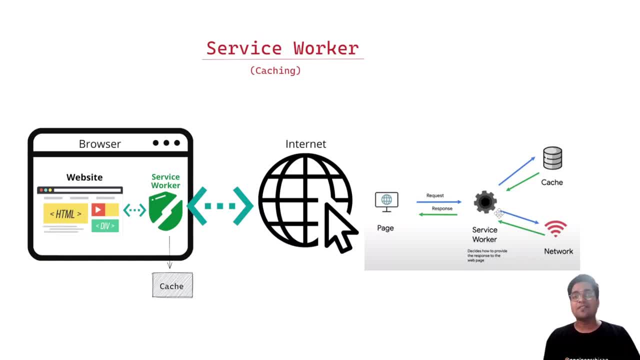 back. basically, you do all those operation on the network so that, even without an internet, you can have a good experience to your end customers right. so this is how all the offline things that you might have seen, like google doc or anything which is working on the browser in offline mode, to 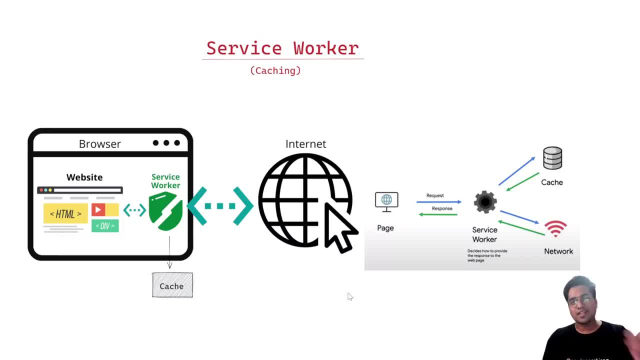 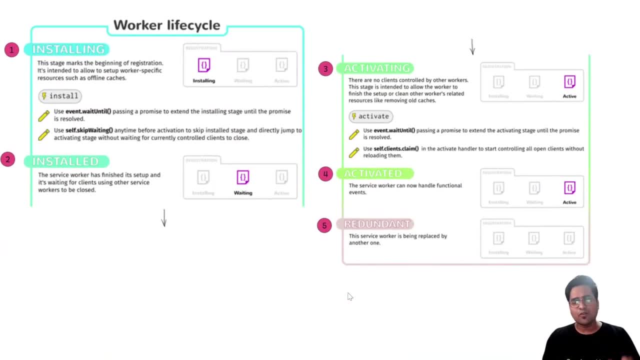 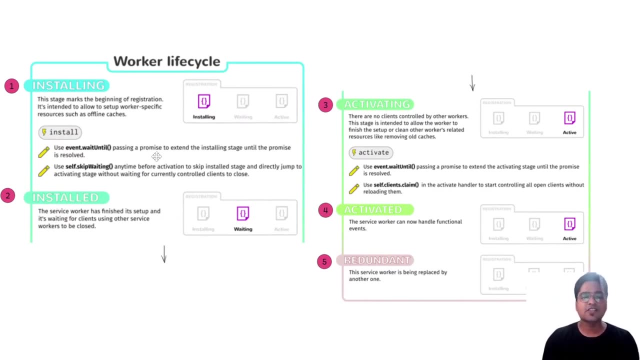 provide you a better experience. those are basically using the service worker and definitely, uh, that also helps you to build the pwa progressive web app. so now try to understand what. what are the different phases of the life cycle of the service worker where you can actually fit your lot of use cases. so first thing is installing, installing right. so 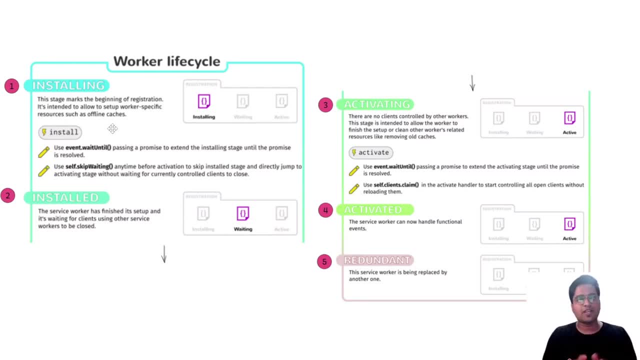 there is a file. basically there is a way. basically we will be talking about the code as well. you can basically write your code, you can initiate your service worker and it will install in your browser, basically, uh, and the service worker instance which is created. it can be shared between the multiple. 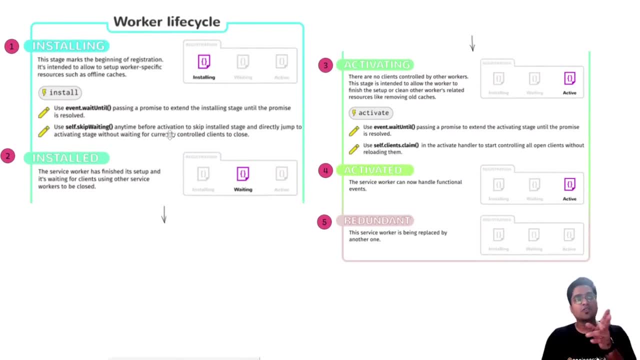 occurrences in your uh tab also. say, suppose you have two tabs open for the same domain or the sub domain and you wanted to have a communication between both of them. you can basically leverage that as well. so there are strategies and ways. we will be talking about that as well. so once first, 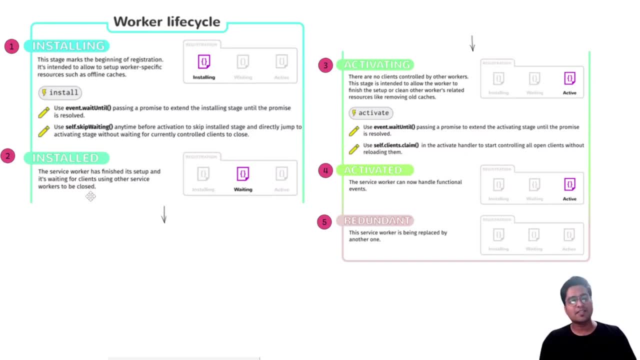 it is going to install, uh, the service worker. the second one is installed in that particular case. what you can do? uh, it will basically wait for other clients who were using the previous set of service workers, sort of, in order to get it closed so that you can have a fresh installment. 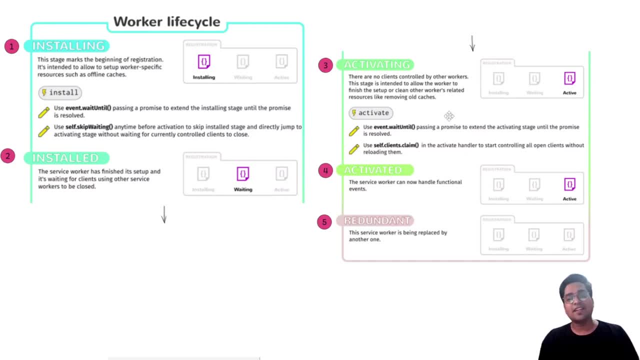 of the new service workers instance. now it is activating it. over here you can take certain decision in order to clean up some cache, the previous cache, or you wanted to do some operation on the cache. once it is activated, now it is a ready to listen all the events that can happen. 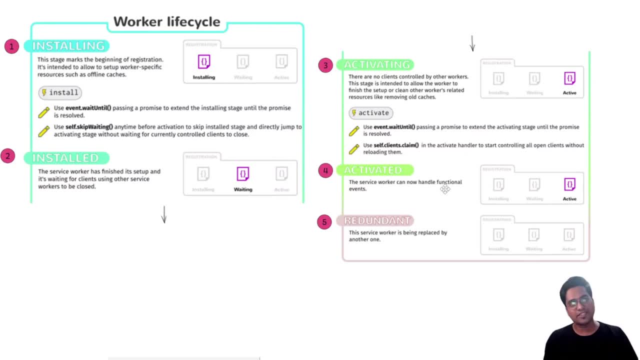 the, which you can basically transmit via the service worker. all these things you can do- and definitely this is redundant- if your service worker is replaced by another service worker. this is basically being called: you can take certain decision in order to do something up or something you wanted to make sure. now where the service worker basically resides in your browser, where 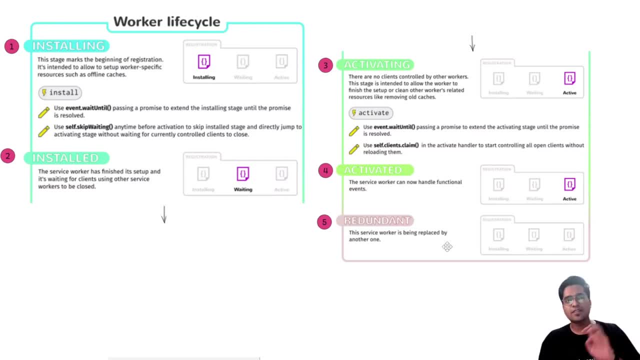 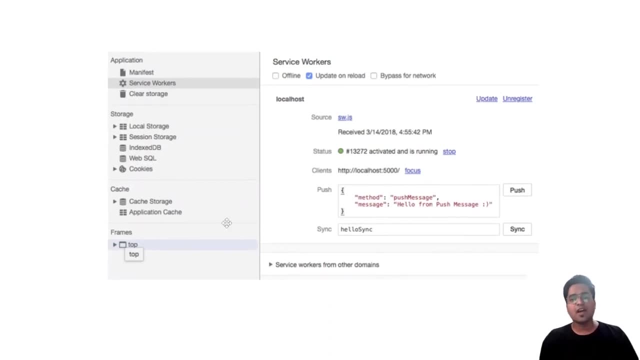 you can see and how you can basically debug certain things, then we will jump into the code part of that as well. okay, over here let's, let's have a look up. so in your browser, uh, in your dev tool, basically we have application. you can go into the application, you can try it out. if you haven't seen the service worker. 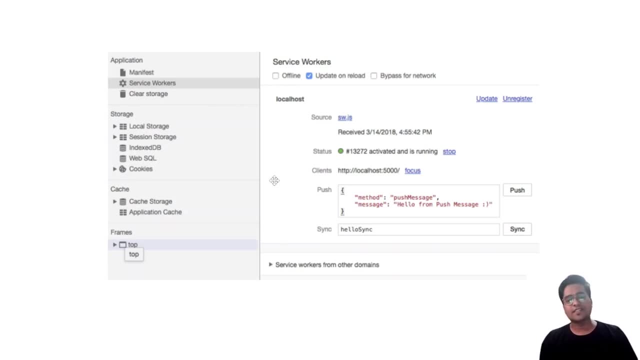 go and basically tab into the service worker tab. you will see the service worker over here and if this worker is activated, you can see the service worker id and if, in which state it is basically involved, when basically it was set up right, you will see all the events. you can actually do a. 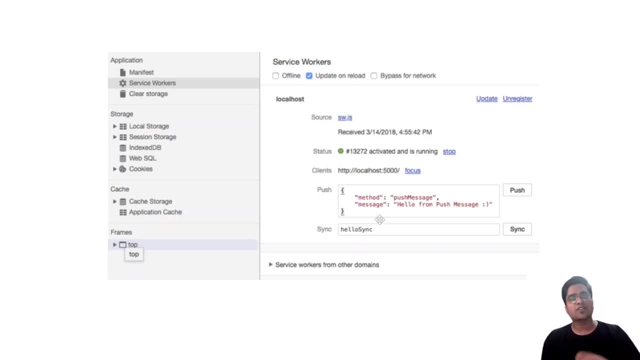 testing. you can try pushing, uh, some operation over here. you can try to push something over here, or you can try to sync from some something over here. you can update and register. you can play around. just give a try, play around that, but again, playing around that, first you need to basically. 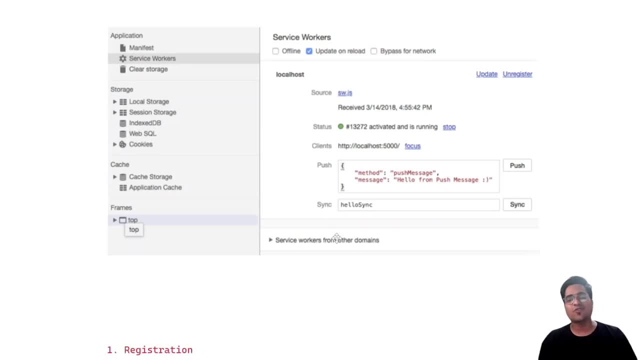 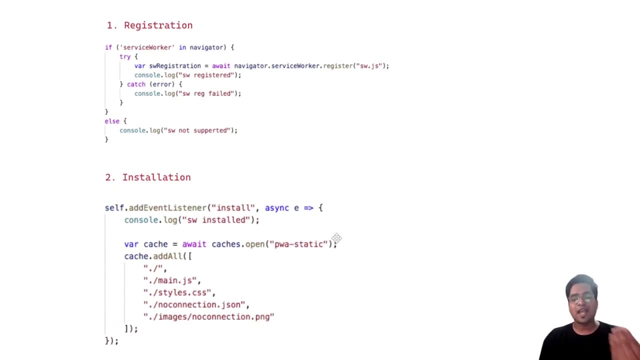 understand how these different stages are and how you can leverage. so we'll go through quickly some glimpses and i will also telling about. you don't have to actually learn all of these. they are small uh libraries and small tricks, basically will help you to set up your service worker. and it is going. 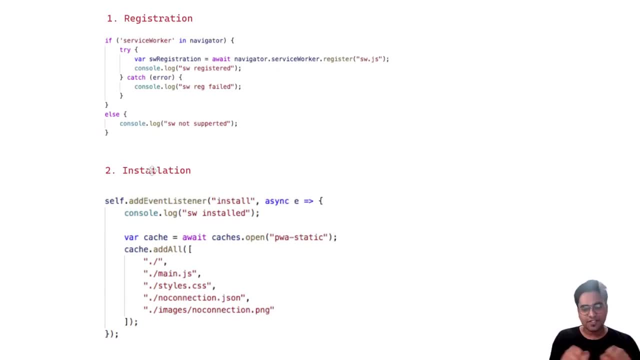 to boost your experience. so let's talk about that basically. first step is, in order to register, you have to do a small thing. you have to basically check if the service worker is available inside the service worker and if it is not available, basically you can actually set up. if it is not, 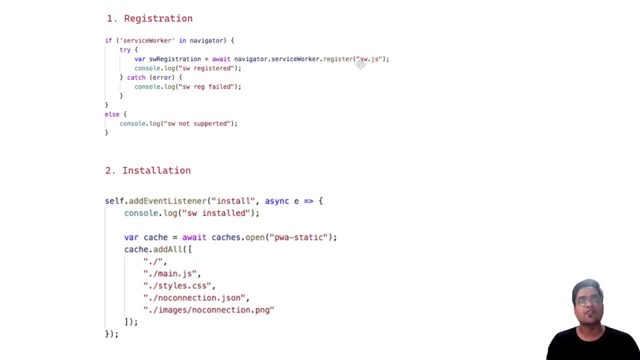 available. you can't do anything if it is available. what you have to do is just a simple thing: using service worker, you have to register. this is the file. basically, this is where your code will go for the service worker right now. what are the other things? there are simple steps that you can. 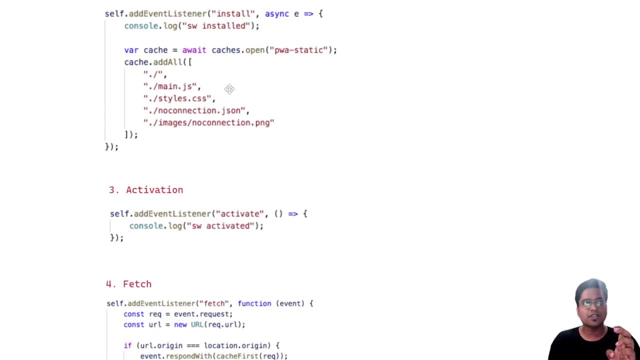 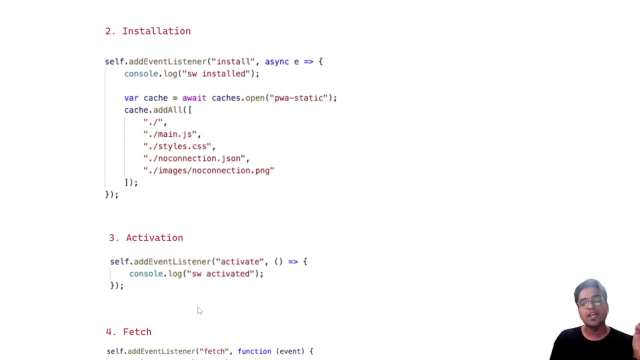 basically write in your service worker file. what are those? you can write the first installation step, which is this. you can write your activation and you can define what will happen in case of the fetch, if something is basically looked after in the installation. you can define how basically you wanted to respond from your service worker, right? 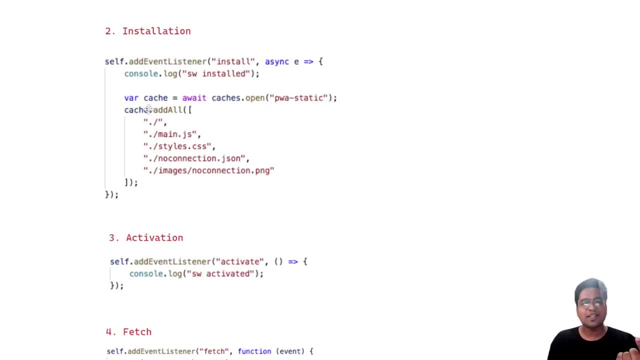 from the installation, you can see what. what is basically we are doing. we are basically trying to open a cache with certain name. we wanted to add some files to that particular cache and we wanted to make this available. when a person is basically looking for, uh, the fetch calls right in all those. 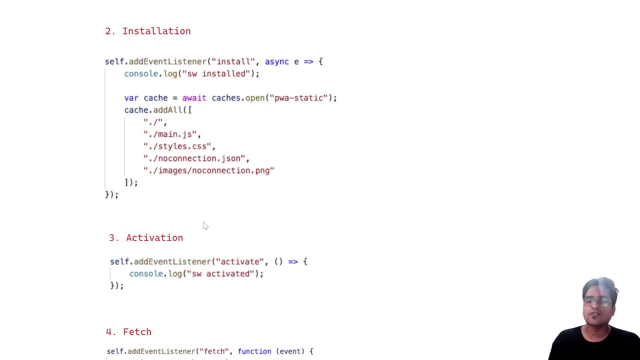 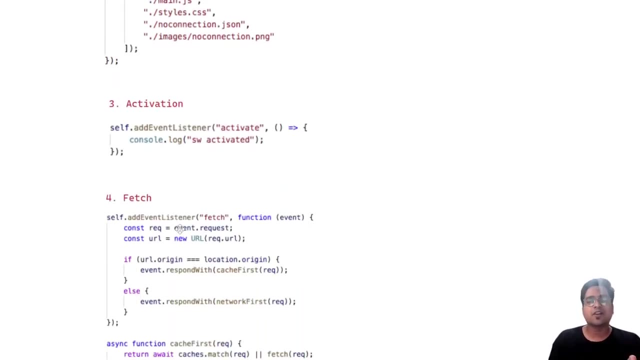 cases you can define. you wanted to basically fetch these files from the cache only or cache first approach. there are different approach that that we can talk about right. second is, if it is activated, you can start listening a lot of the event now. the the third important is the third important event. 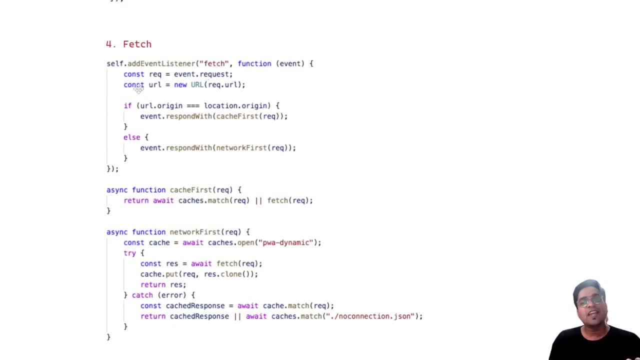 is your fetch right in this particular case, what we are doing? you can basically look for the request. you can basically fetch for the which url this request is being made. you can get to know the, you can check the origin and everything inside your logic. now, based on that, you can decide you. 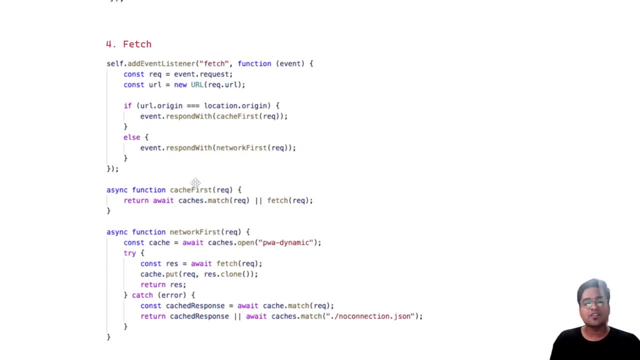 wanted to do a cache first or a network first approach. based on that, there are a lot of strategies which you can define. if it is a cache first, you can define. you wanted to look from the cache, or you wanted to make a network call first. you wanted to basically look for the. 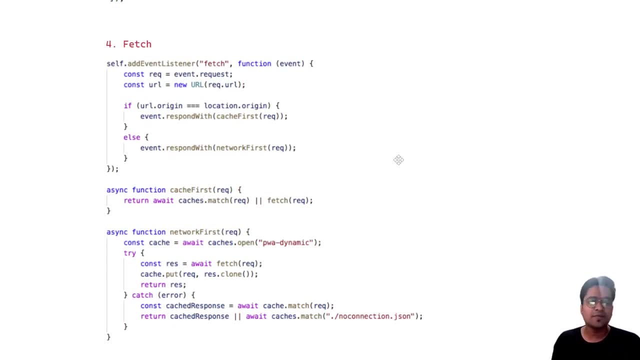 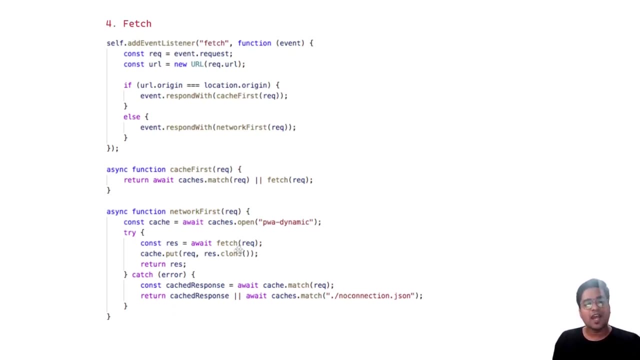 cache. if it is not available, then probably you want it to go and make a network call, right in case of network. first you can see, uh, in this particular case, what is being made. uh, we are fetching from the network and we are basically putting that particular data into the 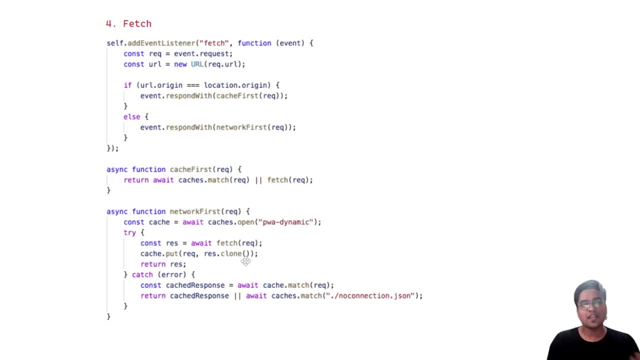 cache so that if the next time someone is looking for the cache, first approach in that particular case, our cache is already having those data right. so you can do lot more interesting thing and we can also see if they were looking for the data which we were looking for, which we wanted to. 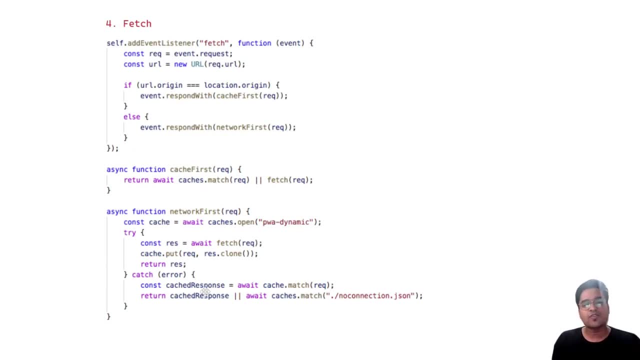 fetch from the cache at that particular point. this is a really useful and you can understand, is some error. basically, in order to fetch the network call, you can actually land back into the cache strategy also. right, so many things can be done using the service worker and these events that we have talked about I have just given 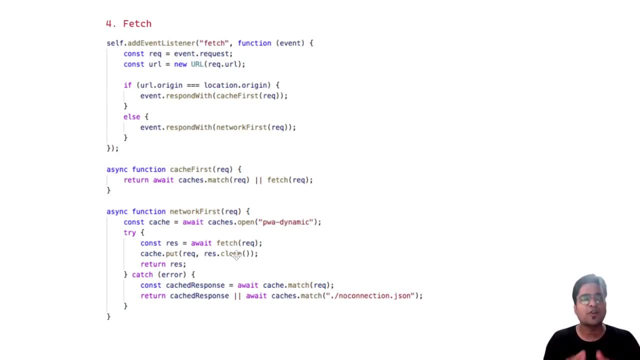 you a glimpses so that you can basically go and try it out, because this is very, very cool. if you haven't actually looked into this, so trust me, you are a step behind and you have to give a look into this now. say suppose you have to build. 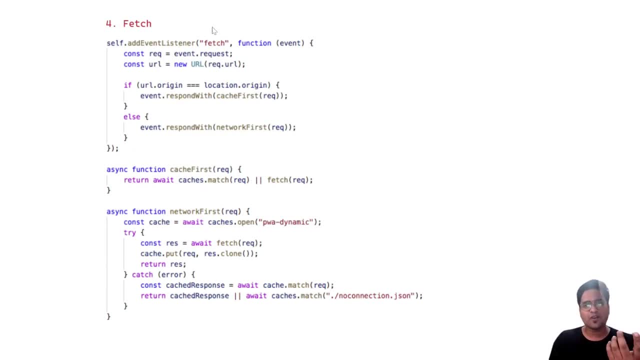 a lot of complex use cases. in that particular case you don't want to write all of these method and all of your implementation. can be there some way to write. thus you can say standard code or good quality code with a very less things that you have to peep into right. yes, there is something called workbox. 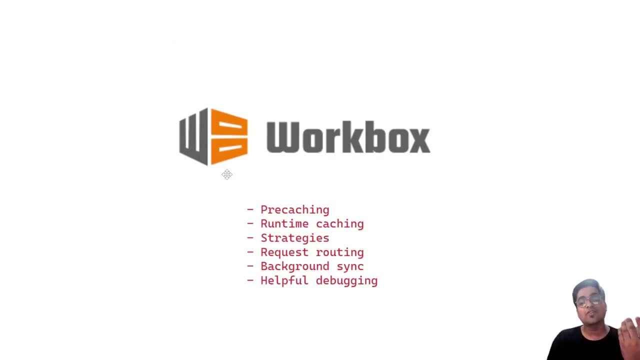 which gives you out-of-box lot of capability and it gives you things to enrich lot of things. so, taking example, prefetching is something that you can do using workbox. you can actually define some caches. on the runtime strategy, you can actually define the strategies. you can build your own strategies, strategies like I wanted. 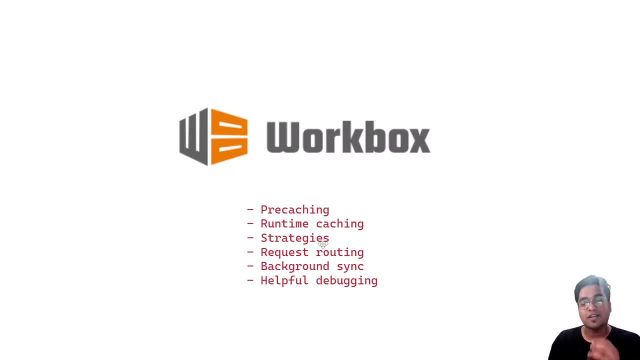 to make a cache only, or cache first network, or first network only. right, you can define cache and network. right. first, try to look from the cache. if it is not available, make a network call. right, you can define a routing so the request which is coming from this particular path. you wanted to basically make a 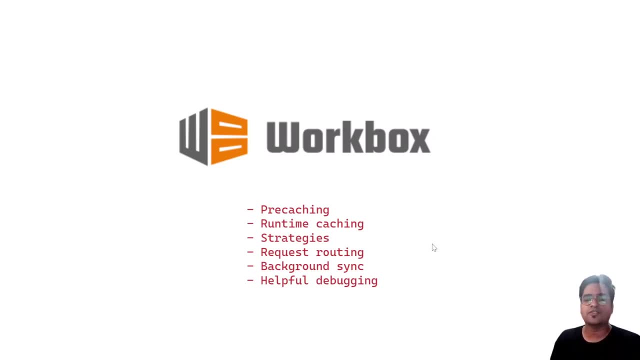 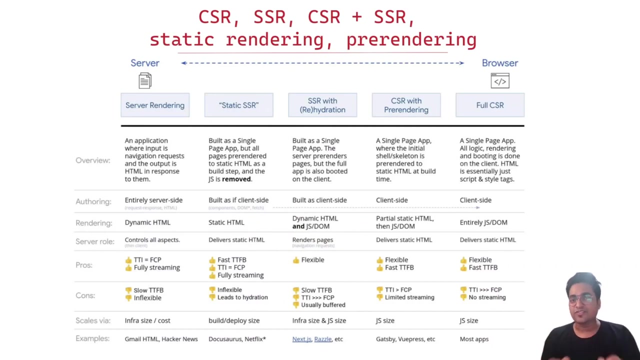 request to a different server or different. you can say web all together, the server all together. right, you can basically define very easily the background sync processes- right, you can actually help lot of like good debugging capabilities you will get with the workbox. so if you haven't tried, go and try it out. we are going to talk about 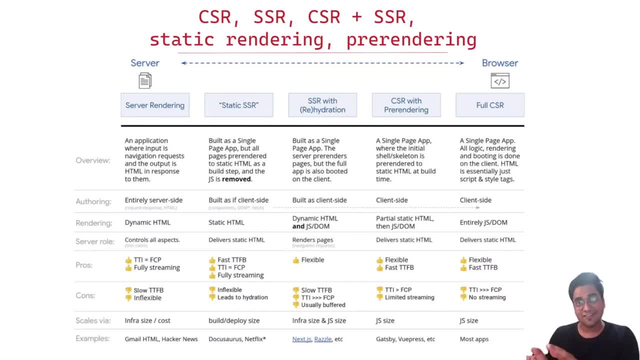 very interesting concept, which is client-side rendering, server-side rendering, combination of client-side rendering in server-side rendering, static rendering and pre-rendering. hold with me this is going to make basically change the way you think about how to create a web app right now, before we jump. 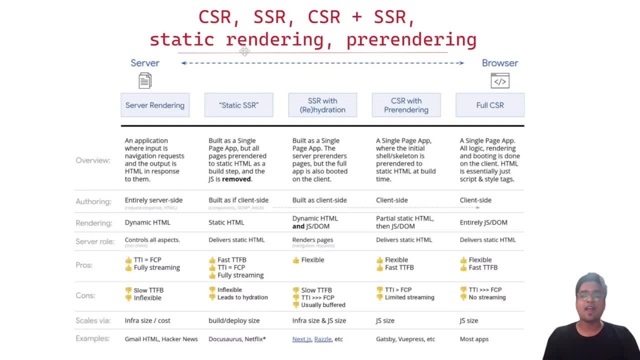 into what is this client-side, server-side and basically understanding the pre-rendering and the static rendering. let's try to understand very basic and the fundamental things, which is going to help you in order to understand this important thing. so, first thing first, what is the server-side? so 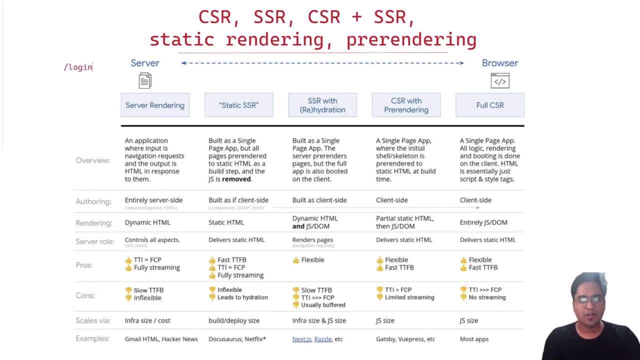 consider example you are requesting, for I wanted a login page or I want a dashboard. this is a request which goes from a browser to the server. now I'm saying it turns out to be a server and a server-side message, and the server-side message is a safe account. so we'll just go and I'll just do that in just a couple. 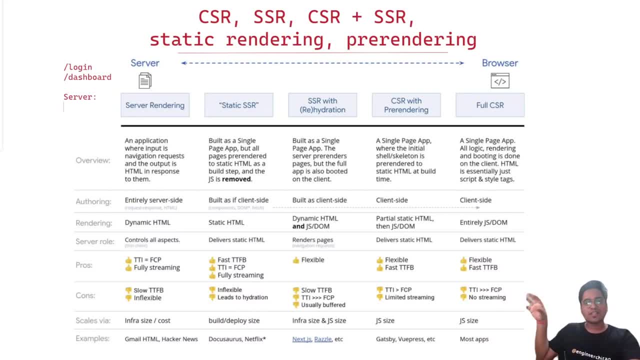 of minutes. so now, if your server basically does some certain things, what it does, it basically processed the request for this particular route, which is slash login in slash dashboard. it generates the HTML, it generates the relevant JavaScript and everything and it ships right. so your server got a. 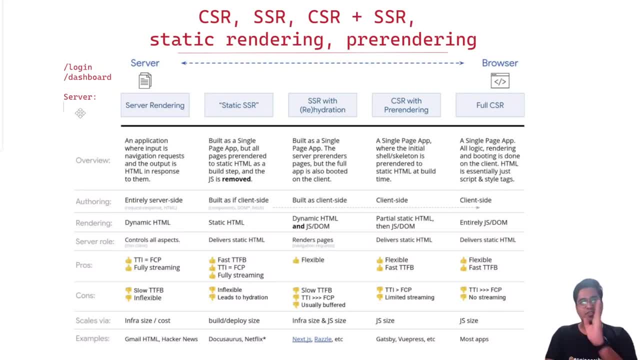 responsibility to generate and shift for each and every route where the browser is a decide what need to be rendered and it gives you the final HTML that need to be rendered. now coming to the second part, which is our client-side rendering. in this particular case, what your server gives, your server gives the J's. 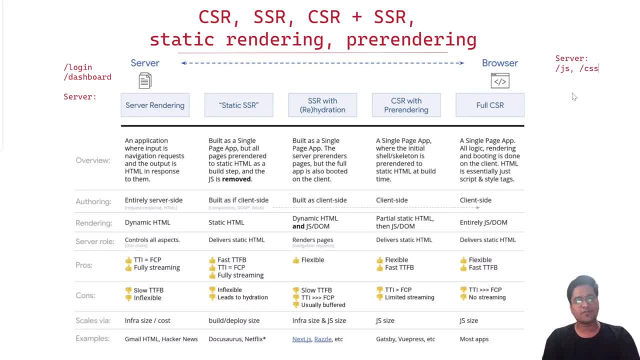 respective. you can say CSS and all sort of thing. now your browser does certain things. what it does browser start understanding the routing. so, say suppose, is the similar example: someone was on the dashboard, the home page slash. now he wanted to go into the login now in order to get that data or the HTML for slash. 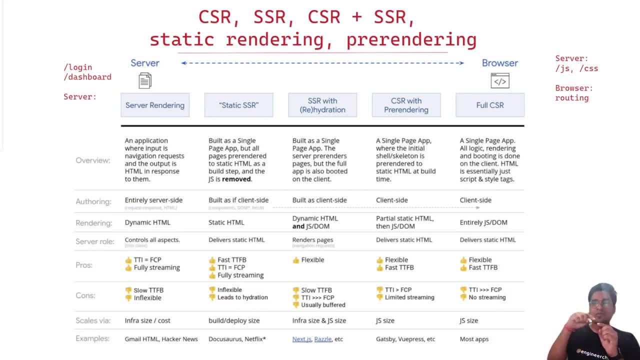 login. your browser is not going to make a request to the server. your browser is capable enough to understand. there is something called slash login and I should basically get the data from the local chunks all together, although while rendering it it require any extra JavaScript or chunk it. 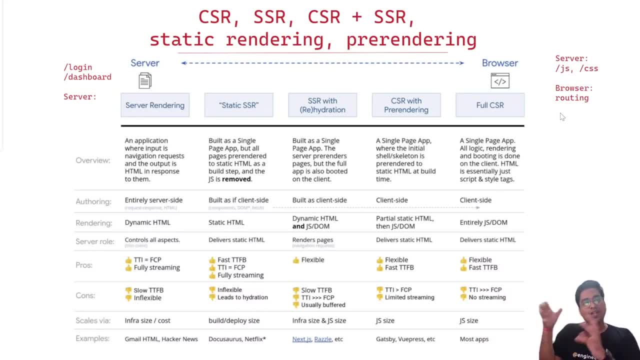 can be rendered in the same way. if you want to get the data from the local chunks all together, although while rendering it it require any extra javascript or chunk, it can go to the server. that is different thing. but for your routing purpose, your landing page, which is required in order to do the routing, you don't need any. 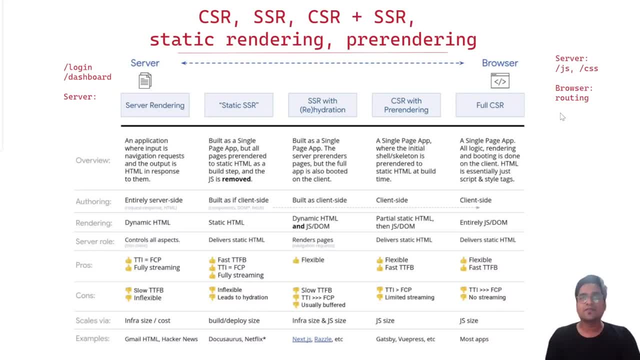 server in order to tell you for this particular route, you need different, different. they say, no, everything is managed on the client. okay, now, what are these things which are in between? let's try to understand and will understand, its benefit and which one to use and when to use what? what? all you can do? 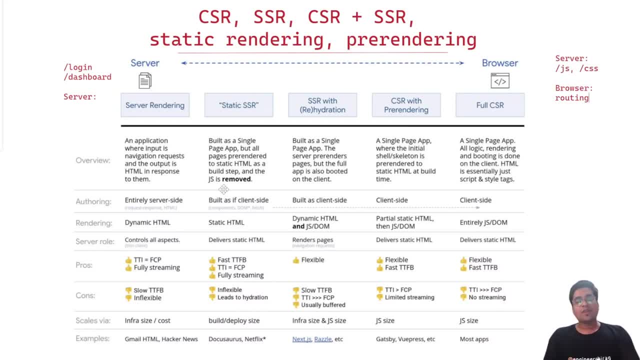 static SSR. what it meant by when, basically, you are building your application, when you are writing something like npm, run, build or doing the similar kind thing on the server. what it does say: suppose you are creating some blog and you know you have thousands, or you see, suppose hundred. 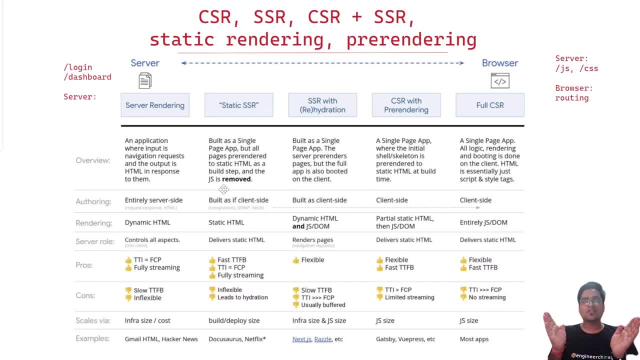 pages with a static data. what you can do: you can build those hundred web pages all together and you can put that web pages directly on your browser so that anytime the page is requested, you basically go and serve that static web page directly from the server. okay, this is cool, right, because there is no dynamic thing, no API request. we can. 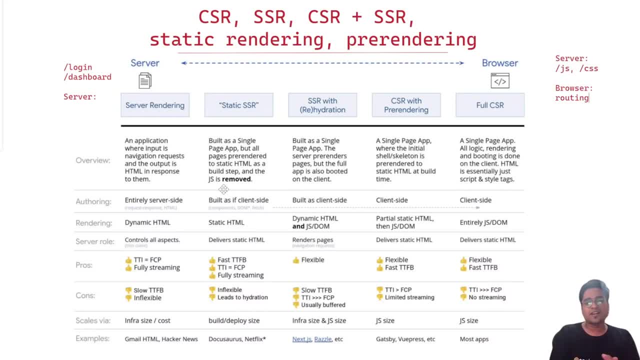 avoid a lot of thing and you can directly serve the already pre generated web page right. the second thing, which is again very popular: people call it server site rendering, with dehydration, what it meant by you might have used- react or angular. by using the server site rendering what it does, it creates a web. 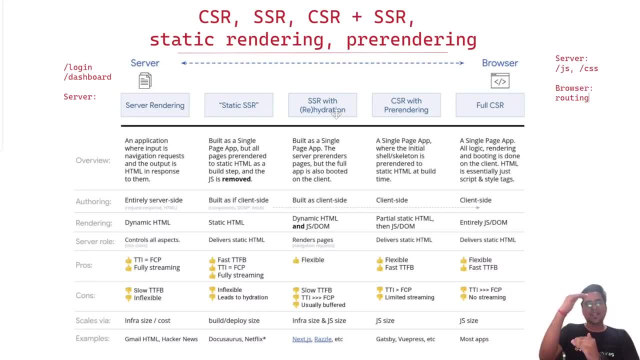 page. it's basically generate your HTML, but that HTML needs some events to be there, right? say suppose you have a form in form, you wanted to add some event handling on change of this, on blur of that, on different. different events are there. you want those events to also work, but on the server, your server don't. 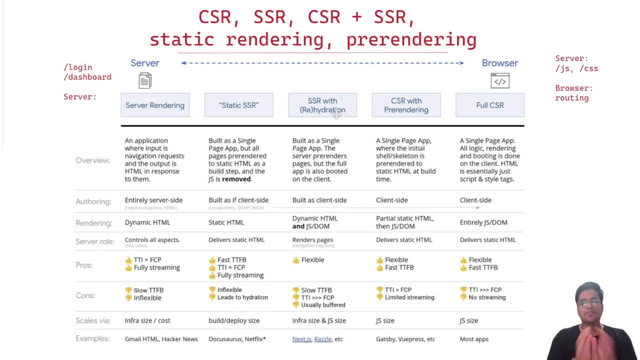 understand these event, what it will do. it will generate this HTML and it will give to the browser. now, browser have a responsibility to rehydrate. it rehydrate in essence. you have given me HTML and I know the events which need to be binded. I will bind these event so that your, your web page, become interactive. 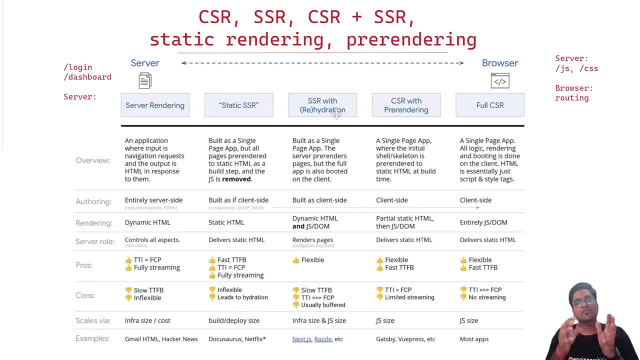 now before hydration. your web page is not interactive, so this is basically called your server site rendering with the rehydration. now there is another concept which is called client-side rendering with the pre-hire, pre rendering. what does it mean by this is very interesting concept, what it says. 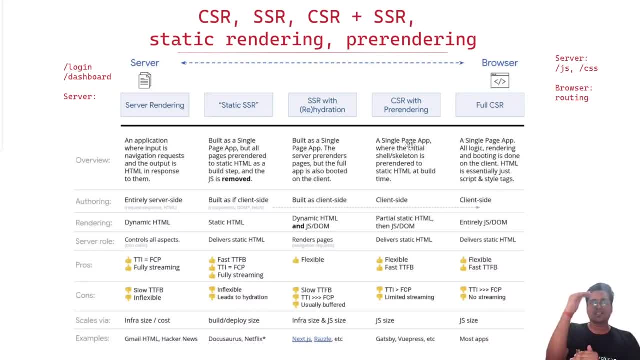 that I am NOT going to basically render everything on the server. what I am going to do, I am going to just give you a shell and it will have the basic HTML and things rendered. the rest of the things client is going to take care of in order to render. but over here, any dependency which you have in terms of 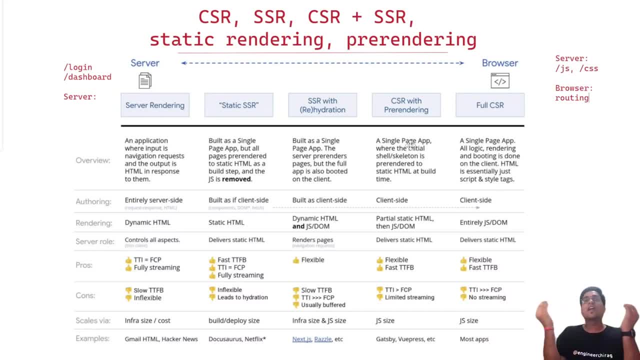 the JS in terms of the CSS or anything which need to be loaded at a faster rate. I will make sure I get those dependency and inject those dependency in your web page itself so that when you are you doing a client-side rendering on the client, on the browser, you don't have to look for those dependencies. those can be. 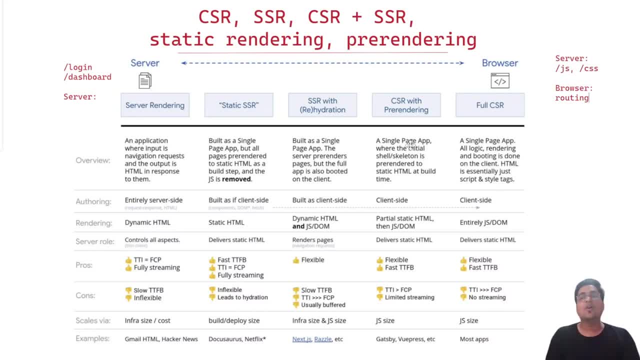 made advanced right. this is. this is very cool. now you will find lot of the application, old application that was built on the hundred percent server-side rendering. you will find a lot of application which is like on the pure, you can say, client-side rendering and there are a lot of application which are 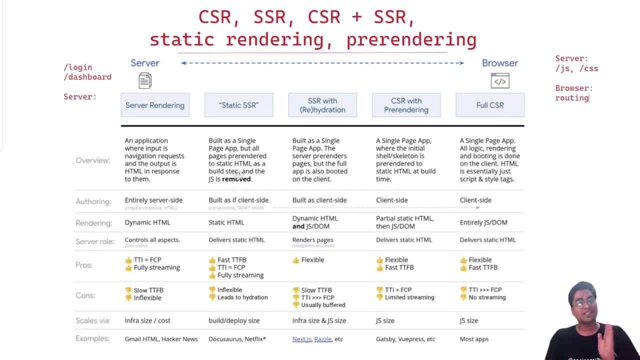 blog related, which are built on the server side: the static server-side rendering and using the dehydration. so there are two very, very popular these days these mechanism which people are using. one is client-side rendering with the pre-rendering mechanism and the server-side rendering with the 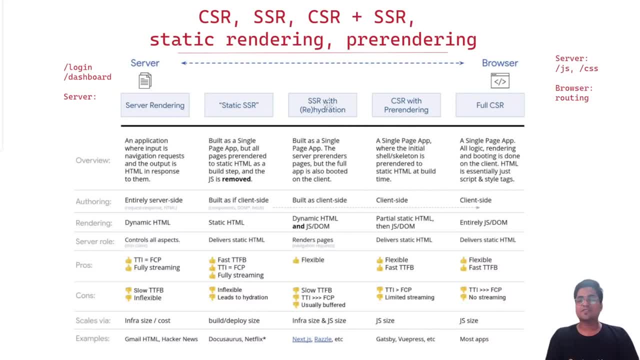 rehydration mechanism. right, these are two ways which is very, very, very popular. let's try to understand couple of more important things over here. what are those? first, let's try to see who is basically using it. in this particular case, you can see the Gmail was using is very actively, even you see the static one, the Netflix. 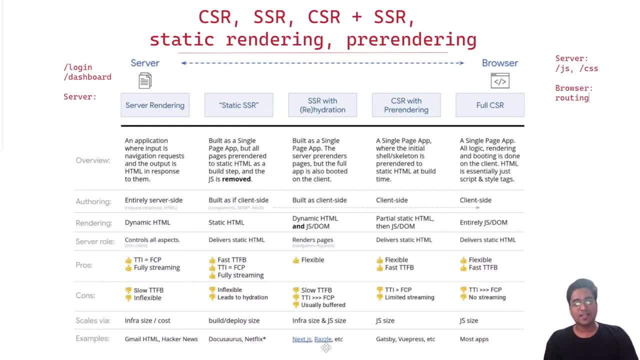 was using for a lot of the static pages. the server-side rendering with the rehydration, you can say next, just is built and on the same concept and even the razor is based on the same concept. so client-side rendering with the pre you can say pre-rendering. this is used by Gatsby and the view press and the. 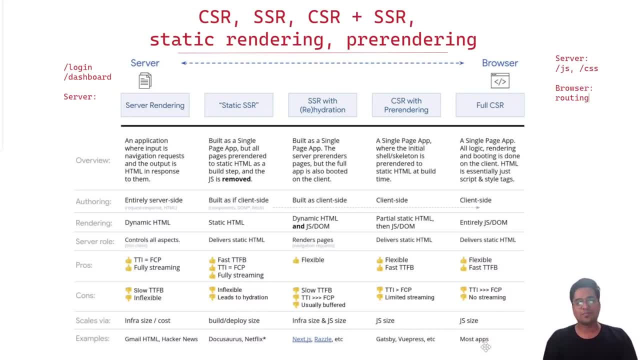 mindful. you can see the client-side sourcing is used by most of the application. by so, although there are a lot of strategies in terms of the gmail is also trying to use, you can say client-side works and entering T like these are the different applications or the companies which keep 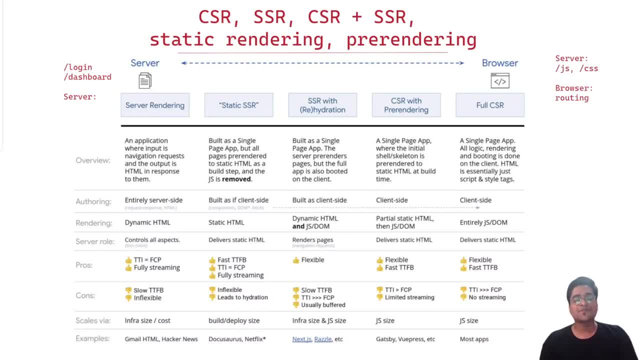 on experimenting and trying between the law between now. they're a couple of thing that we have to understand. what is the cost of these different mechanisms, like the first one, which is server-side rendering? it is going to cost you a lot in terms of use of in for us. 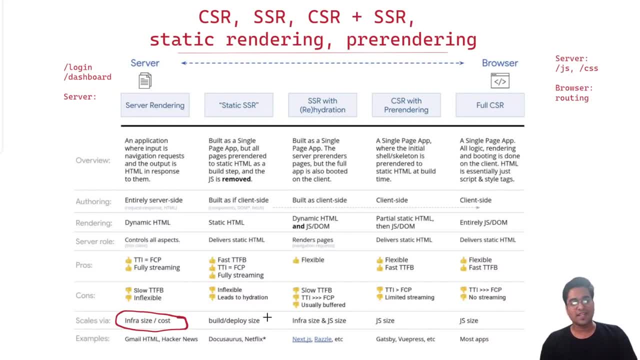 reason, every request need to be handled from the server. second, this is going to cost you in terms of when you are building and you have to keep all those asset on your browser. your storage is basically going to be very costly in in terms of server side rendering. with the rehydration, your 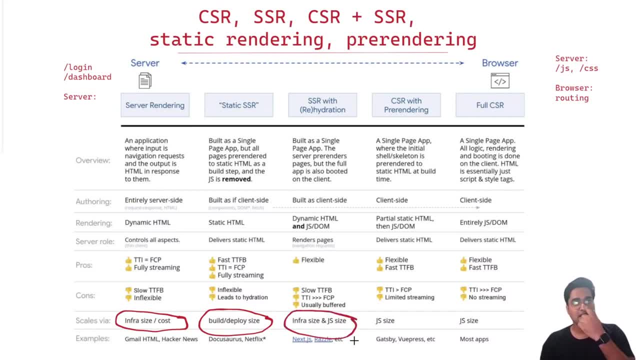 infra cost is going to be costly and you have to basically think about the js, uh, js size as well. right, because infra cost, because, uh, most of the request basically, is going to be on the server and that need to be rehydrated on the on the client side. right, this is going to cost you. 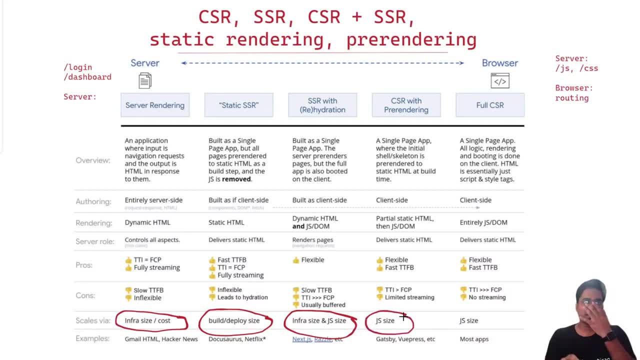 javascript, because you just get the cell and rest. everything is basically going to be costly operation in terms of the javascript need to be loaded and a lot more. this is 100 percent. you can say javascript, because the server takes care of nothing. it will just give you the html, uh, html. 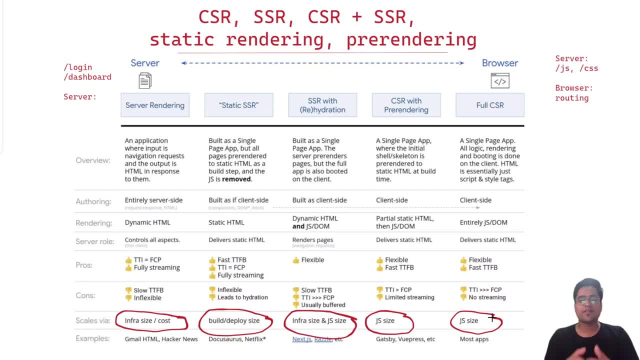 and from there the parsing, loading, rendering, getting those js's and running on the web page. everything is taken on the client now along with that. this is very interesting, which is time to interactivity is as close your. you can say first, uh contentful, uh, paint, although this is very, very 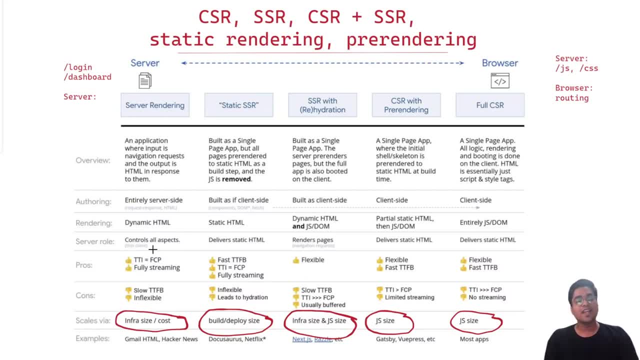 reasonable, recommended. if you have your time to interactivity and your first contentful paint very close, this is very, very good, right, it is almost equivalent and in this particular case you can see, this is also equivalent. but your uh tt fb is very fast in this particular case, right. 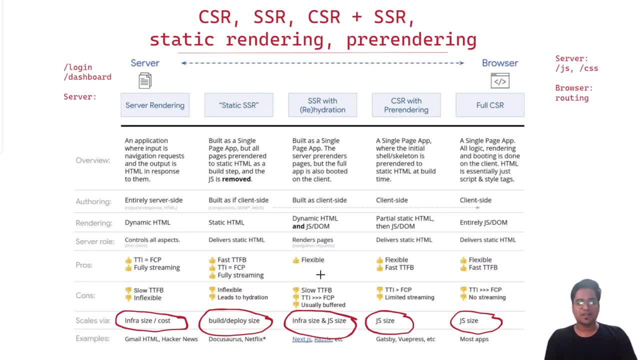 so time to get your first bite, which is- which is, again, this is a flexible approach. you can do a lot of thing in terms of the ssr with the hydration. this is again doing a csr with the pre-rendering is something which you can leverage. you can do a lot of optimization over here, so just go through. 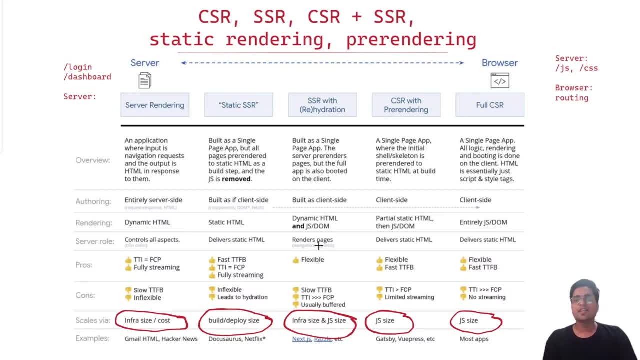 this and try out these different thing. you will definitely get the best out of it. and you will definitely get the best out of it. and you will definitely get the best out of it. and you will definitely find, depending on your use cases, you are going to leverage a lot of stuff over here. 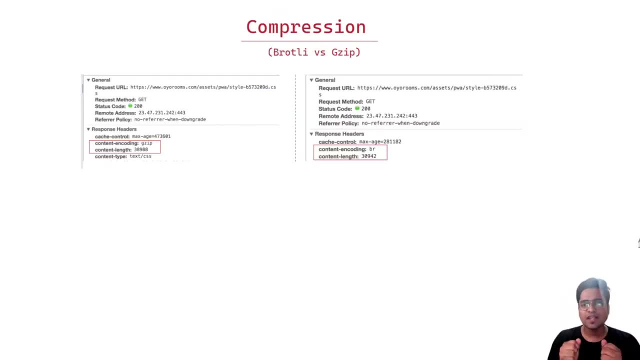 so don't forget to try it out and keep watching compression. this is another very small but very powerful technique, what it meant by. so consider example you- i think most of folks have already used a foam matrix mattress. basically, in that particular case, how those are shipped, those are. 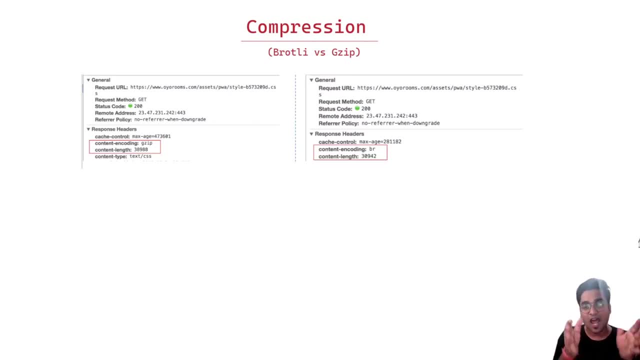 rolled back and those are delivered to your home, but how those small wrapping basically converts into a actual mattress. what you have to do, you have to just cut the cover. it will basically roll up and roll out basically and you will see after certain time, after getting the air available, it 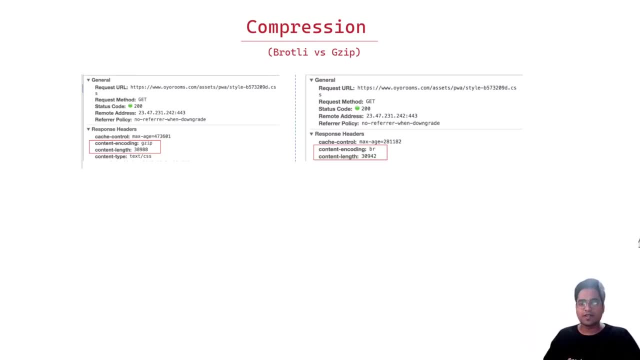 will actually block into the normal size of your mattress. or you might have seen some crystals basically in those crystals are small, small thing you have to put into the water and it actually glows up to a bigger size and those are very eye-catching sort of thing, right? 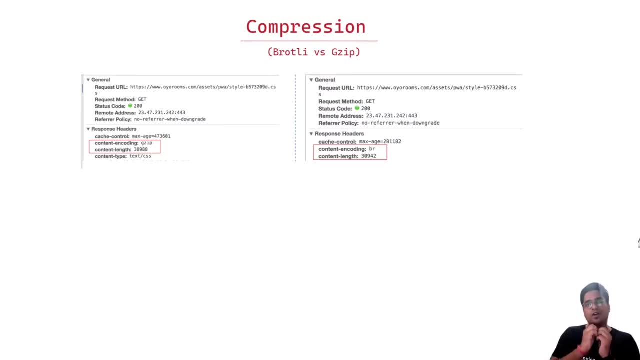 so we have seen a lot of these things, which are basically very helpful in order to transfer from one place to the other place. else, basically, it will. it is going to occupy a lot of the space, right? similar kind of thing happens with your assets as well. when we say assets, your javascript. 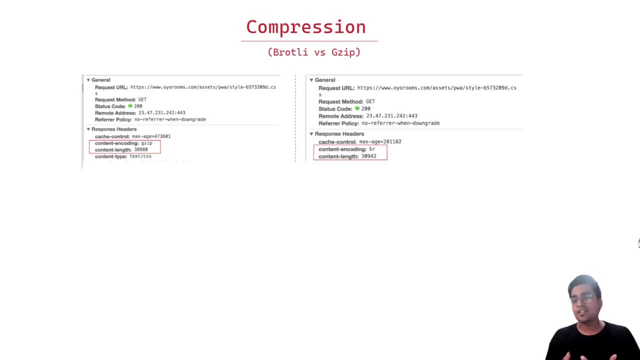 css, the images and whatnot. so consider, instead of shipping your 300, 400 kbs of files in through the network, what if i say i'm going to compress it using some encoding and basically i browser knows how to decode it. so in our case, suppose the water was one of the medium in order to decode. or, say, suppose the air was another medium. 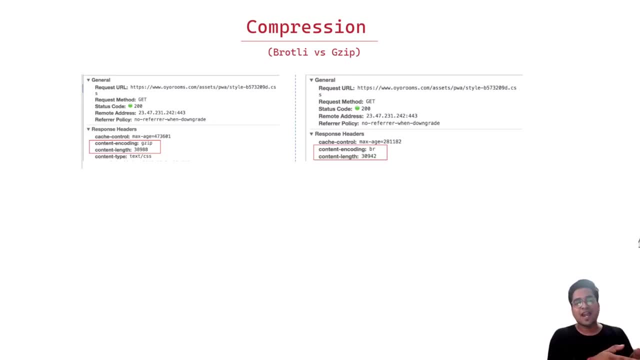 in order to decode right. so similar thing. if the browser understand the way i have encoded from the server, if browser also understand how to decode it, then our job is simple. right, we can compress it from the server and in the network layer, those compressed file which converted from the 300 kb. 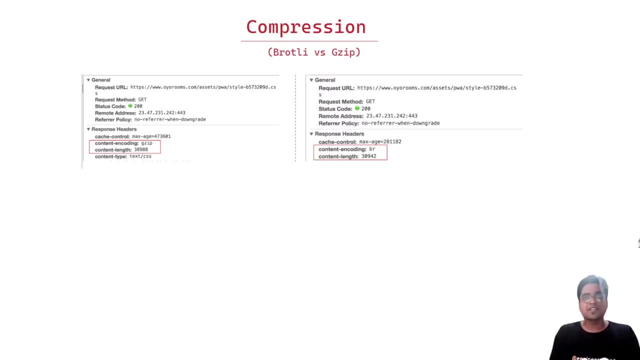 to a small- you can say 60 kb file. 60 kb is definitely a very cheaper as compared to the 300 kb, right? so there are two very popular strategies which browser also understand. one is the broadly and second is the gzip, so we can see a. 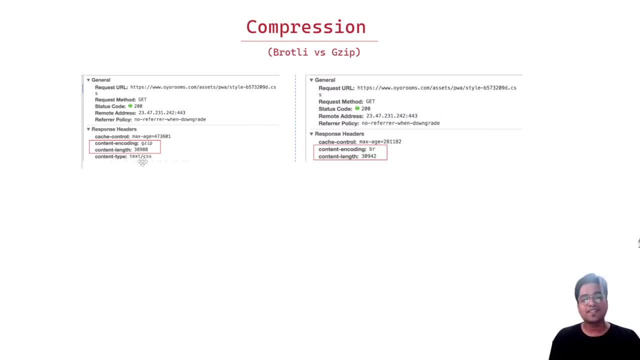 comparison, even the broadly, is far better than the gzip we can see. one of them is from the oyo, which they have uh shared the, the report and the thesis from there. we can see earlier the size was around we can say 38 kb sort of, and now you can see it's around 30 uh kb over here, right, so that's. 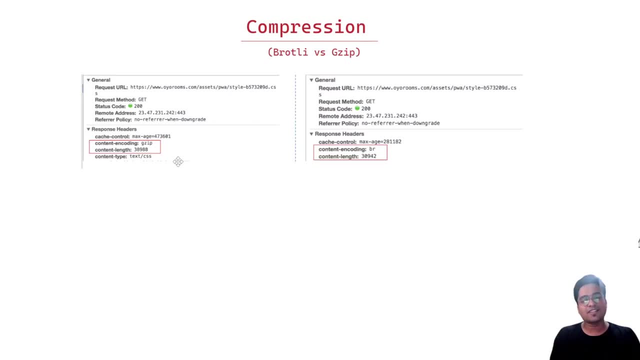 the difference we can see. uh, it has a lot of reduction in the approximately eight kb reduction, right, but it's just enabling up broadly, so that's a big deal, right. so you, you get a lot of thing. now there are still some browser which does not understand the broadly compression in that. 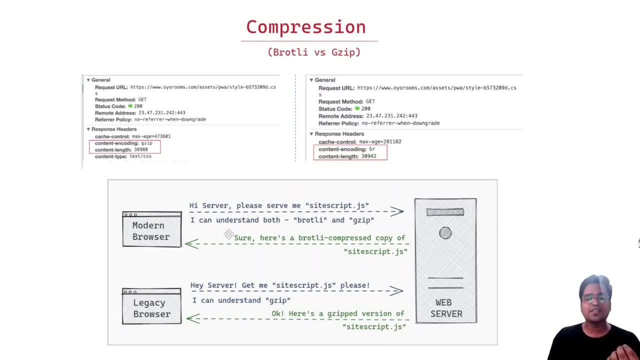 particular case how we can leverage it. we can add a strategy which says that from the browser- hi server, please serve me the any file which is maybe site scriptjs. i and i can understand both the browser and broadly and does easy right, this is your browser- says that in that particular case. 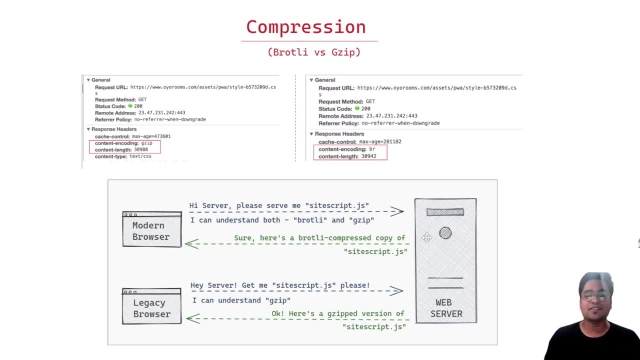 your server is going to give you uh one with the broadly comparison- right, in that particular case, you are getting a lot of benefit because the size is small. but their legacy browser, which does not understand, they will say: i just understand the z-zip. right, in that particular case, what browser is going to give? browser is going to give you the z-zipped. 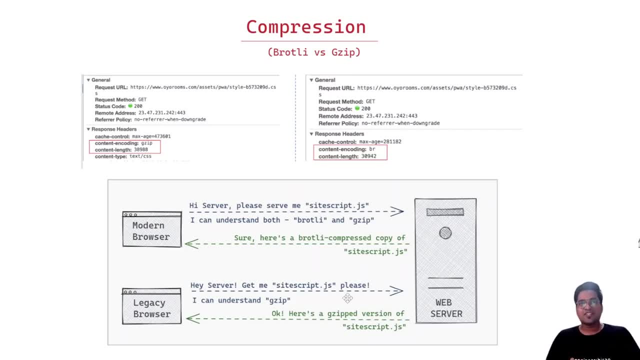 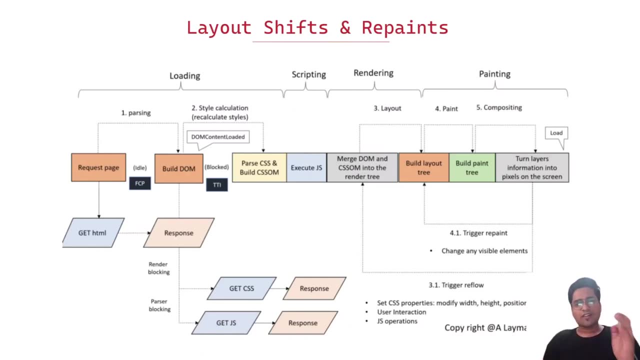 version of that. so now, in that particular case, you can leverage the broadly compression but also taking care of the legacy browser. in the starting of this video, we have talked about how javascript delay or the css delay- loading from the network- can impact the performance. right now it's time to dive into the detail: actually what is happening and why this is impacting. 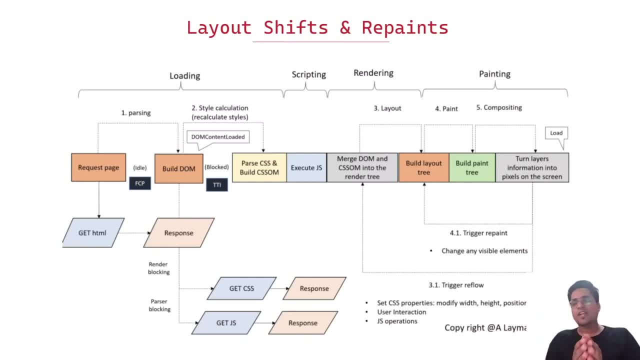 we will be going through the render cycle and we'll try to understand different cycles, different phases of this rendering cycle and what are the things that you have to take care of in order to make your web application more, more, more performant. right, so we'll be talking about. 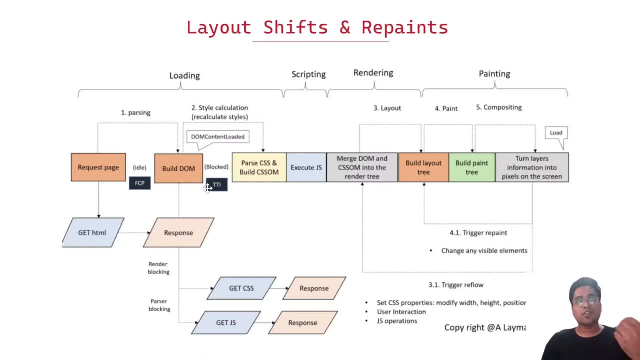 layout shift and the repaints. that happens because of certain things not taken care in a certain fashion. now let's understand the rendering cycle. so first first thing is you have to request your page. you will get a html from that html. you will get the response from your response. in a sense, if there are certain css or if there are certain js, those will be. 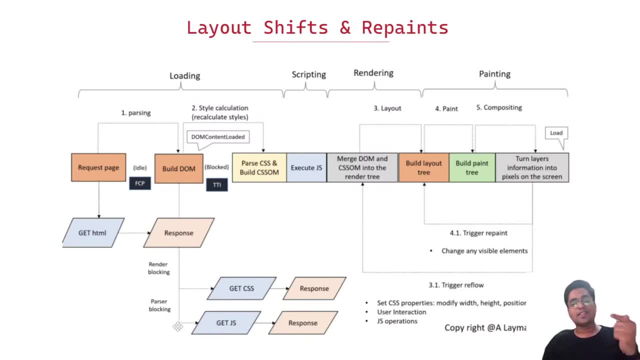 downloaded. to note, it is very important- any css or html basically which is on your head, and those are, in general, basically render blocking or parsing, blocking, right. so your render blocking basically, you see, anything is not going to render until unless your your javascript or css are basically loaded. and similarly, if your css is not loaded, it is not going to block your. 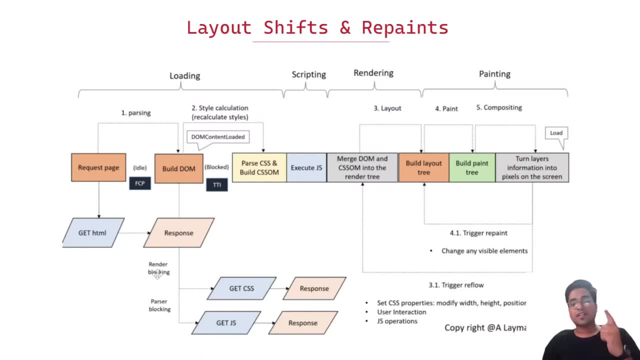 passing, but it is going to block your rendering, right? this is very important thing to note. once you have a response, your dom is created. you are aware of the dom tree, basically, which is created from that dom tree. now you have your html, you have your css, both of them get combines and there is a 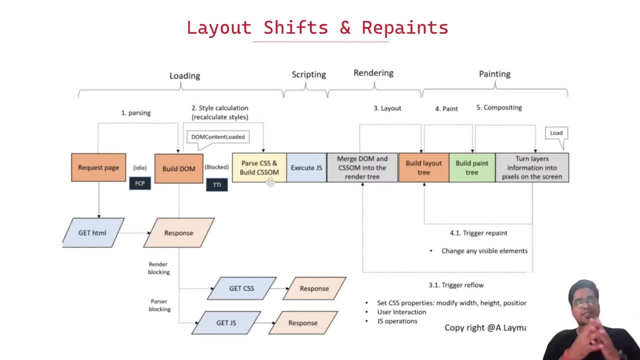 recalcate styles is done and the css om is basically created now, depending on what strategy is being used in order to load your javascript. now your javascript is basically executed over here. once a javascript is executed, you get your dom and css om merged. so now there was a dom. 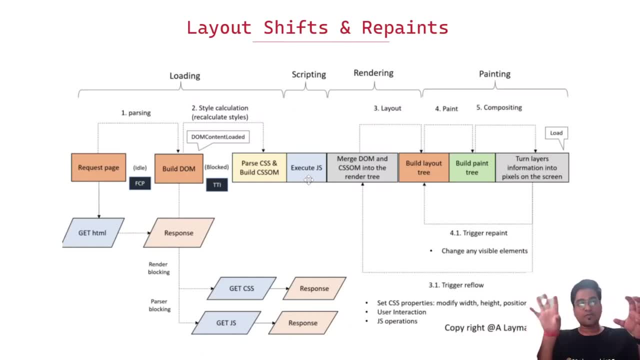 there was a css- now css om- that rules for the css was generated. both of them get merged in order to create your render tree. this is very important phase. we have to understand right. you created certain rules. with that rule, we have css om. we have dom tree, which talks about the 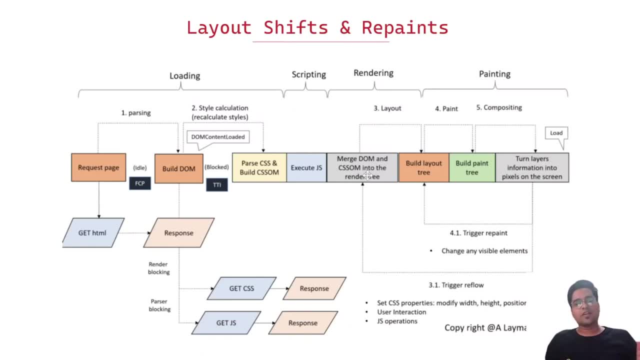 structure and different div and different layouts that you have in your dom tree and now both of them got merged in order to create a render tree. from there, the layouting is basically done. when we say layouting, layouting is just. you can consider you whenever you see a big buildings in. 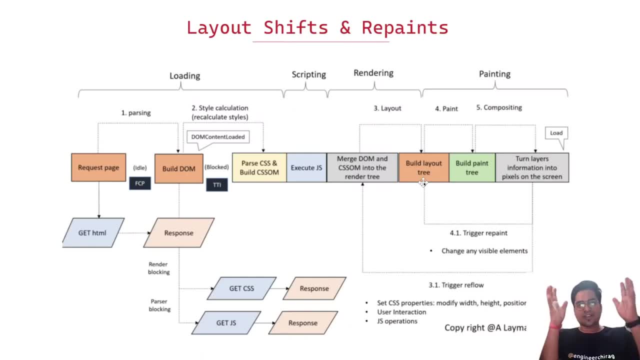 metro cities how they are basically structured. they are structured based on the pillars. first the pillar, the blocking, and everything is done, then the walls, and everything is basically structured and your interior is done right. similarly, you have a long, tall building where the pillars are basically configured or, you can say, established after that. 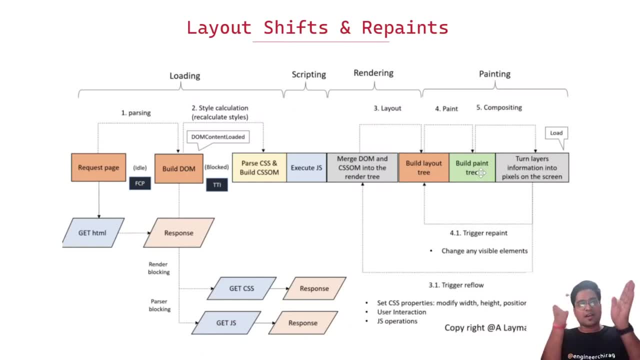 what is happening you? you basically build your different walls and then your paint basically starts. right. your painting is like you get things started furnishing in your empty house and finally, once everything is configured, you start basically putting the items at their different places, like you put your tv, you put your sofa and different, different thing in your house. right, that is. 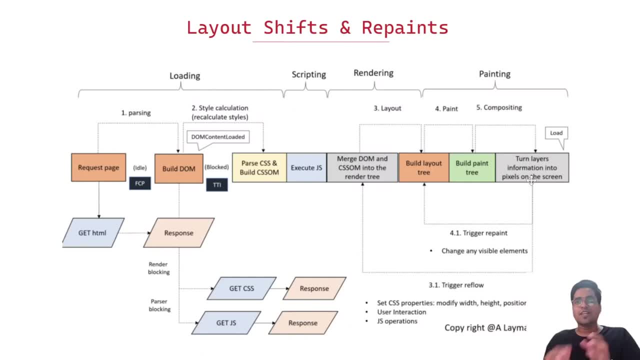 basically a pixel, perfect thing which is basically drawn on your screen. so in similar fashion, you can basically relate from a building construction to getting things basically created and segregated using your walls, and then getting it painted, and so that you have full furnished, marble tiles and, uh, whatnot- painting is done and then finally placing those things in your home. so similar thing. 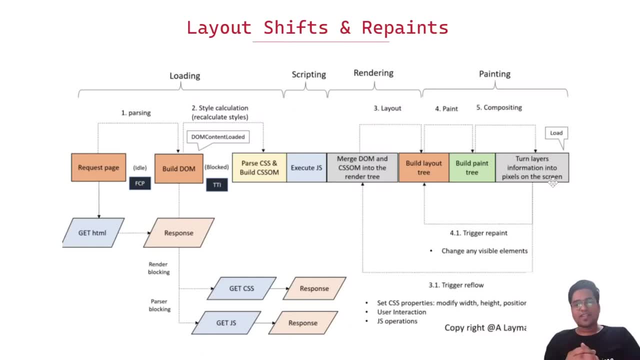 happened over here. now you have to understand with taking the same example. there are certain things that you should be aware of. right. first thing is composting. second is painting. third is layout parsing. right, these are the terminologies you should be aware of. now try to understand there. 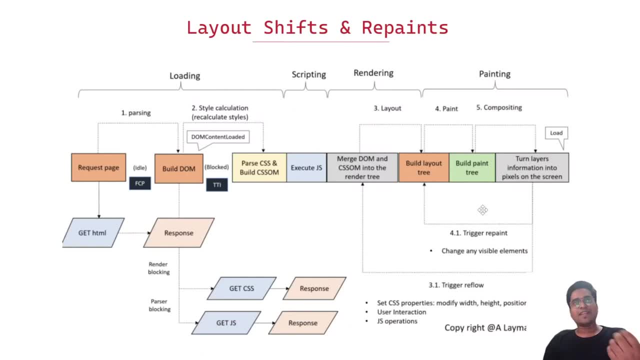 are certain scenarios which are very costly. when i say costly, consider example: once your house got built, your, your setup got built, you realized, oh dude, my kitchen is way small. i want to increase my kitchen size. what do you have to do, think of, in order to increase the size of your kitchen? 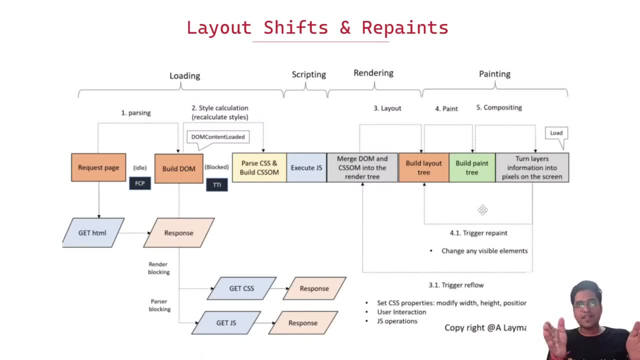 you have to shift your wall to increase the size, you have to again get the denting painting marble and sort of thing, and then again you have to, basically, in order to make your kitchen model, you have to make some major changes and in order to put the different item in your kitchen. this is: 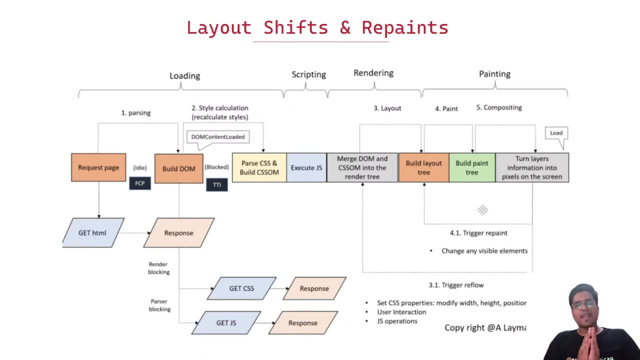 very costly. what if you have to just say, okay, everything is perfect, i just wanted to place my refrigerator from this wall to that particular wall. that is way cheaper, right? so now let's put those terminologies inside: the: the wall right. the rendering, so how, how this is basically going to happen. consider, there was a change. 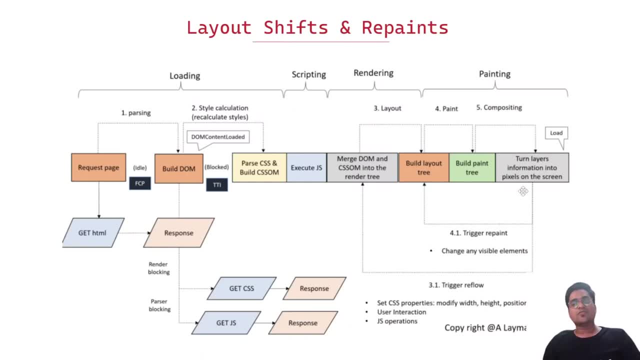 there are two type of change. basically, one is just going to trigger your repaint, which is just shifting your refrigerator from one location to the other location. it is not going to impact anything. second kind of thing: anything which is related to the dimension, anything which is related to the user interaction or the js operation, those are basically going to actually change the 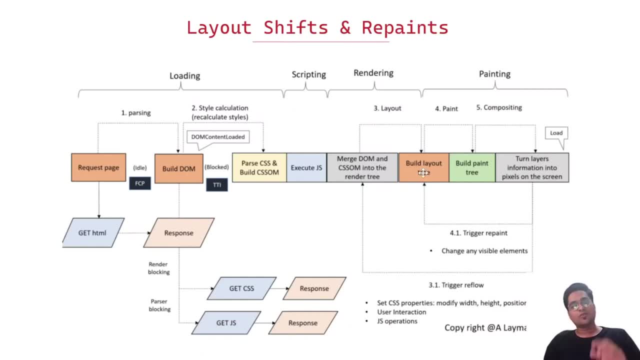 dimension of your kitchen as well. right, in that particular case, it will go through again creating a layout, again doing a painting and finally putting it into the pixel. perfect thing. now let's try to understand what are the different things, what are the different properties which can basically impact this and which can be main cause for this. let's, let's understand that we have. 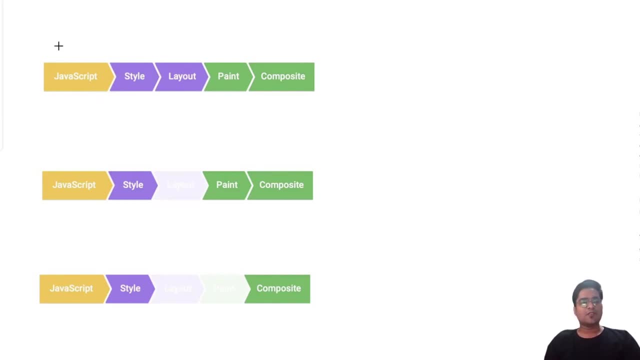 seen this, these phases right. so anything which is related to the like- downloading the javascript because of the javascript, if there is an impact in the css or the dom, basically taking care of that, anything which is basically going to impact your css home, right. then basically there is a layout, layout in a term, the similar thing. we talked about the builders. 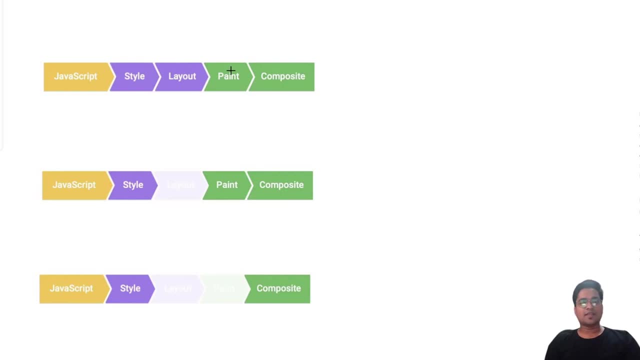 building structure which need to be created. painting is again making it full fun. uh, you can say making it denting, painting marble and whatnot. the painting done with that composting is basically- uh, this is very interesting. we talked about above, this is the final- like putting your pixel perfect and the items in your house at a different, different places. 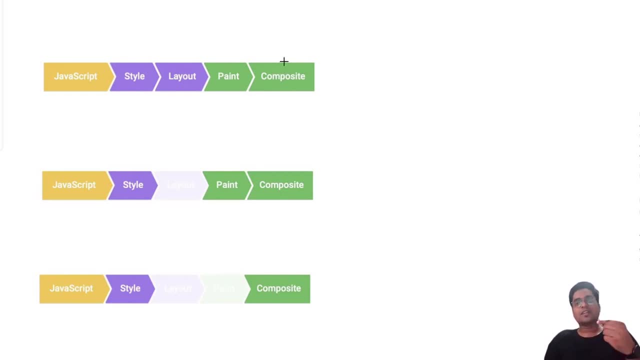 one thing which we have to also consider over here: it also do consider the different layers that we have. so in your webpage, say suppose you have a model that comes in a different layer, all together right, you hover on certain things. you see the different tooltip and different uh layout, all the dialog box model which you see. those are the different, different layers. 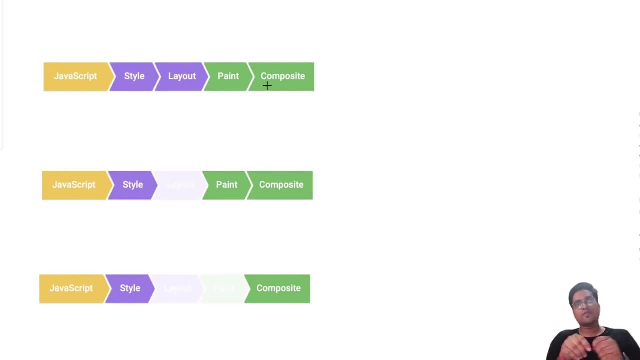 right, even you use position absolute side of thing or position fix, those are the different layer kind of thing. those are handled in this particular composting phase. now try to understand if we try to make any change in our styles using javascript or css which is going to change our dimension, what are those dimension property which can be changed? 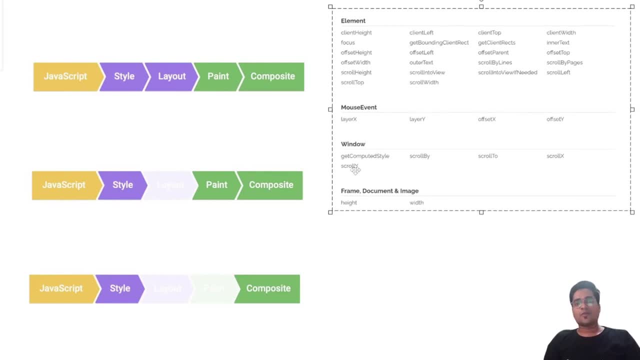 let's quickly peep into that. these are the properties which can basically trigger all of these cycle. either you are changing from here or here, it doesn't matter, either you are using javascript or the stylings. basically, what are the phases it has to go? it has to basically go through. 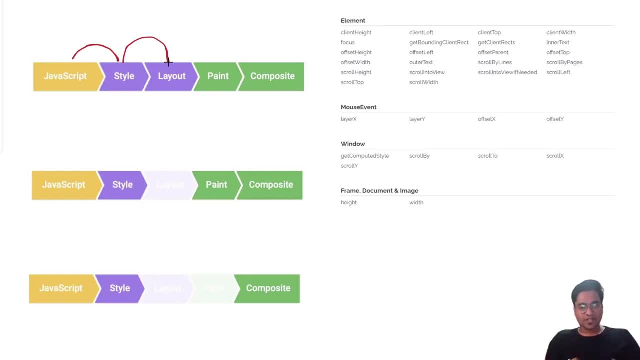 layouting, which is basically creating your building structure. second is painting, getting stains and basically getting the marble, everything perfect. then finally, composting, putting things in a different layer, making it final, giving it a final touch by placing the different, different items right. all of these has to be taken care of. this is very, very costly. what are these property? 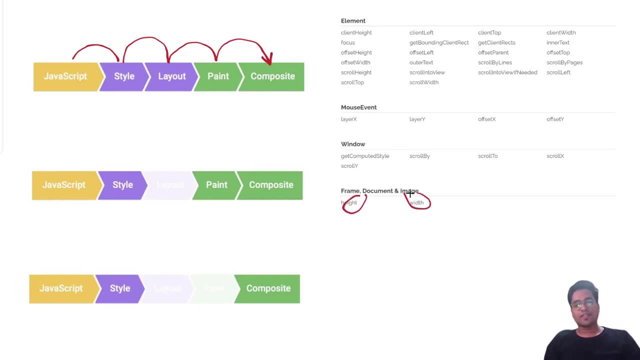 anything which is related to your height, which is related to your width, anything which is related to the dimension. so if, even if you're trying to read certain properties which are related to the dimension, you can see which is related to the offset or client height. so all of these are going. 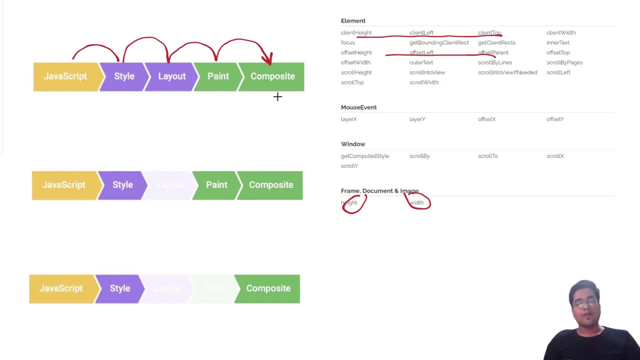 to trigger all of these phases, which is very, very costly. why these are very costly? because browser have to give the latest values of these dimension whenever you are looking for. even that is read, not right, right. this is very, very important to note down- anything which is related to the offset. 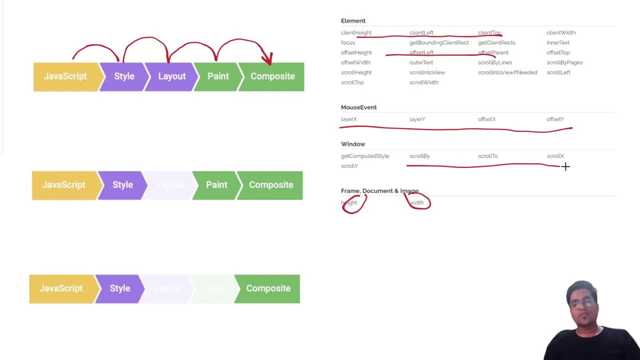 again, those are going to be very costly. anything which is actually going to make your scroll to top, or we might have used scroll x or y sort of thing- all of these are very costly and these are going to basically trigger all of these phases. now, what, what? 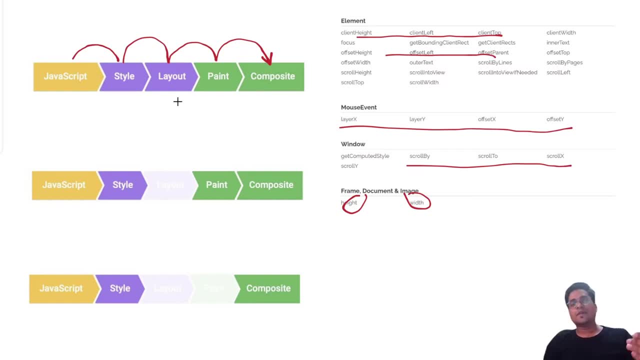 better we can do? what are the properties which can actually save something in this particular cycle or these phases? so the other set of properties which are very important and cool to understand, anything which is related to your background color or even your text color, right, anything which is related to shadows. 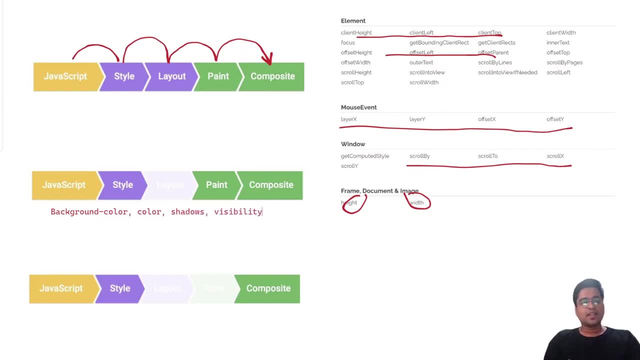 right, anything which is related to visibility. these are, and they are a couple of more. these are basically going to do a very, very important thing which is related to your background color, and i always like to say that that's going to hurt up your background. that's going to be. 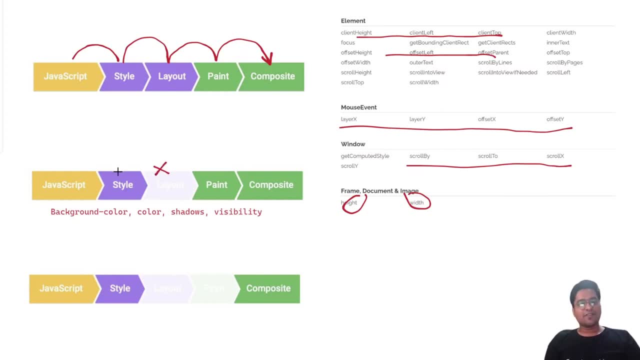 really, really bad. but with the xbox play 4 you can do a very good job for you, which is it won't do a layout shift in this particular phase. it will basically definitely if there is anything from the javascript or style that is going to be there, but it is directly going to jump into the paint. 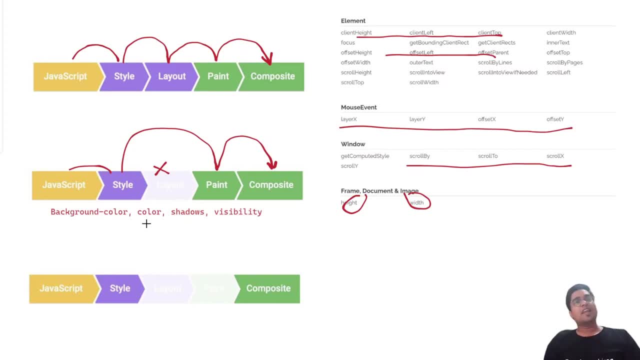 and it is going to directly jump into your composting. it is not going to do anything which is related to the layout shift and which is very, very important thing if you can basically avoid. this is very time consuming and this takes a lot of- uh, you can say- computation for the browser in order to basically draw the layout shift, and so you have to do a good job of that. 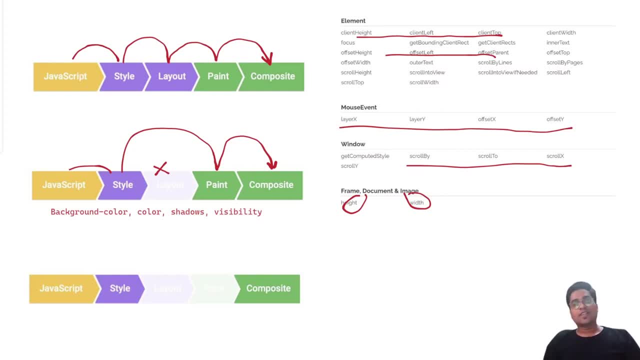 the final pixels on your web page. now there are other cool things which you can do. you can even avoid your paint. you can directly jump into the composting uh, compost, uh step. how you can do that? there are two properties which helps to do that. one is transform and second is the playing with. 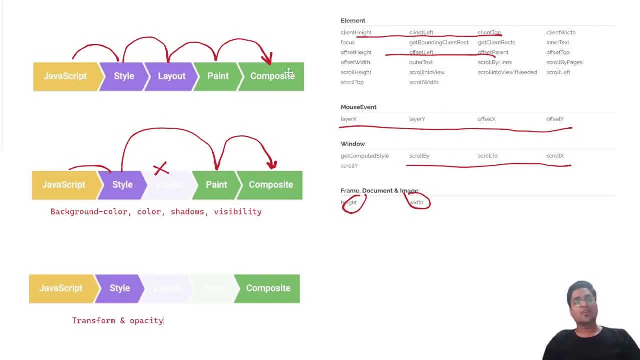 the opacity. these are the two things which is even going to remove two different phases and important phases, which is your layout and your paint. you can directly, or definitely any from any place we are doing. you can directly jump into the composting over here and this is very good. so 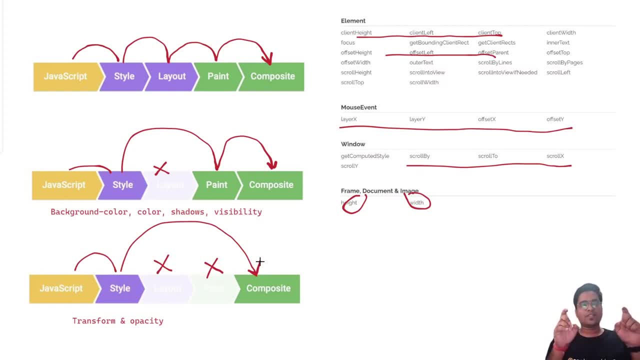 that's why you might have seen anyone who wanted to play with some sort of animation where you wanted to change the dimension of your- uh, you can say dialogue- or you wanted to change, or you wanted to play some animation placing a component or a visit at one place and you wanted to do a transition. 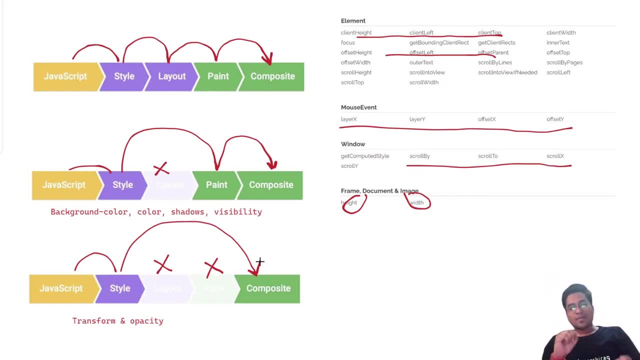 to a different place. in that particular case, it is recommended not to play with the dimension within height of this. instead of you can basically do a transitions, which are going to help you out right, or do a opacity, play with the opacity. these are the two things which is going to help you, even the composting. now the question comes even: why these things? 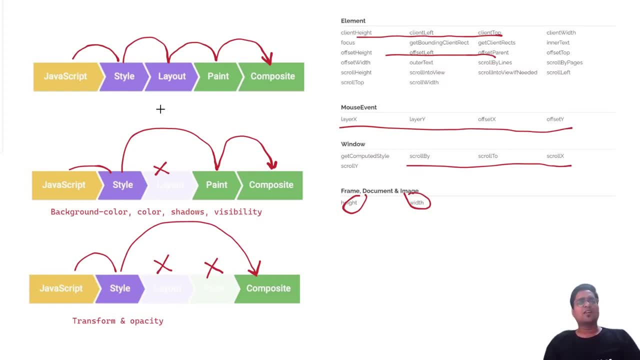 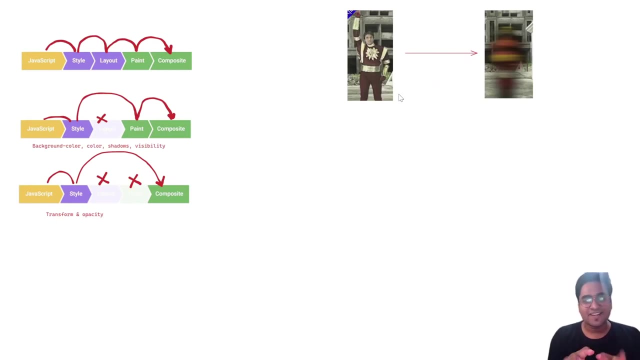 actually matters, like even if we ask our browser dude do some extra work, then what's the harm for a browser in order to do an extra work, which is layouting, what it costs? let's understand what it costs for the browser in order to do that and why this is important. let's understand very interesting. 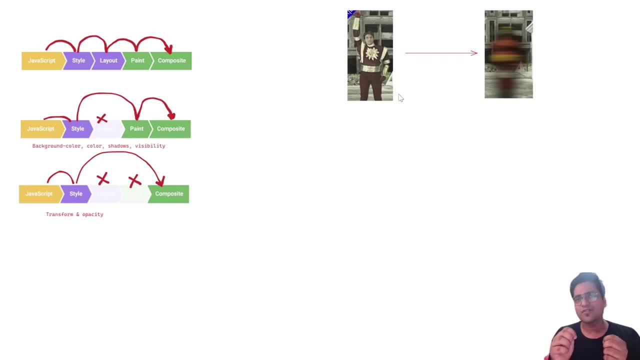 thing about how this is related to- you can say- different devices- and how it is even related to what we just talked about. right, try to consider, when we are scrolling our web page, what we wanted to see. we wanted to. we even we are scrolling fast. we wanted to see some content on that. we don't want. 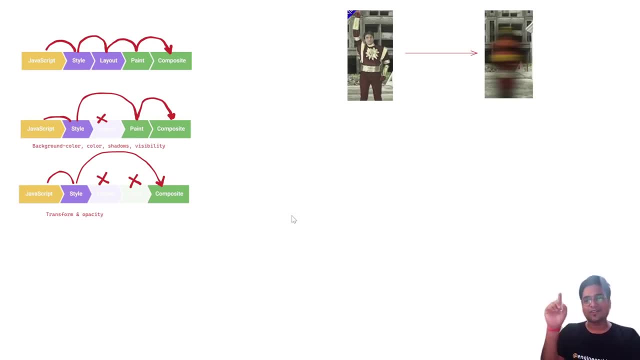 to make it Shaktimaan, right what it meant by. we scrolled and we see something is happening weird, but we are not able to see anything right. we don't want to make Shaktimaan- people who are aware of it don't want to make it flash like we don't know what happened in behind. we are not able to see. 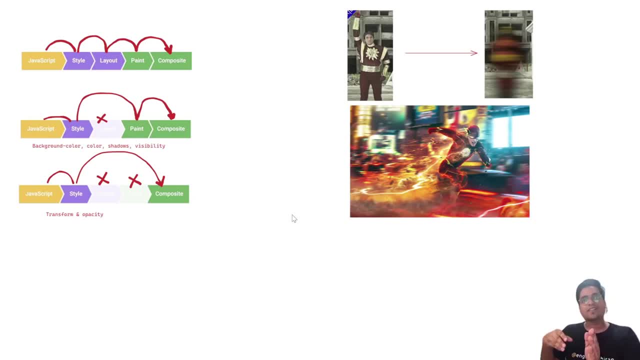 anything in between when you are scrolling, and we don't need that experience at all when we are scrolling or doing some activity on your web page, right. so for that there is very interesting thing that we have to understand which is a frequency or which is a, you can say, device refresh rate. so 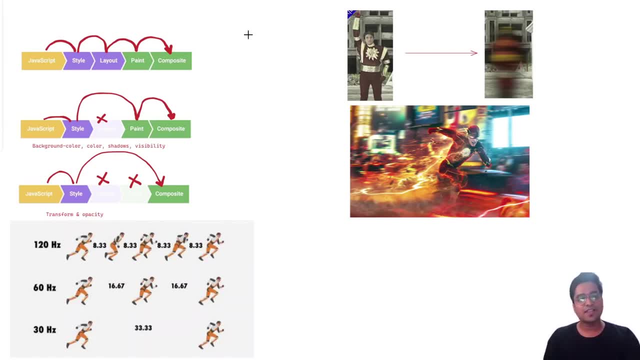 most of the browser, most of the devices that we have has a frequency of, has a frequency of 160- you can say 60 Hertz over here, which is equivalent to what it meant by. it is going to basically render or refresh your screen 60 times in a second. okay, what it meant by 60 times in a second. then how many frames do you see? 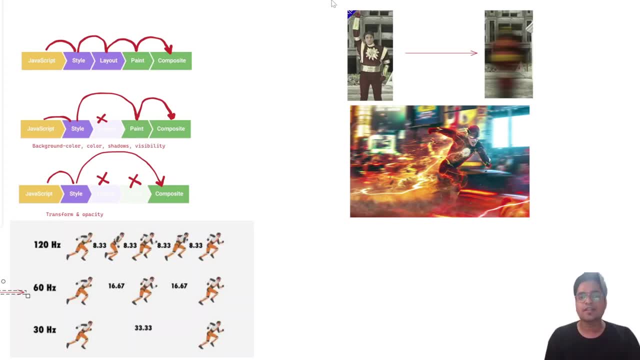 in a second. any guesses? I small map, let's do that- how many frames we are going to see in that particular case, what we are saying in one second, how many, how many frames basically we need or how we are going to refresh? it is going to refresh 60 times, so this is equivalent to your 16.67 these. 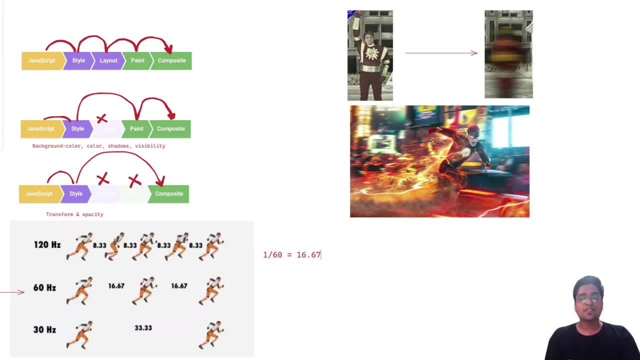 number of the frames. basically, we have to show within that one second so you can understand. a browser have got a job in order to complete whatever we talked about: your styling, layouting, paint and your composite- whatever activity are doing within this particular interval. don't you think this is crazy? this is way crazy for this. it is going to be. 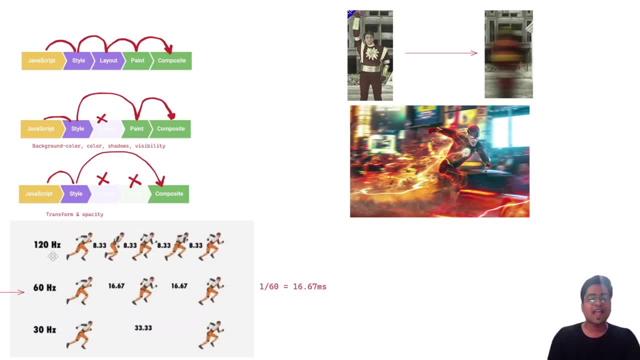 like 16.67, but there are a few devices which actually works on 160 Hertz where you wanted to show better experience when you are playing the game. you wanted to have a very refined. you don't want those delays between the frames and you want it to be very real-time, active on that right. 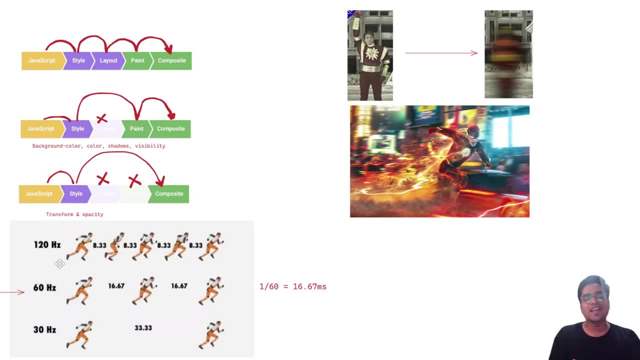 so in those particular case now, device are having 120 Hertz as well, which is these many frames that need to be rendered in a second right? these many times it need to be rendered? how many frames is like? 8.33 ms is required in order to. 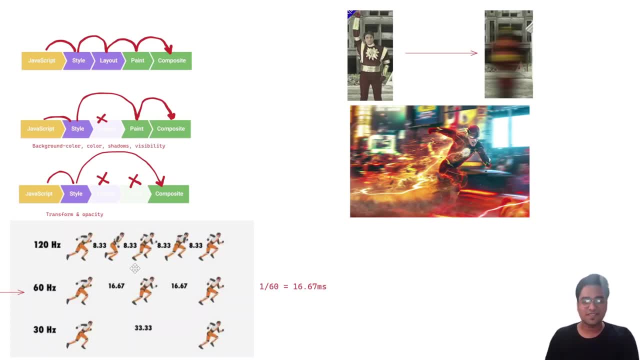 uh, basically render a single frame. now this is, this is even complex and tougher. now this is very tedious if, if we have to basically what? so? so understand, even if we are not able to do in 16 or 16 ms actually, which is not a 16 ms, I will tell you very frankly, because 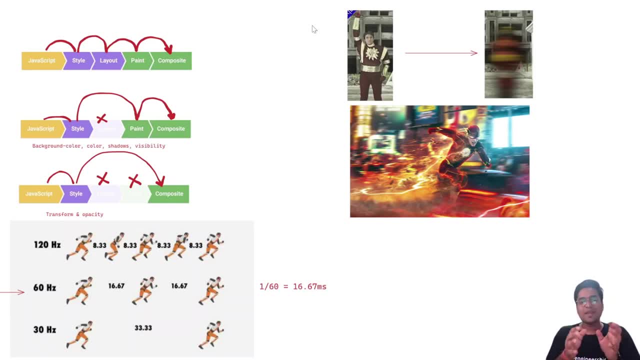 their browser have to do a lot of other things in order to basically make the render, the one frame right. so, behind the scene, actually, if you see, you actually got 10 ms in order to render a single frame so that you don't give a Shaktimaan experience to your users in that particular case. 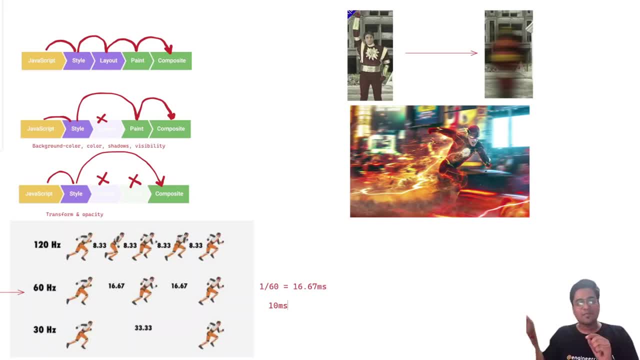 you have to make sure whatever activity is being done can be completed by in within 10 ms by the browser, so that there is no glitch and what it meant by you might have seen. you are actually doing something and your browser hangs. you are scrolling, your browser hang, you are not able to. 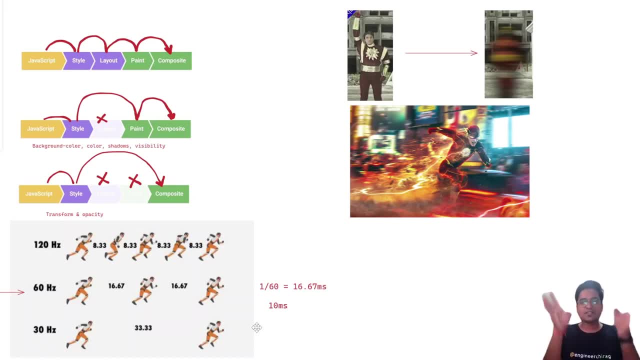 see certain things when you're doing a very, very frequent scrolls and your screen gets blank, right. these things happens basically when your browser is not able to the expected stuff within your 16 Ms, or you can actually say which is 10 Ms, right. 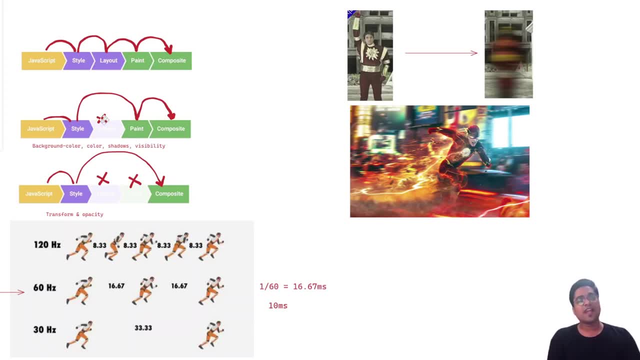 So you have to make sure these things which we talked about- layout shifting and the repainting- why this is important- If you give browser to do a less job, then browser can make sure these things happen within our given interval, which is within our required Ms, which is there right? 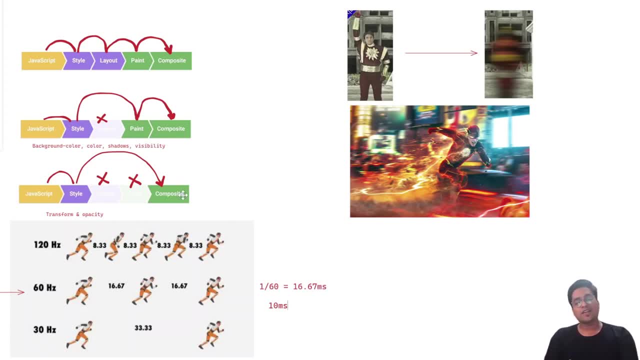 Which is 16 Ms for the browser. Now there are a couple of more interesting thing which we have to understand. Say suppose we are loading multiple fonts. in those particular case, can we club those font in order to render them in one time, load them in one time and apply to in the? 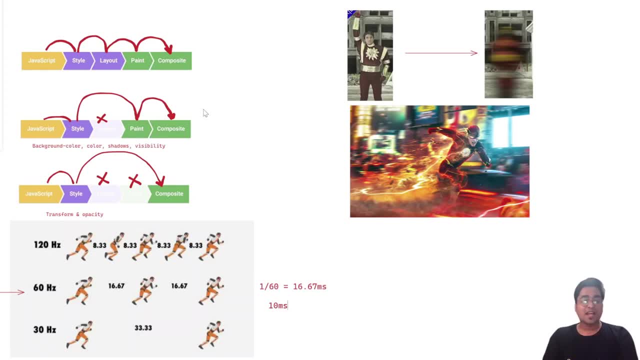 one time altogether right? Can we set the height and the width of the images when actually it is going to the render for the first time? instead of, it is deciding the height and width of the images when it is actually rendering it, right? 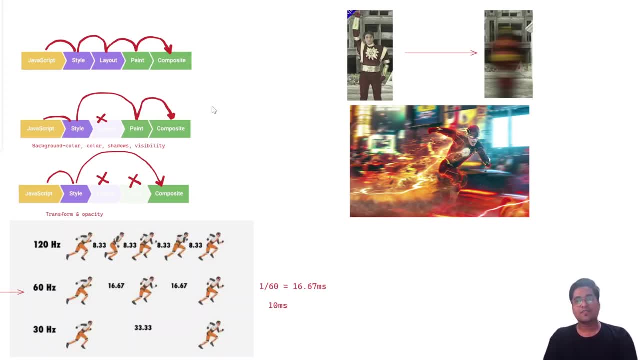 Can we basically use the SVG placeholder for the images and the videos to reserve the display box So that it does not basically Create a layout shift when actually actual images are basically rendered? So there are so many interesting things that you have to think about in order to avoid. 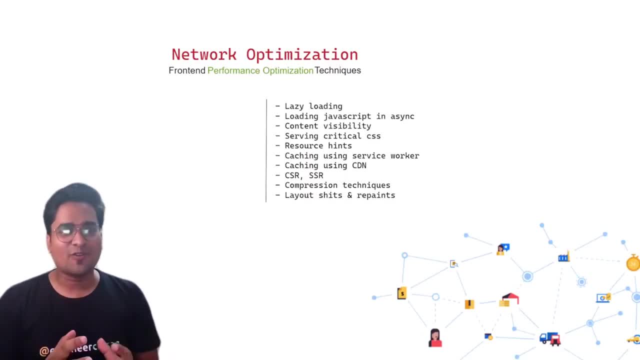 these things- Whoa. this was a powerful pack with the network optimization and there are so many things that we wanted to cover in the optimization in the upcoming episode. This is just a start. We are going to cover the asset optimization, We are going to cover the build optimization and the performance related stuff. 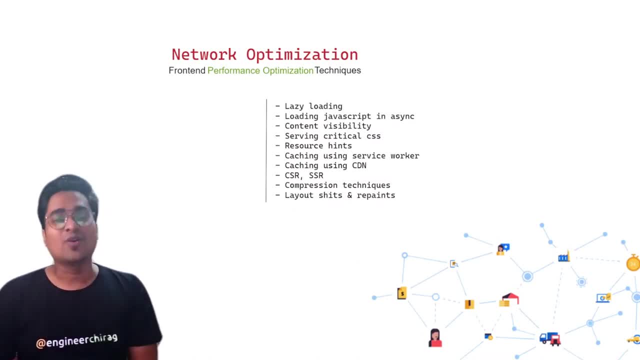 How to monitor. a lot more is coming in the upcoming episode, So Keep watching. and with that just wanted to recap what we have basically learned over here. We talked about the lazy loading. We have seen the tricks related to how you can load your JavaScript in a async fashion.